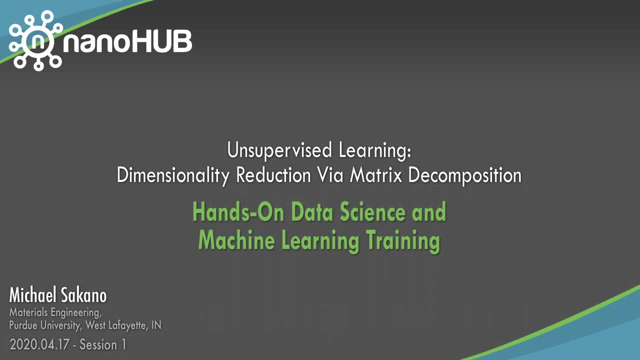 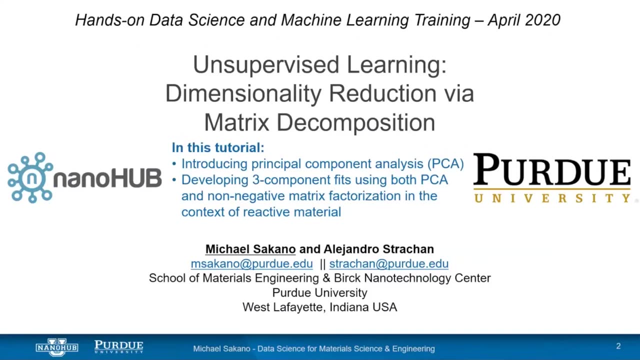 Thank you everyone for being here. I'd like to go over a brief overview of what we're going to cover today, which is to address unsupervised learning algorithms in the context of dimensionality reduction. Namely, we're going to review two techniques principal. 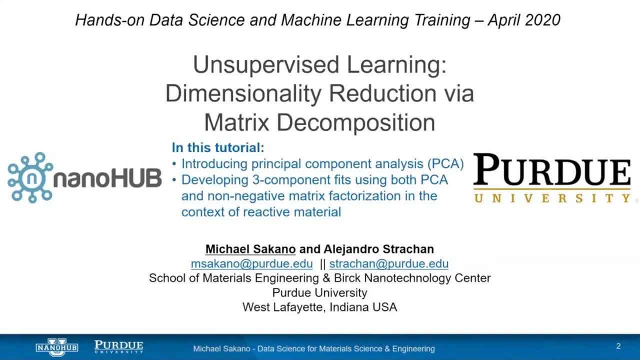 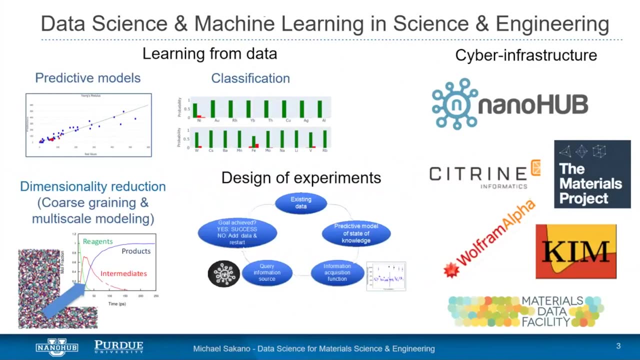 component analysis and non-negative matrix factorization, And we're going to put both of these in a specific example, which is to explore the decomposition of reactive materials. So if you're a veteran of the series, you'll know that we've been able to go through various 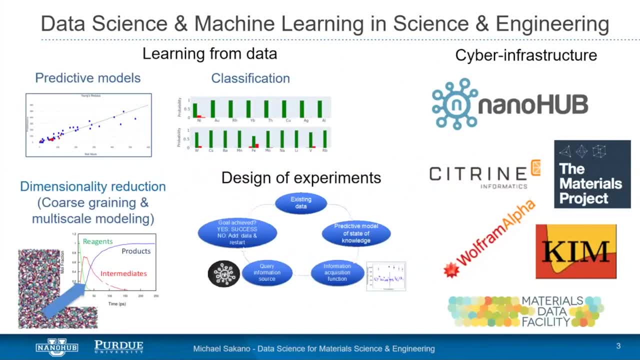 different modules that have explored where you looked at learning from data, And this can come in the form of a cyber infrastructure and data repositories. In previous sessions, we've developed predictive models and computed classifications For materials and, specifically for this session, we're going to look at dimensionality reduction. 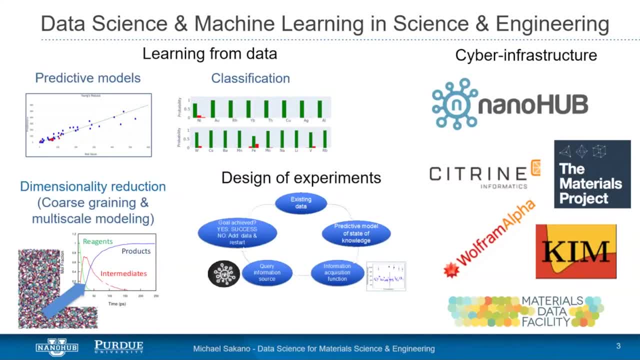 where we're going to have an end dimensional space our data exists in And we're going to try to see if we can extract out certain features that can still explain the vast majority of the data, But this reduction algorithm will allow us to take our data further to. 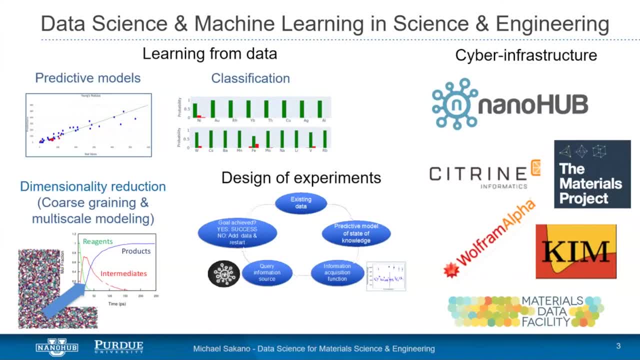 do more post processing than to have to consider all the data that we've captured either in experiments or in simulation. This is to help guide our design of experiments to ensure the highest probability that our next experiment will be successful. As I stated, this session will specifically focus on dimensionality reduction. But if 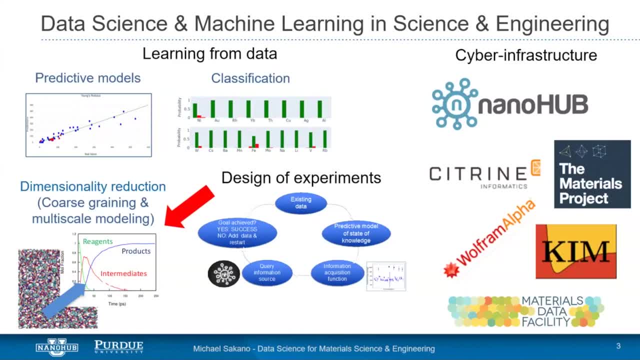 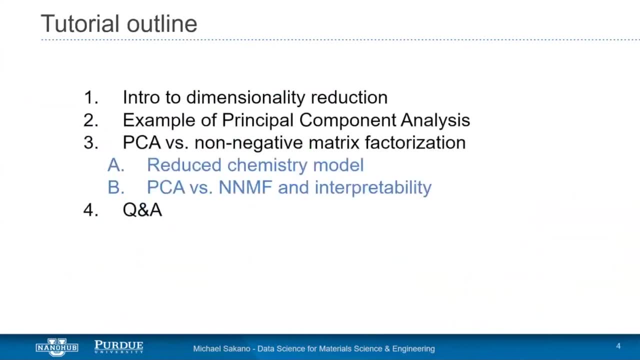 you're interested in any of the other labels here, they will be posted on the website shortly. So, as I stated, we're going to go over dimensionality reduction algorithms, mainly principal component analysis and non-negative matrix factorization, And particularly we're going to look at the 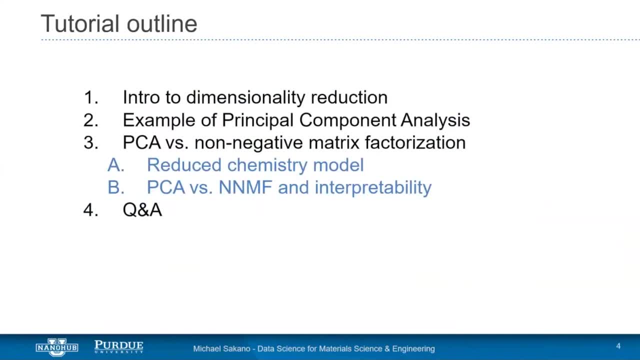 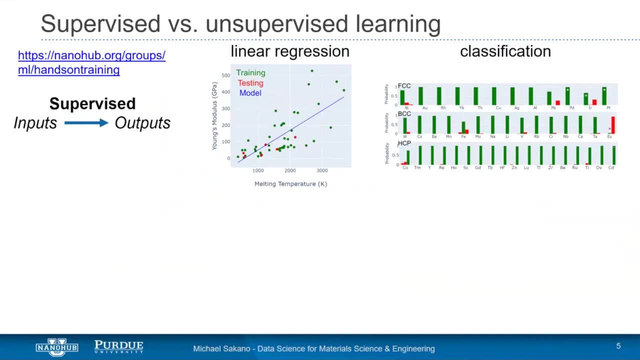 distribution of data And we're going to put in the context of a chemistry example. So I like to start out by breaking apart machine learning into two general categories: that being supervised and unsupervised learning. In the earlier sessions we looked at supervised 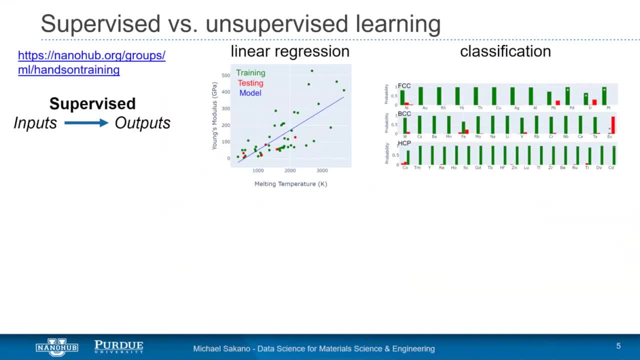 learning, where you take inputs, pass it through a model and that provides you with some sort of outputs to explain what's happening. For example, we covered linear regression, where we take in a melting temperature and try to predict Young's model. 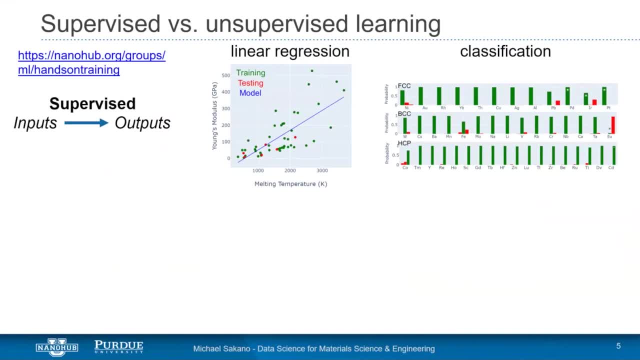 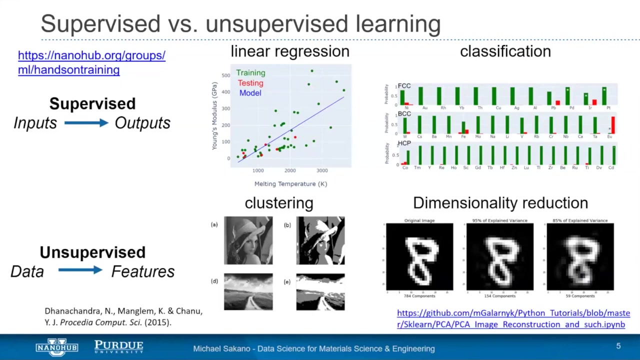 And then we covered classification, where we read into various features such as ionic radius conductivity, Young's modulus, and we tried to categorize them based on their crystal structure. What we're going to focus here on is the second branch, which is unsupervised learning, where 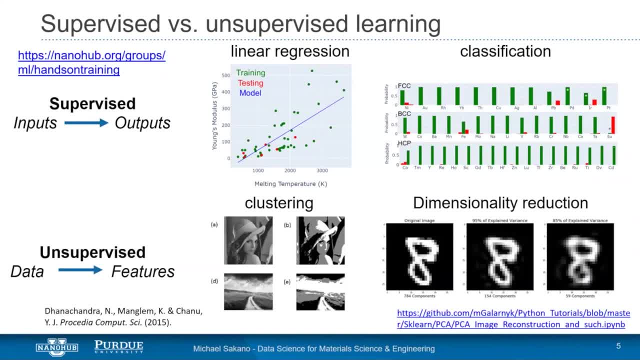 in this case, we're taking in a wealth of data that we've captured either through experiments or simulation, And we're going to try to abstract out certain features that explain the majority of what's happening in our data. This can come in the form of either clustering or dimensionality reduction, as two broad categories. 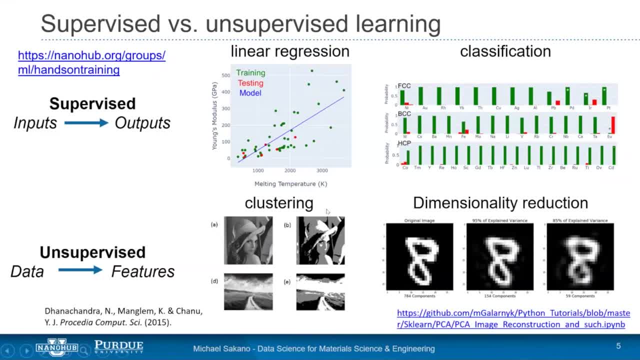 In clustering. what you can see here in this example is that we have certain features that we can extract out in our face, in this image of a person, such as the eyes, the hair, the hats, or the sky and the roads, And it's able to categorize. 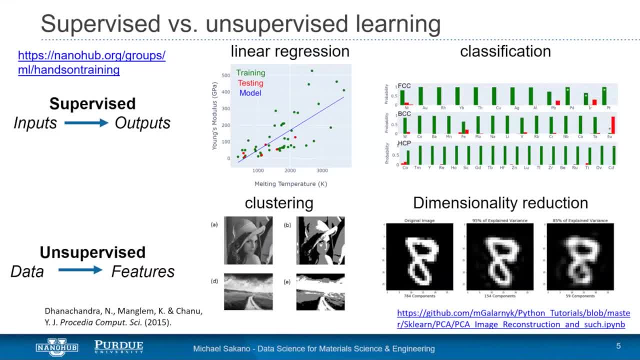 We can categorize that by doing a cluster algorithm shown here as a K-means clustering technique. What we're going to focus on in this session is dimensionality reduction. We can see in our base example of the number eight: we have an n-dimensional space certain. 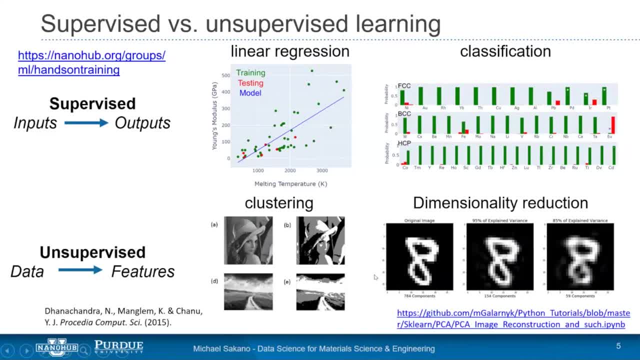 number of components. that explains how we can draw the number eight or how we can define it in our data. What we want to do is reduce the dimensions to something lower and still retain the overall outline of our data. We want to see the dimensionality of our original image, this being number eight. 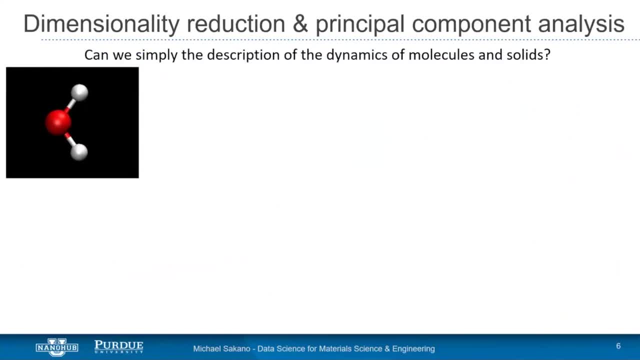 So I like to start out by explaining dimensionality reduction and try to compare it with the algorithm that principal clone analysis actually does. So what we want to do here is we're showing a simple molecule composed of three atoms. We're going to try to understand if we can actually describe the motion of these atoms. 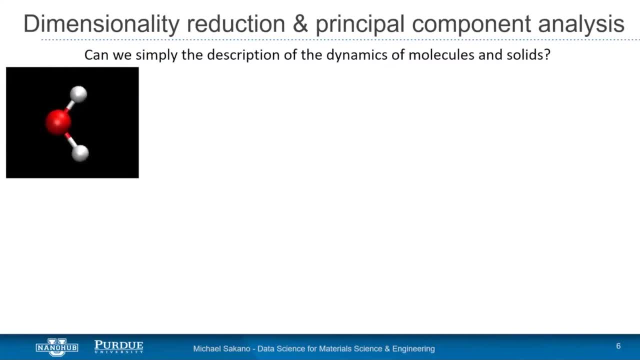 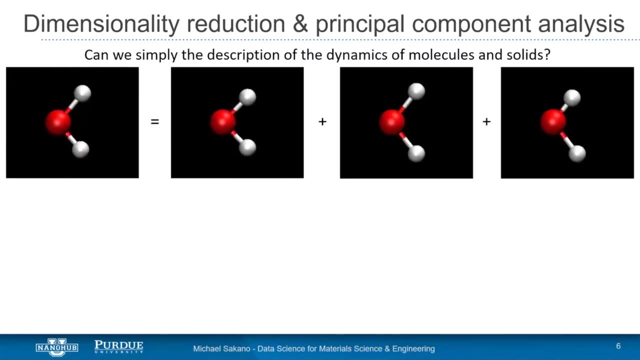 in the system over time And what we can do is we can break apart And we're going to try to understand if we can actually describe the motion of these atoms in the system over time, So we can start this complex motion into a linear combination of independent motions. 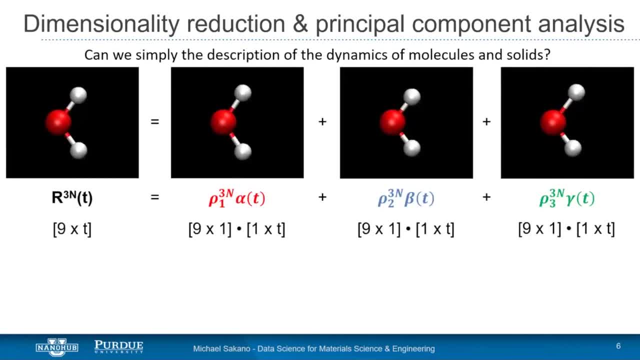 And what you can see is that for n number of atoms, this being a three dimensional space, we have a nine by time matrix for our complex motion of the molecule, And this can be broken down again into a linear combination of three independent, uncorrelated. 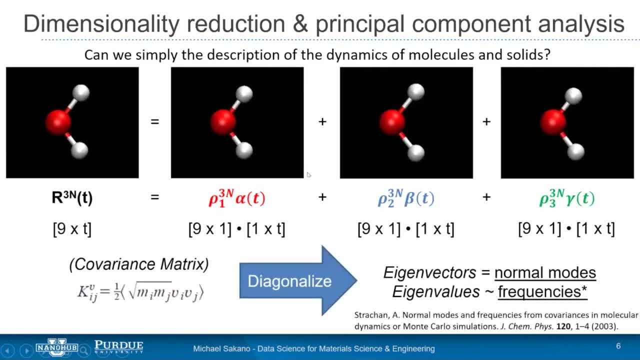 motions. In order to solve this problem, we need to actually compute the covariance matrix And, as the name suggests, what this matrix contains is the correlation between any of the features inputted at the specific index. So the correlation between feature one with feature two will go into the index of one. 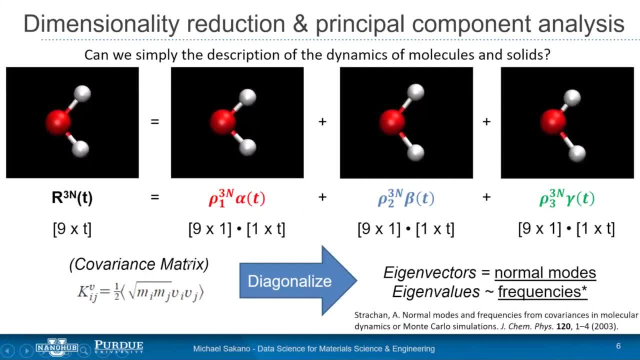 two, so on and so forth. In order to solve this problem, as it is a linear algebra problem, we want to diagonalize the matrix. And what diagonalizing the matrix will do is we essentially want to eliminate the off-diagonal terms of our n by n matrix, covariance matrix. 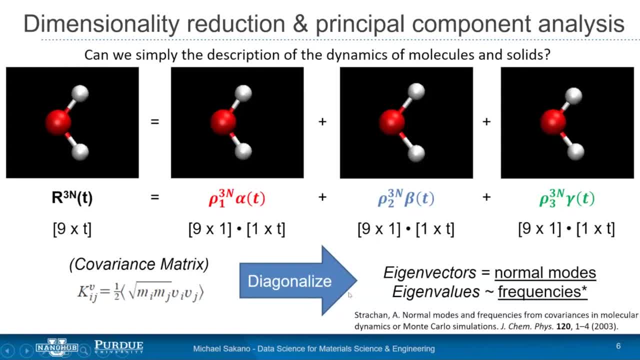 And in doing so we ensure that we decouple or de-correlate the features from one another, thereby maintaining orthogonality or making sure that the motions are independent from one another. In solving this eigenvalue problem, we'll get both eigenvectors and eigenvalues. 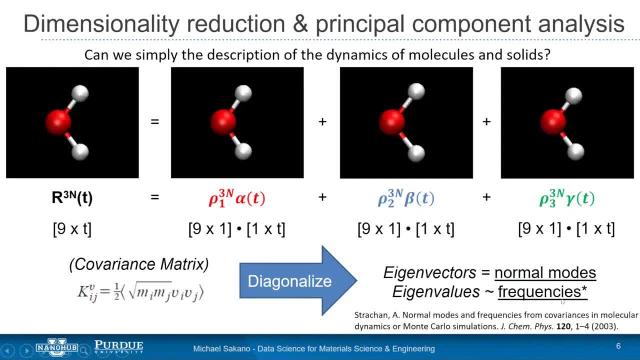 And if anyone from science or chemistry or physics or even computer science will know, that this is akin to normal modes analysis, where our eigenvectors will determine the normal modes or the correlated motions of the specific molecule broken down independently, and the eigenvalues are correlated to the frequencies that exist. 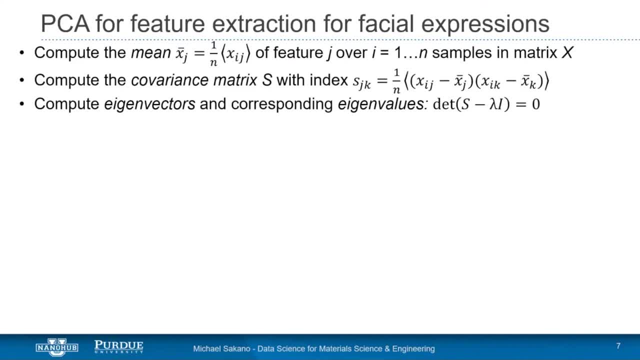 Now, as that toy example, I'd like to move on to A feature extraction using PCA and determining facial expressions. So to review again the mathematics behind how PCA works, first we need to compute the mean Using the means. we then need to calculate the covariance matrix defined here. 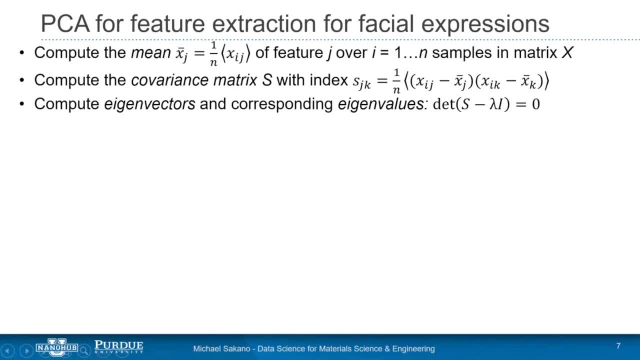 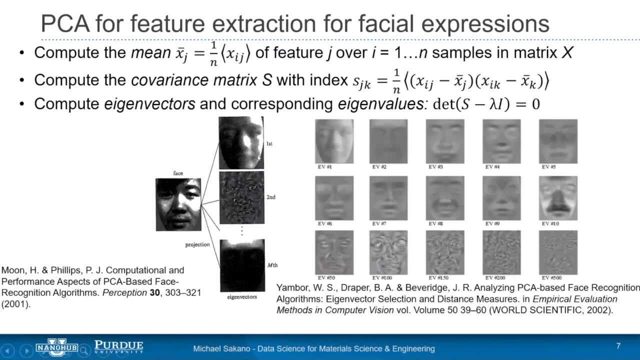 And then we need to solve the eigenvalue problem, And in an example of facial recognition you can see that when we compute our eigenvectors we get a certain amount of the, The original image described by each of the features here going from the first eigenvector. 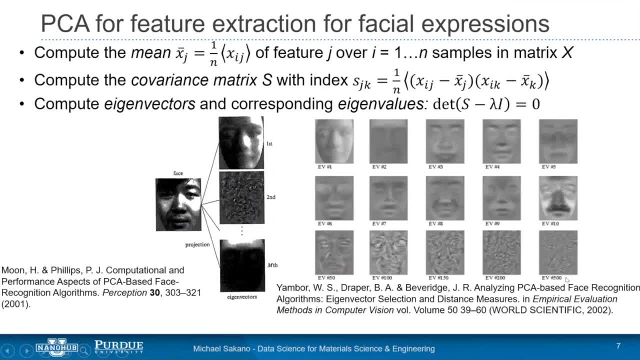 or, in this example, going from the first to 500th eigenvector And the way it's categorized, is that the first eigenvector will describe the most information based on the original image. What I want you to take away from here is that eigenvectors will encode features to: 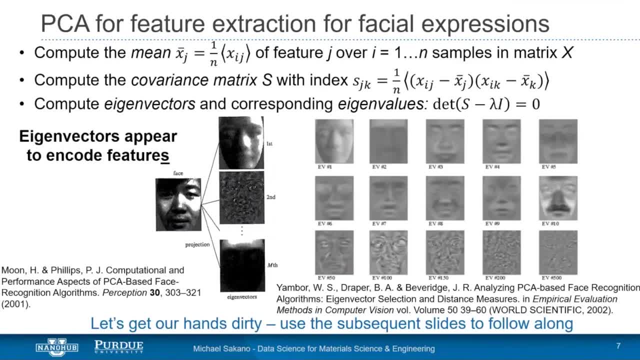 the eigenvectors of our PCA analysis will actually relate to Features of the original image, in this case noses, eyes, mouths. as they, you do a linear combination to sum them up to recover the original image, which is the face. So let's get started with our first Jupyter notebook. 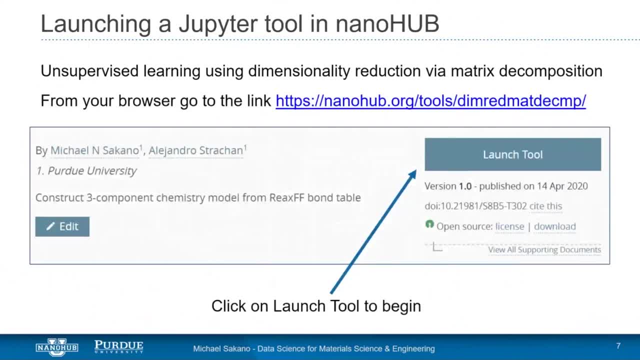 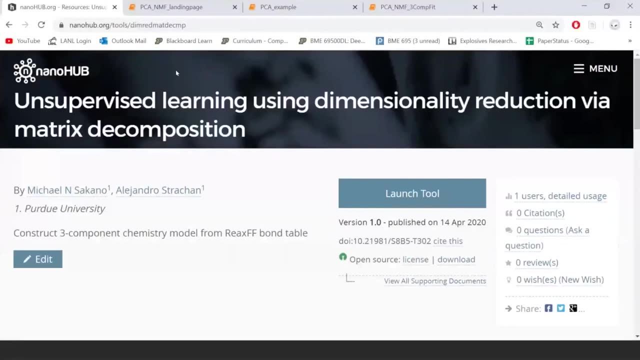 So I would like you all to do. hopefully you have a nano hub account. You can please follow me and go to this link here: nano hub dot org. slash tools- slash dim- red matte decomposition. I will jump over there. So if you open up your web browser and go to that link, you should pull up this tool. 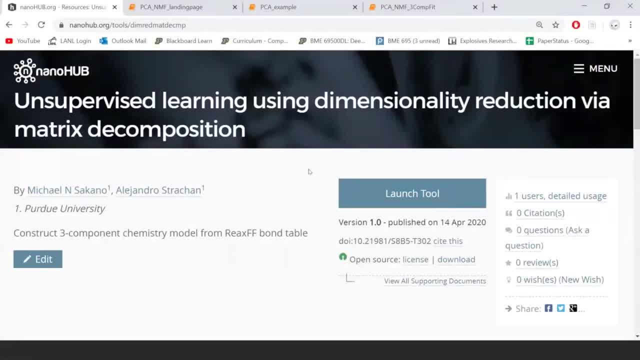 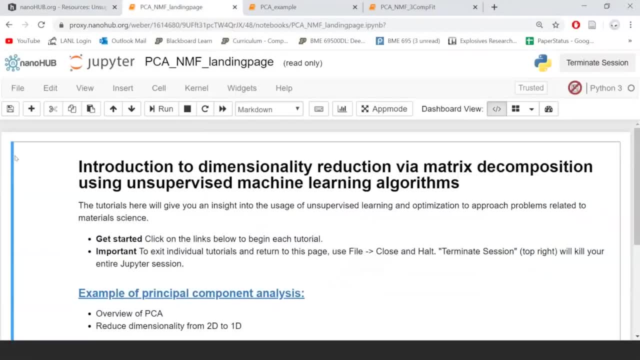 here And we're going to watch the tool, and doing so should take you to the landing page, So I'll wait a couple of seconds for everyone to catch up. All right, So if you follow along and we're able to make it a landing page, we're going to first look. 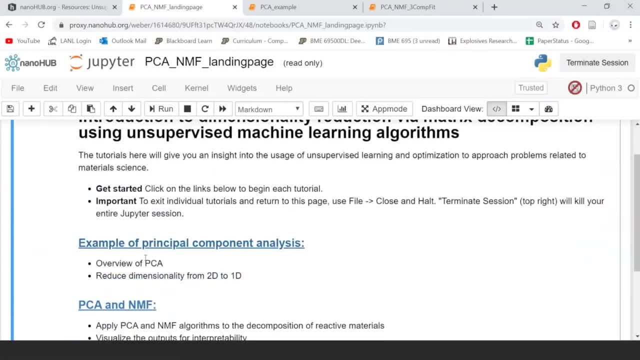 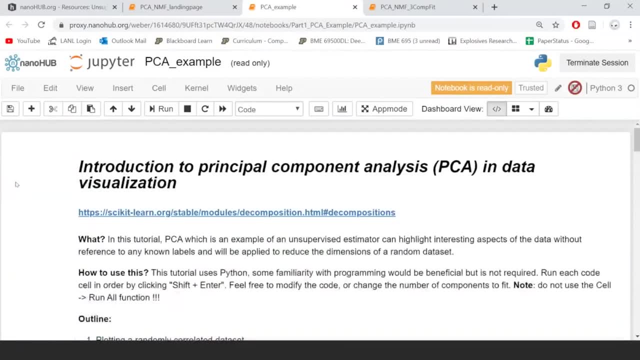 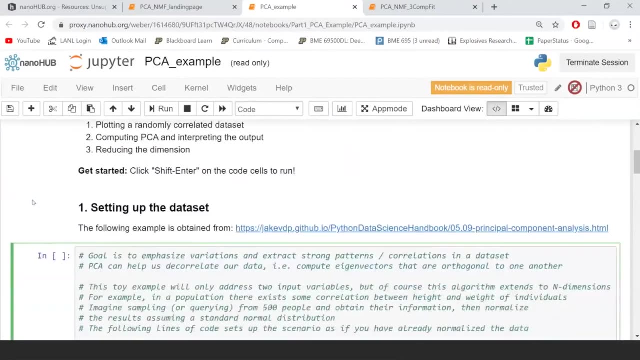 at this example Very first, Jupyter notebook, which is an example of PCA. So clicking on that will take you to this browser here and it's going to take you through an example of doing PCA in terms of visualization. So I like to just qualify that I've added some comments to help guide this example in. 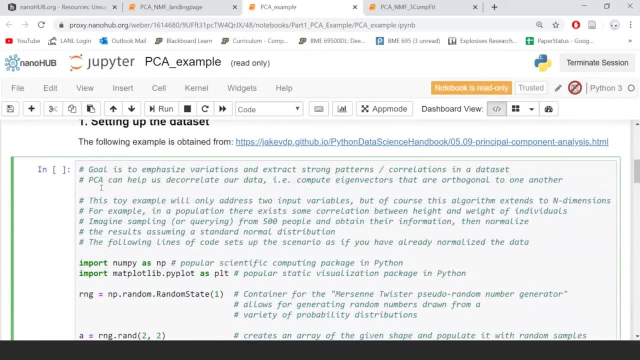 more detail. So you're probably going to see more comments here than the actual tool, but hopefully it'll make sense if you're following along in this recording. So what we're going to try to do in this example is we're going to try to understand how PCA 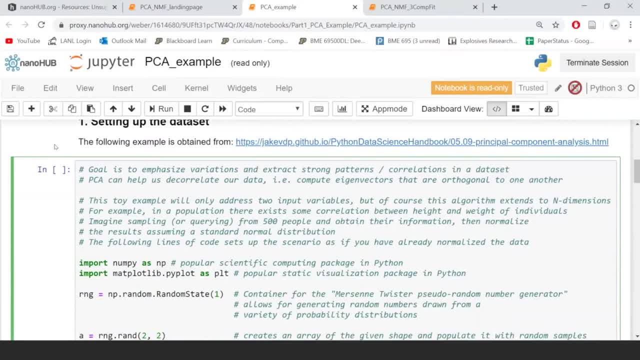 can extract out correlations in our data set. as I described previously, What we want to be able to do is use PCA to then de-correlate our data and to show that the eigenvectors that we obtain from our data are actually orthogonal to one another, and 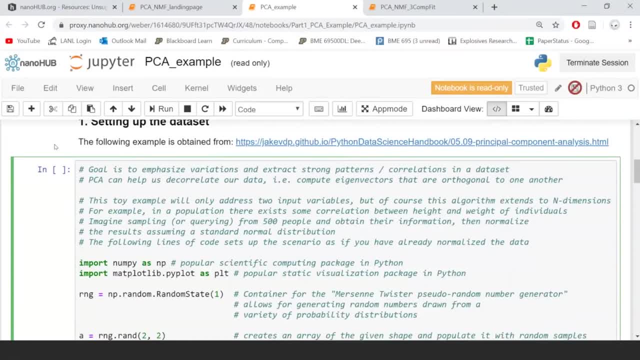 to understand how the algorithm actually works. So I'm going to go over this toy example where we're only going to address two input variables. But of course, as I stated, you can do PCA on n dimensions. So we're going to go over this toy example where we're only going to address two input variables. But of course, as I stated, you can do PCA on n dimensions. So we're going to go over this toy example, where we're only going to address two input variables, But of course, as I stated, you can do PCA on n dimensions. 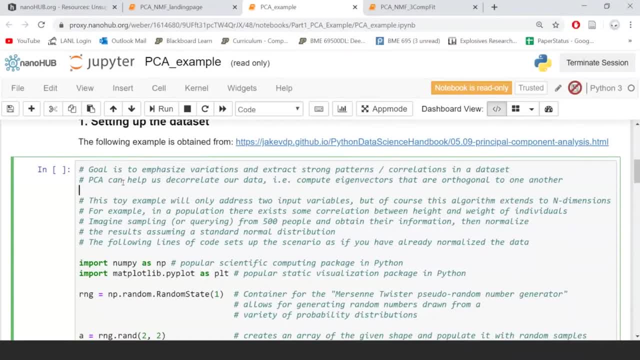 So we're going to go over this toy example where we're only going to address two input variables. But of course, as I stated, you can do PCA on n dimensions. So we're going to go over this toy example where we're only going to address two input. 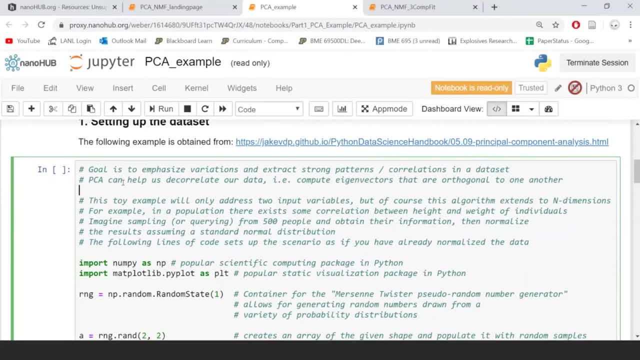 variables, But of course, as I stated, you can do PCA on n dimensions. So we're going to go over this toy example, where we're only going to address two input variables, But of course, as I stated, you can do PCA on n dimensions. 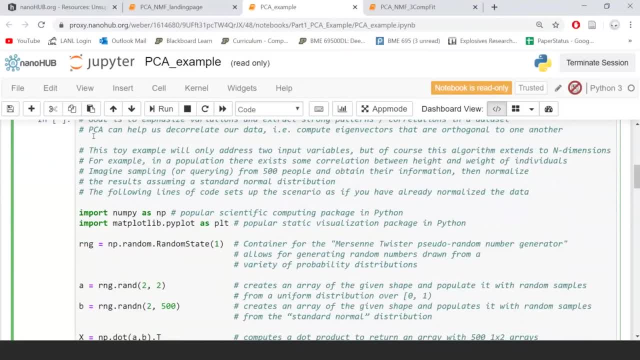 So we're going to go over this toy example where we're only going to address two input variables. But of course, as I stated, you can do PCA on n dimensions. So we're going to go over this toy example where we're only going to address two input. 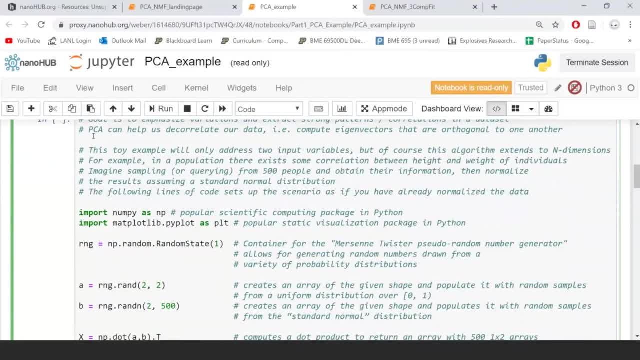 variables, But of course, as I stated, you can do PCA on n dimensions. So we're going to go over this toy example, where we're only going to address two input variables, But of course, as I stated, you can do PCA on n dimensions. 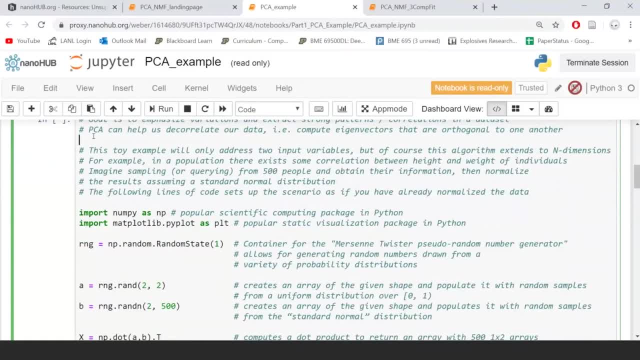 So we're going to go over this toy example where we're only going to address two input variables. But of course, as I stated, you can do PCA on n dimensions. So we're going to go over this toy example where we're only going to address two input. 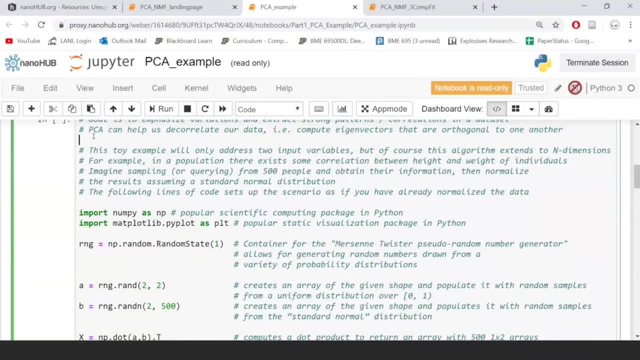 variables, But of course, as I stated, you can do PCA on n dimensions. So we're going to go over this toy example, where we're only going to address two input variables, But of course, as I stated, you can do PCA on n dimensions. 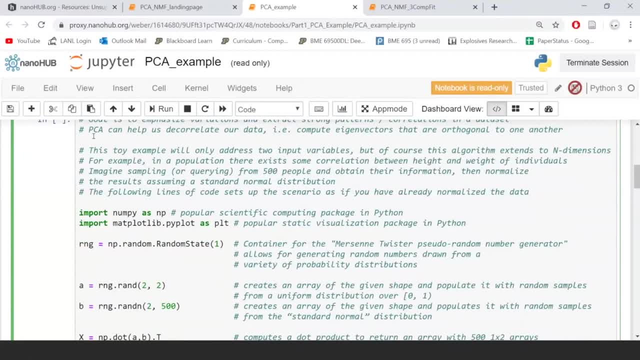 So we're going to go over this toy example where we're only going to address two input variables. But of course, as I stated, you can do PCA on n dimensions. So we're going to go over this toy example where we're only going to address two input. 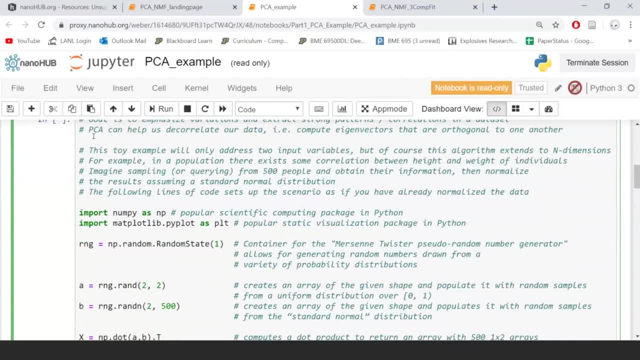 variables, But of course, as I stated, you can do PCA on n dimensions. So we're going to go over this toy example, where we're only going to address two input variables, But of course, as I stated, you can do PCA on n dimensions. 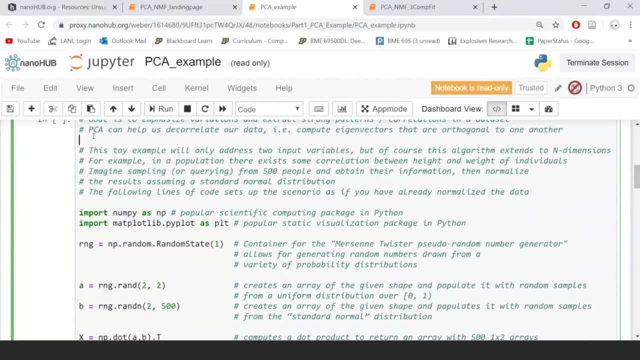 So we're going to go over this toy example where we're only going to address two input variables. But of course, as I stated, you can do PCA on n dimensions. So we're going to go over this toy example where we're only going to address two input. 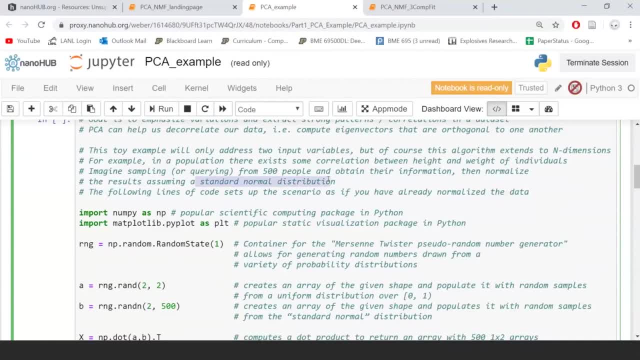 variables, But of course, as I stated, you can do PCA on n dimensions. So we're going to go over this toy example, where we're only going to address two input variables, But of course, as I stated, you can do PCA on n dimensions. 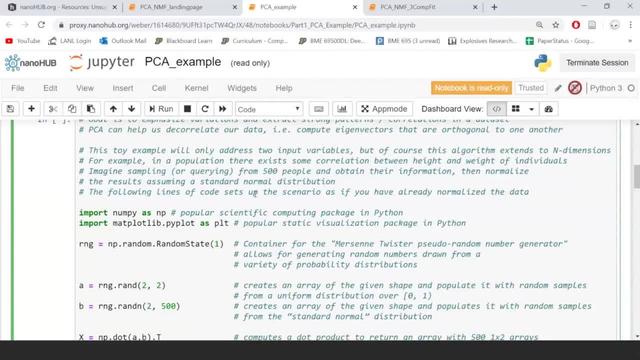 So we're going to go over this toy example where we're only going to address two input variables. But of course, as I stated, you can do PCA on n dimensions. So we're going to go over this toy example where we're only going to address two input. 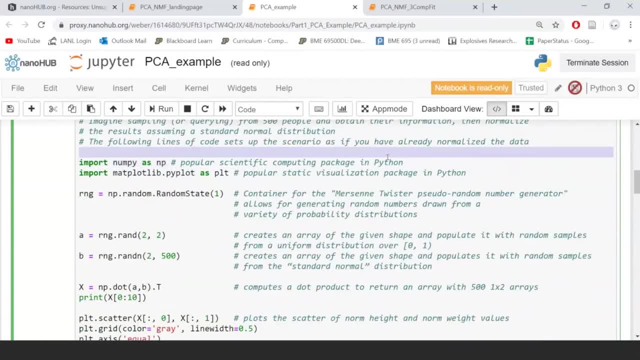 variables, But of course, as I stated, you can do PCA on n dimensions. So we're going to go over this toy example, where we're only going to address two input variables, But of course, as I stated, you can do PCA on n dimensions. 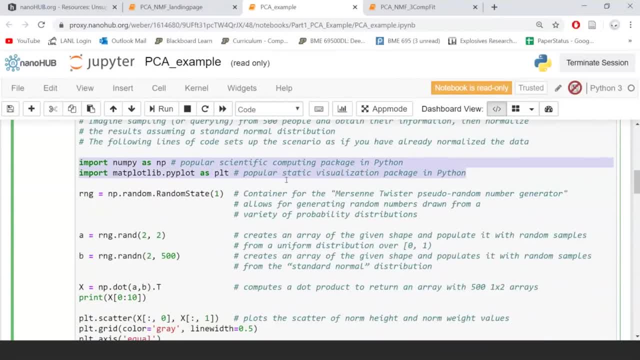 So we're going to go over this toy example where we're only going to address two input variables. But of course, as I stated, you can do PCA on n dimensions. So we're going to go over this toy example where we're only going to address two input. 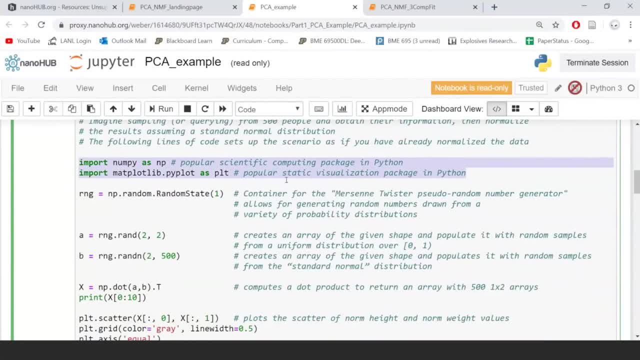 variables, But of course, as I stated, you can do PCA on n dimensions. So we're going to go over this toy example, where we're only going to address two input variables, But of course, as I stated, you can do PCA on n dimensions. 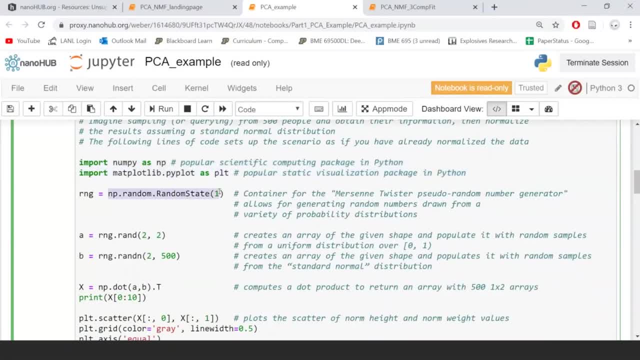 So we're going to go over this toy example where we're only going to address two input variables. But of course, as I stated, you can do PCA on n dimensions. So we're going to go over this toy example where we're only going to address two input. 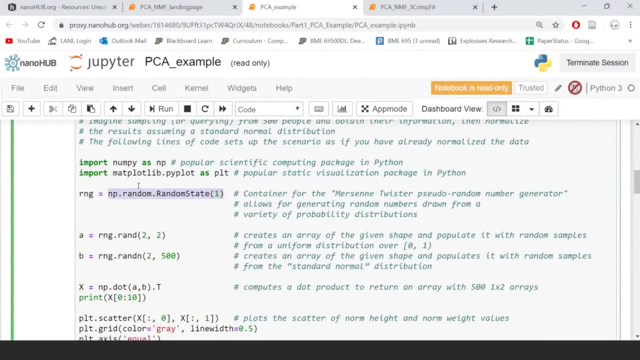 variables, But of course, as I stated, you can do PCA on n dimensions. So we're going to go over this toy example, where we're only going to address two input variables, But of course, as I stated, you can do PCA on n dimensions. 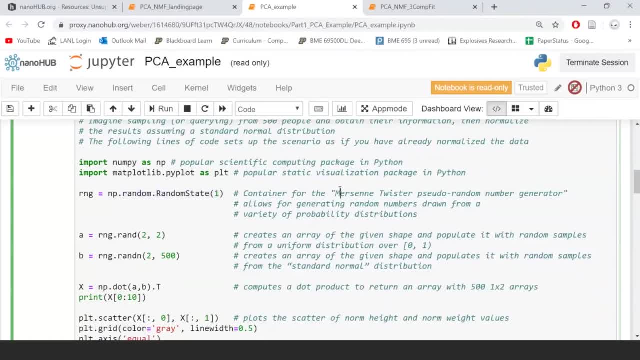 So we're going to go over this toy example where we're only going to address two input variables. But of course, as I stated, you can do PCA on n dimensions. So we're going to go over this toy example where we're only going to address two input. 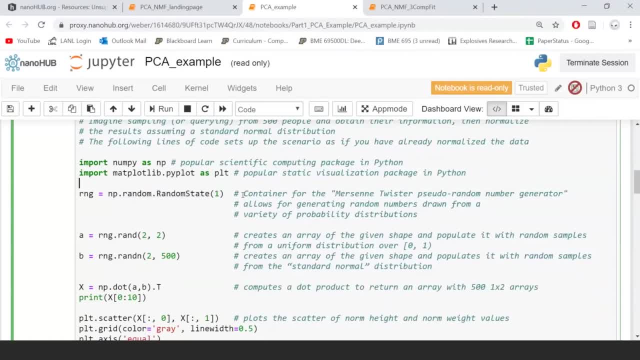 variables, But of course, as I stated, you can do PCA on n dimensions. So we're going to go over this toy example, where we're only going to address two input variables, But of course, as I stated, you can do PCA on n dimensions. 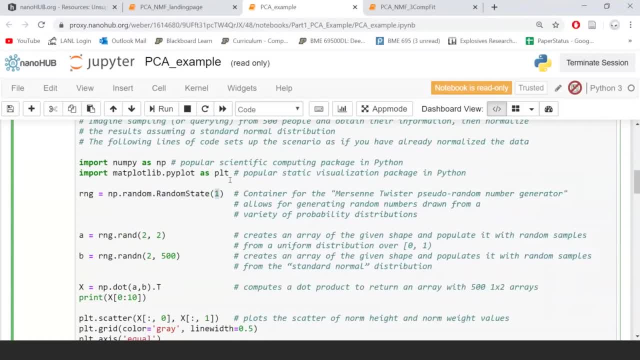 So we're going to go over this toy example where we're only going to address two input variables. But of course, as I stated, you can do PCA on n dimensions. So we're going to go over this toy example where we're only going to address two input. 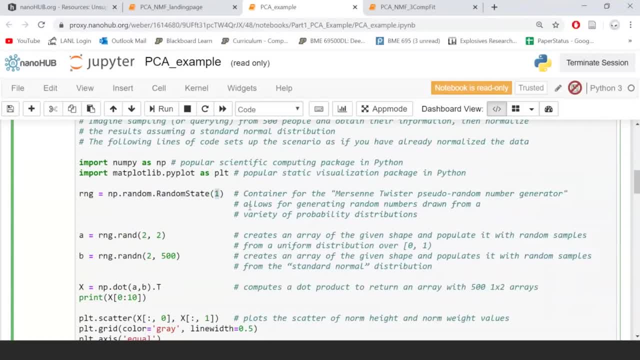 variables, But of course, as I stated, you can do PCA on n dimensions. So we're going to go over this toy example, where we're only going to address two input variables, But of course, as I stated, you can do PCA on n dimensions. 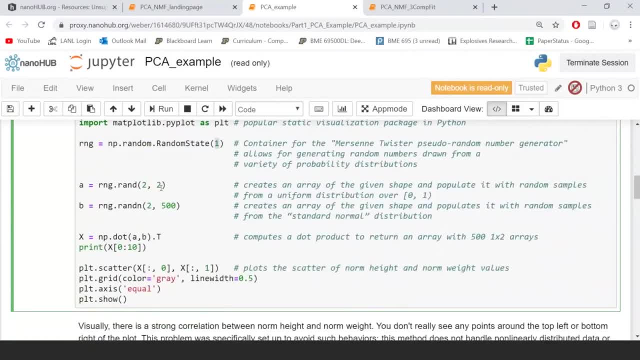 So we're going to go over this toy example where we're only going to address two input variables. But of course, as I stated, you can do PCA on n dimensions. So we're going to go over this toy example where we're only going to address two input. 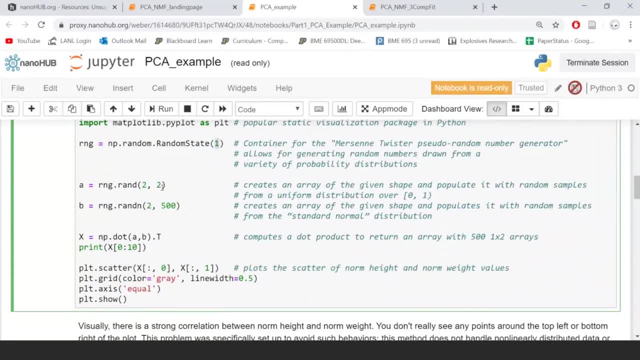 variables, But of course, as I stated, you can do PCA on n dimensions. So we're going to go over this toy example, where we're only going to address two input variables, But of course, as I stated, you can do PCA on n dimensions. 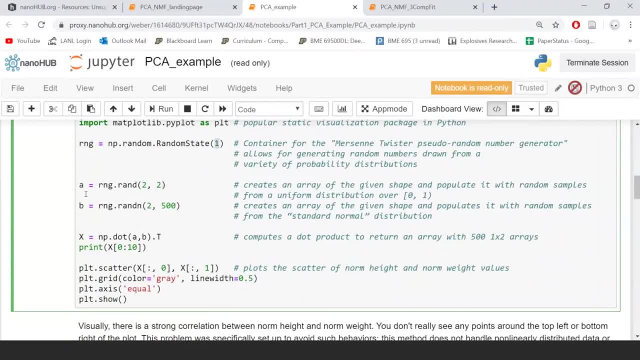 So we're going to go over this toy example where we're only going to address two input variables. But of course, as I stated, you can do PCA on n dimensions. So we're going to go over this toy example where we're only going to address two input. 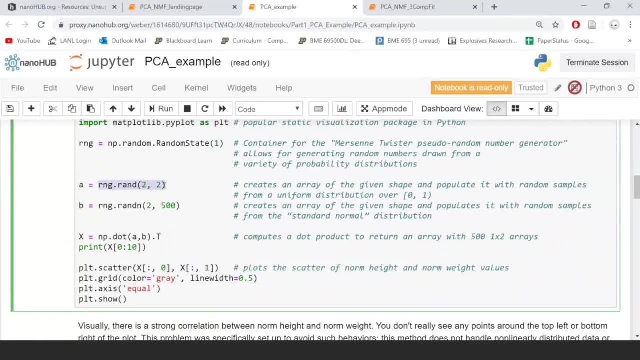 variables, But of course, as I stated, you can do PCA on n dimensions. So we're going to go over this toy example, where we're only going to address two input variables, But of course, as I stated, you can do PCA on n dimensions. 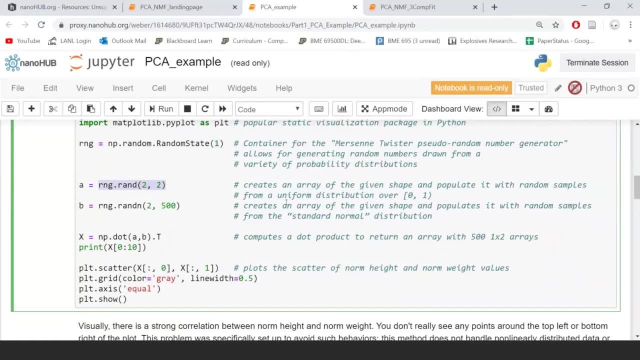 So we're going to go over this toy example where we're only going to address two input variables. But of course, as I stated, you can do PCA on n dimensions. So we're going to go over this toy example where we're only going to address two input. 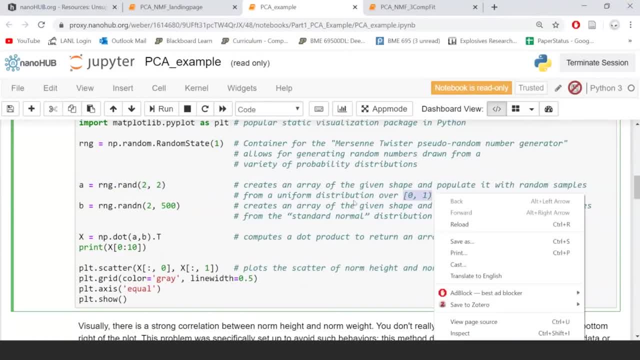 variables, But of course, as I stated, you can do PCA on n dimensions. So we're going to go over this toy example, where we're only going to address two input variables, But of course, as I stated, you can do PCA on n dimensions. 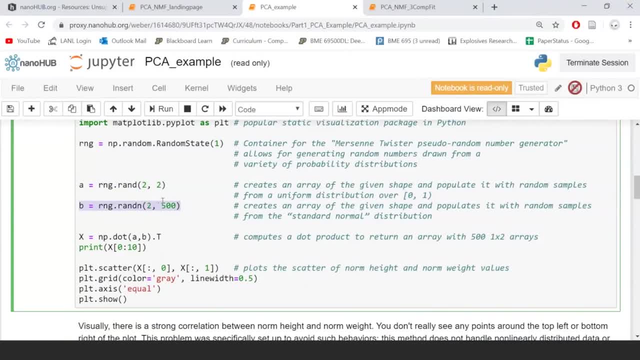 So we're going to go over this toy example where we're only going to address two input variables. But of course, as I stated, you can do PCA on n dimensions. So we're going to go over this toy example where we're only going to address two input. 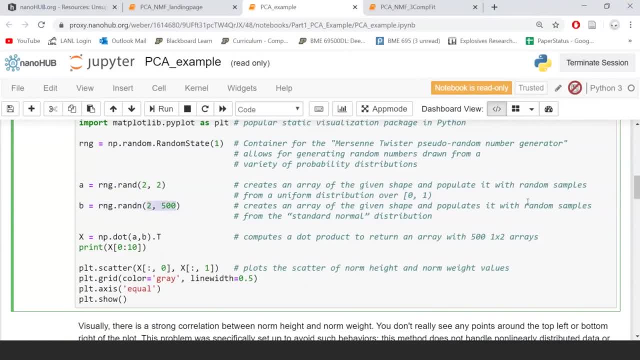 variables, But of course, as I stated, you can do PCA on n dimensions. So we're going to go over this toy example, where we're only going to address two input variables, But of course, as I stated, you can do PCA on n dimensions. 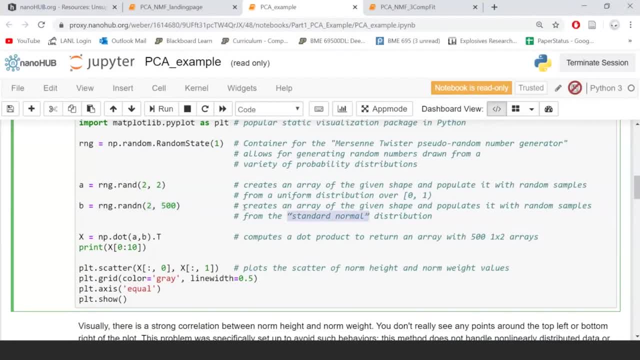 So we're going to go over this toy example where we're only going to address two input variables. But of course, as I stated, you can do PCA on n dimensions. So we're going to go over this toy example where we're only going to address two input. 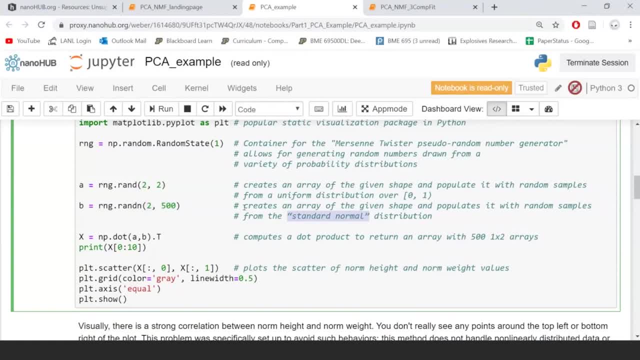 variables, But of course, as I stated, you can do PCA on n dimensions. So we're going to go over this toy example, where we're only going to address two input variables, But of course, as I stated, you can do PCA on n dimensions. 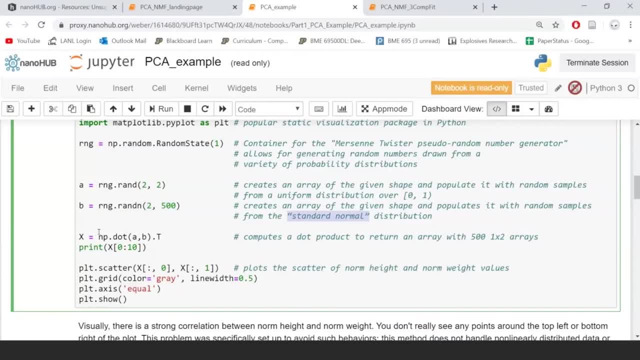 So we're going to go over this toy example where we're only going to address two input variables. But of course, as I stated, you can do PCA on n dimensions. So we're going to go over this toy example where we're only going to address two input. 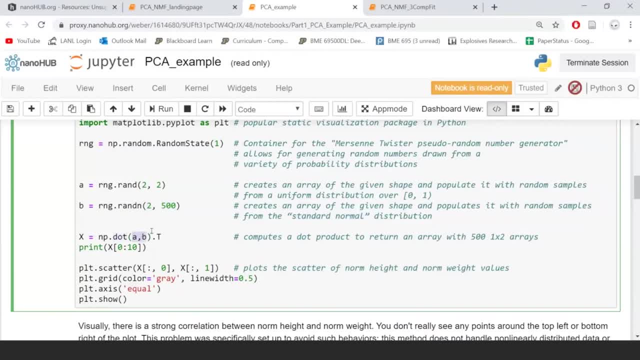 variables, But of course, as I stated, you can do PCA on n dimensions. So we're going to go over this toy example, where we're only going to address two input variables, But of course, as I stated, you can do PCA on n dimensions. 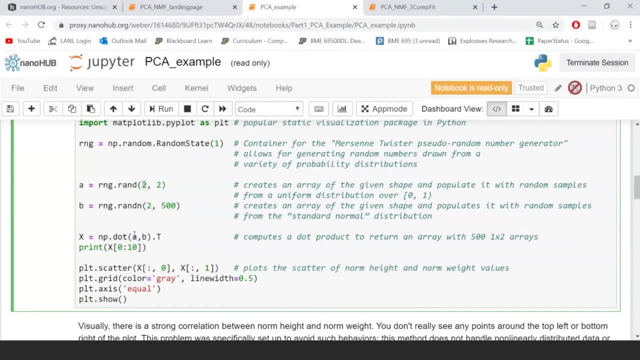 So we're going to go over this toy example where we're only going to address two input variables. But of course, as I stated, you can do PCA on n dimensions. So we're going to go over this toy example where we're only going to address two input. 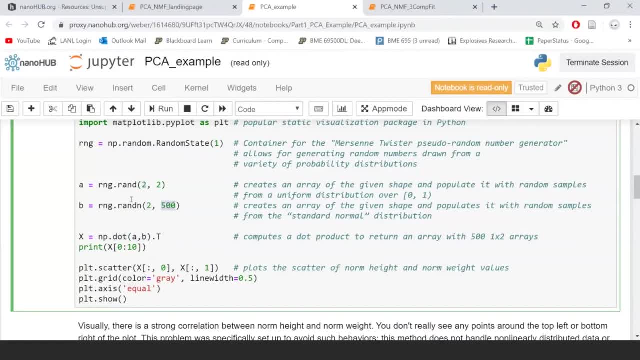 variables, But of course, as I stated, you can do PCA on n dimensions. So we're going to go over this toy example, where we're only going to address two input variables, But of course, as I stated, you can do PCA on n dimensions. 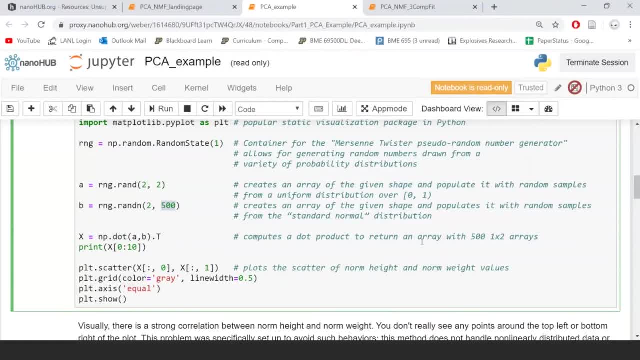 So we're going to go over this toy example where we're only going to address two input variables. But of course, as I stated, you can do PCA on n dimensions. So we're going to go over this toy example where we're only going to address two input. 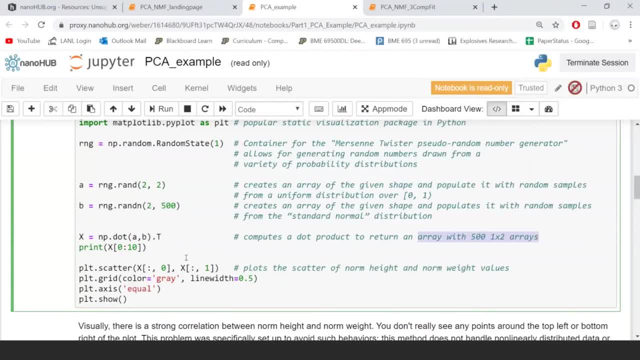 variables, But of course, as I stated, you can do PCA on n dimensions. So we're going to go over this toy example, where we're only going to address two input variables, But of course, as I stated, you can do PCA on n dimensions. 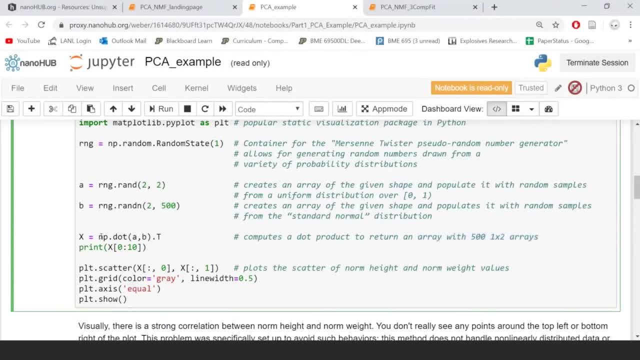 So we're going to go over this toy example where we're only going to address two input variables. But of course, as I stated, you can do PCA on n dimensions. So we're going to go over this toy example where we're only going to address two input. 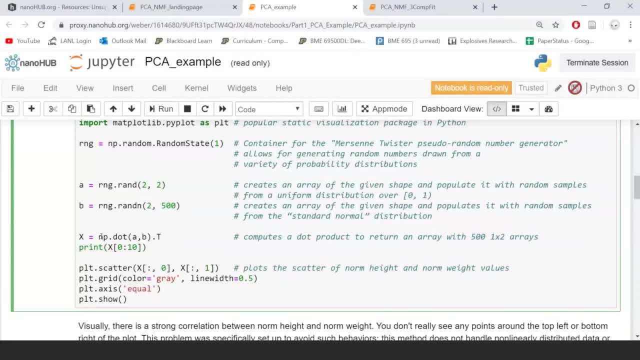 variables, But of course, as I stated, you can do PCA on n dimensions. So we're going to go over this toy example, where we're only going to address two input variables, But of course, as I stated, you can do PCA on n dimensions. 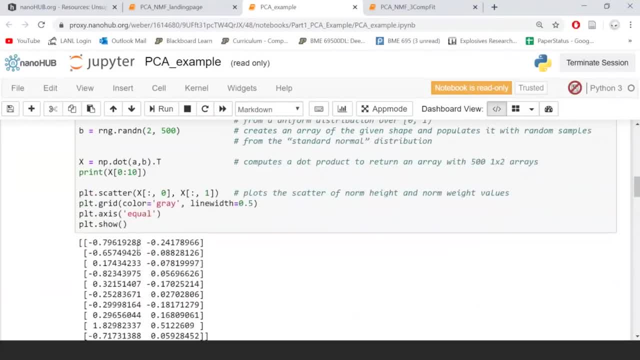 So we're going to go over this toy example where we're only going to address two input variables. But of course, as I stated, you can do PCA on n dimensions. So we're going to go over this toy example where we're only going to address two input. 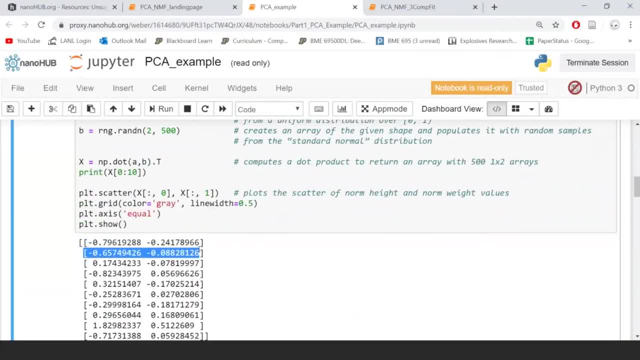 variables, But of course, as I stated, you can do PCA on n dimensions. So we're going to go over this toy example, where we're only going to address two input variables, But of course, as I stated, you can do PCA on n dimensions. 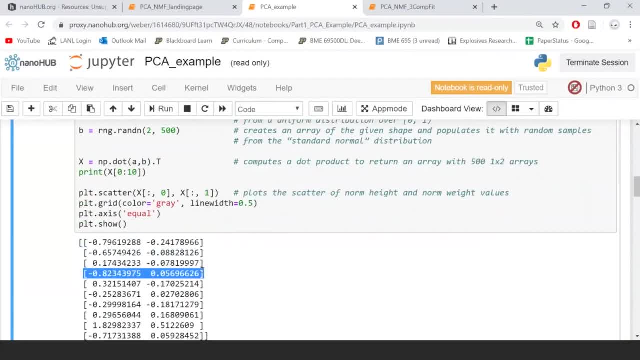 So we're going to go over this toy example where we're only going to address two input variables. But of course, as I stated, you can do PCA on n dimensions. So we're going to go over this toy example where we're only going to address two input. 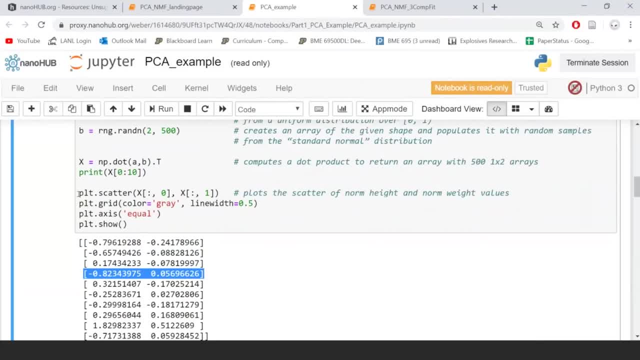 variables, But of course, as I stated, you can do PCA on n dimensions. So we're going to go over this toy example, where we're only going to address two input variables, But of course, as I stated, you can do PCA on n dimensions. 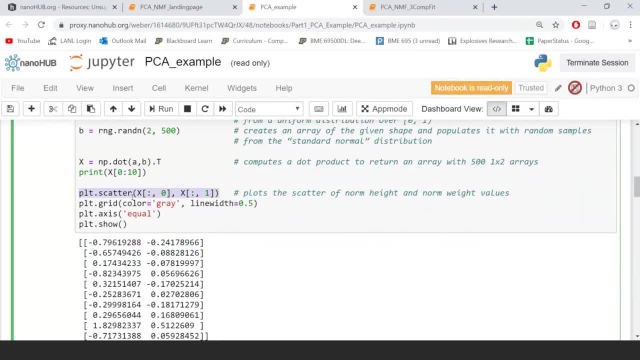 So we're going to go over this toy example where we're only going to address two input variables. But of course, as I stated, you can do PCA on n dimensions. So we're going to go over this toy example where we're only going to address two input. 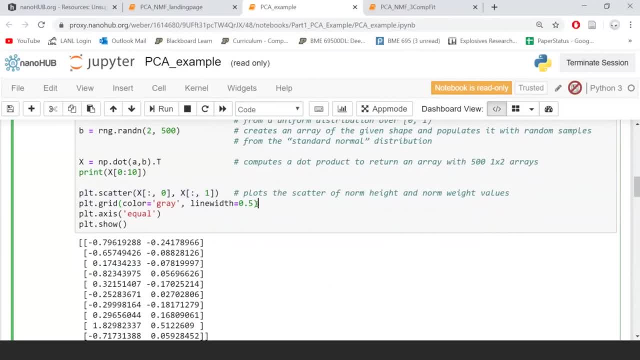 variables, But of course, as I stated, you can do PCA on n dimensions. So we're going to go over this toy example, where we're only going to address two input variables, But of course, as I stated, you can do PCA on n dimensions. 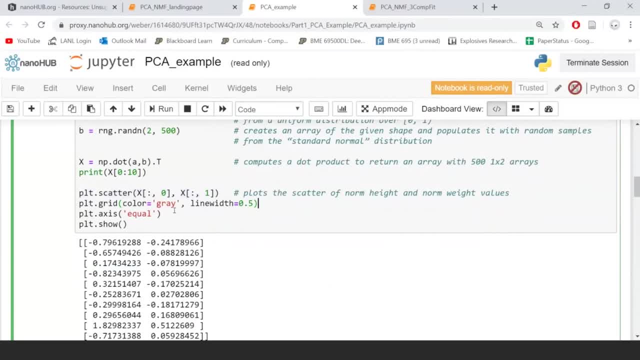 So we're going to go over this toy example where we're only going to address two input variables. But of course, as I stated, you can do PCA on n dimensions. So we're going to go over this toy example where we're only going to address two input. 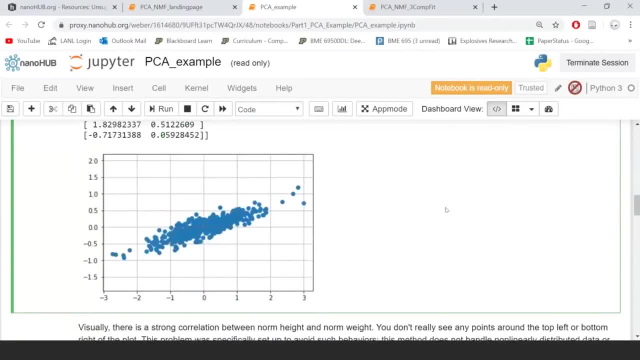 variables, But of course, as I stated, you can do PCA on n dimensions. So we're going to go over this toy example, where we're only going to address two input variables, But of course, as I stated, you can do PCA on n dimensions. 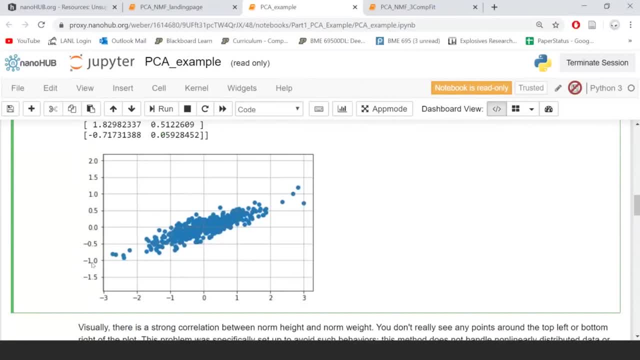 So we're going to go over this toy example where we're only going to address two input variables. But of course, as I stated, you can do PCA on n dimensions. So we're going to go over this toy example where we're only going to address two input. 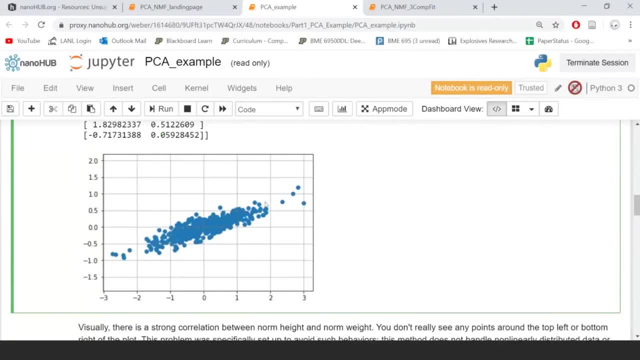 variables, But of course, as I stated, you can do PCA on n dimensions. So we're going to go over this toy example, where we're only going to address two input variables, But of course, as I stated, you can do PCA on n dimensions. 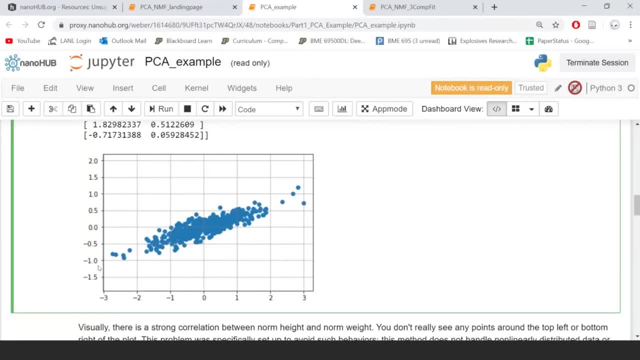 So we're going to go over this toy example where we're only going to address two input variables. But of course, as I stated, you can do PCA on n dimensions. So we're going to go over this toy example where we're only going to address two input. 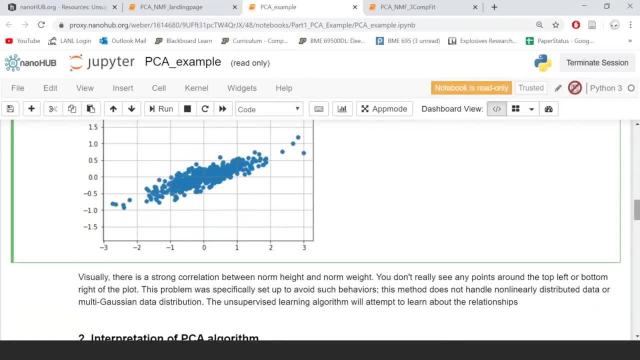 variables, But of course, as I stated, you can do PCA on n dimensions. So we're going to go over this toy example, where we're only going to address two input variables, But of course, as I stated, you can do PCA on n dimensions. 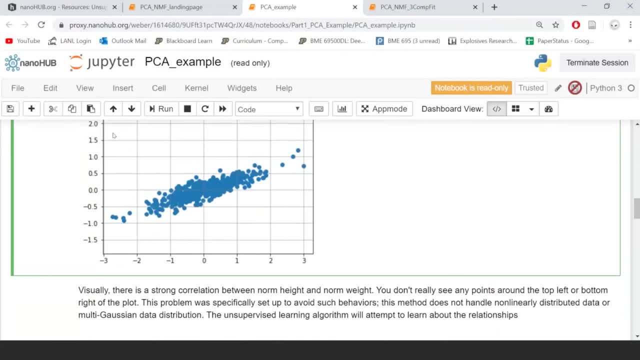 So we're going to go over this toy example where we're only going to address two input variables. But of course, as I stated, you can do PCA on n dimensions. So we're going to go over this toy example where we're only going to address two input. 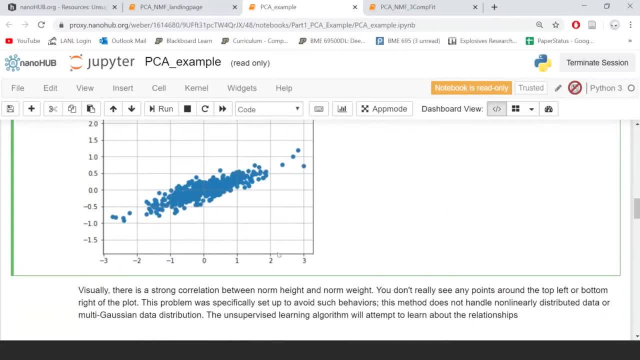 variables, But of course, as I stated, you can do PCA on n dimensions. So we're going to go over this toy example, where we're only going to address two input variables, But of course, as I stated, you can do PCA on n dimensions. 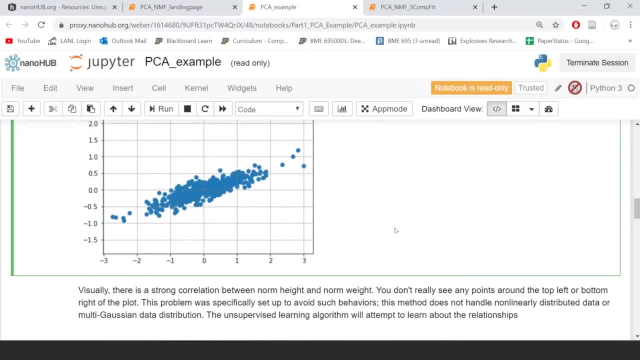 So we're going to go over this toy example where we're only going to address two input variables. But of course, as I stated, you can do PCA on n dimensions. So we're going to go over this toy example where we're only going to address two input. 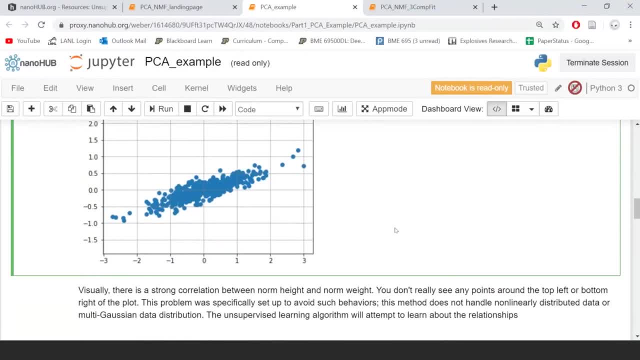 variables, But of course, as I stated, you can do PCA on n dimensions. So we're going to go over this toy example, where we're only going to address two input variables, But of course, as I stated, you can do PCA on n dimensions. 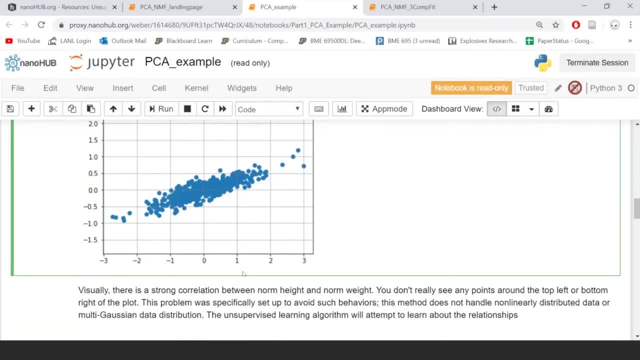 So we're going to go over this toy example where we're only going to address two input variables. But of course, as I stated, you can do PCA on n dimensions. So we're going to go over this toy example where we're only going to address two input. 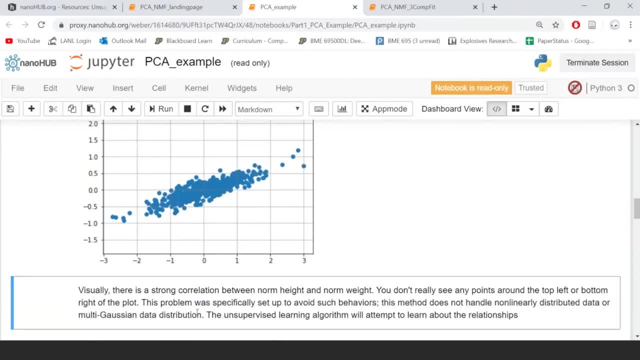 variables, But of course, as I stated, you can do PCA on n dimensions. So we're going to go over this toy example, where we're only going to address two input variables, But of course, as I stated, you can do PCA on n dimensions. 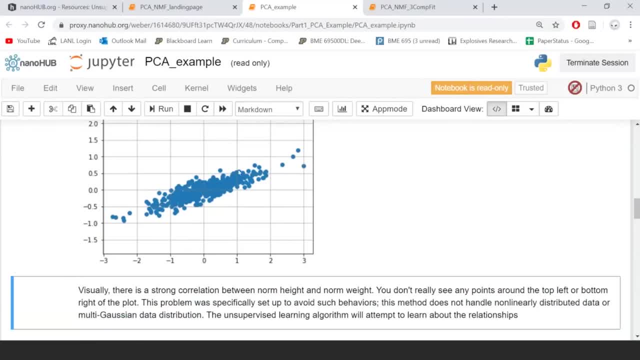 So we're going to go over this toy example where we're only going to address two input variables. But of course, as I stated, you can do PCA on n dimensions. So we're going to go over this toy example where we're only going to address two input. 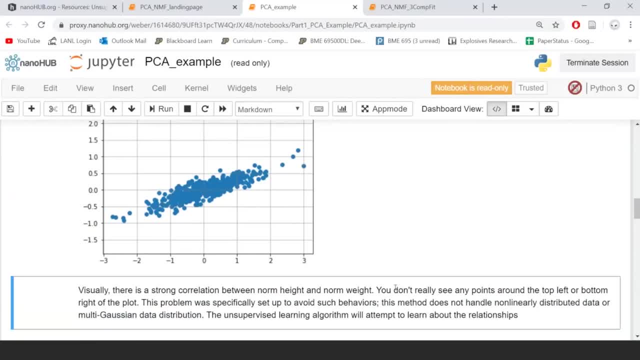 variables, But of course, as I stated, you can do PCA on n dimensions. So we're going to go over this toy example, where we're only going to address two input variables, But of course, as I stated, you can do PCA on n dimensions. 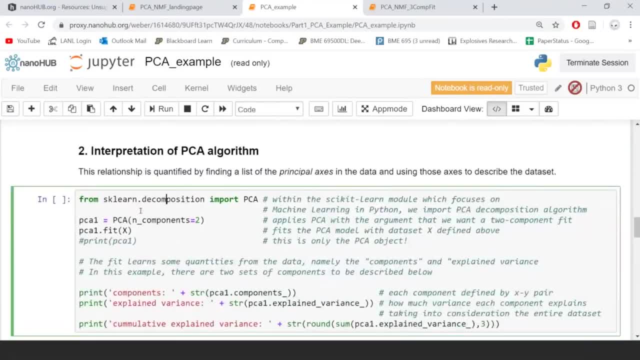 So we're going to go over this toy example where we're only going to address two input variables. But of course, as I stated, you can do PCA on n dimensions. So we're going to go over this toy example where we're only going to address two input. 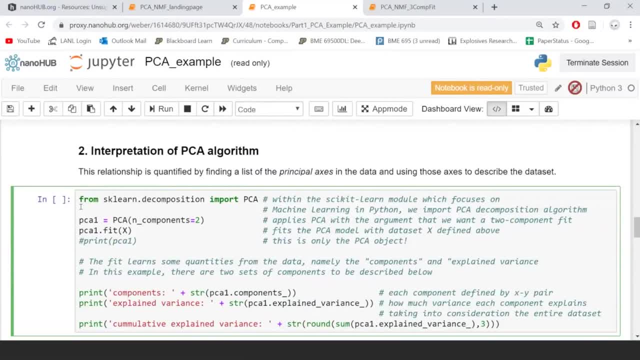 variables, But of course, as I stated, you can do PCA on n dimensions. So we're going to go over this toy example, where we're only going to address two input variables, But of course, as I stated, you can do PCA on n dimensions. 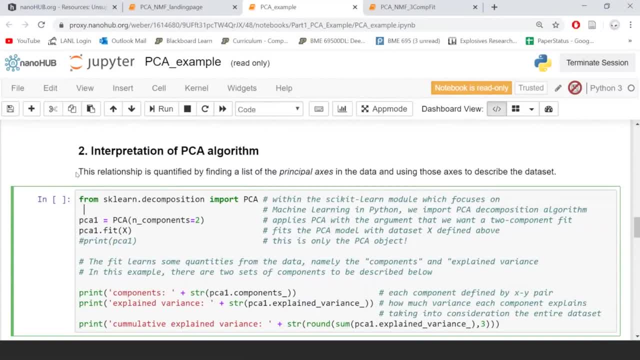 So we're going to go over this toy example where we're only going to address two input variables. But of course, as I stated, you can do PCA on n dimensions. So we're going to go over this toy example where we're only going to address two input. 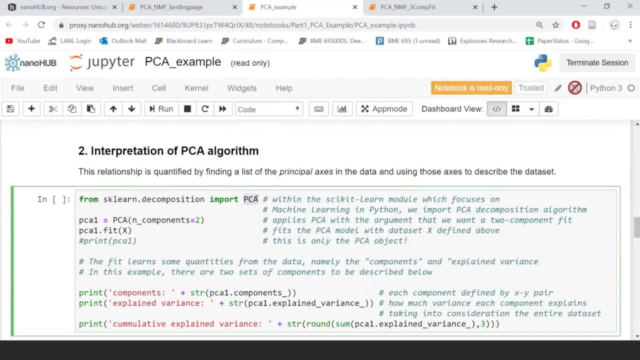 variables, But of course, as I stated, you can do PCA on n dimensions. So we're going to go over this toy example, where we're only going to address two input variables, But of course, as I stated, you can do PCA on n dimensions. 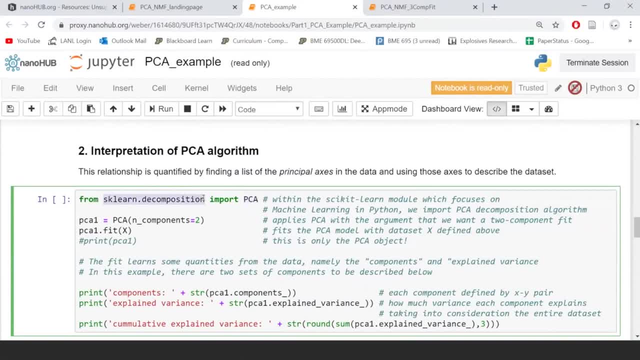 So we're going to go over this toy example where we're only going to address two input variables. But of course, as I stated, you can do PCA on n dimensions. So we're going to go over this toy example where we're only going to address two input. 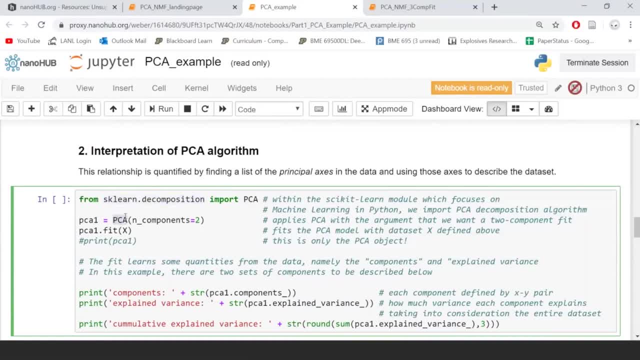 variables, But of course, as I stated, you can do PCA on n dimensions. So we're going to go over this toy example, where we're only going to address two input variables, But of course, as I stated, you can do PCA on n dimensions. 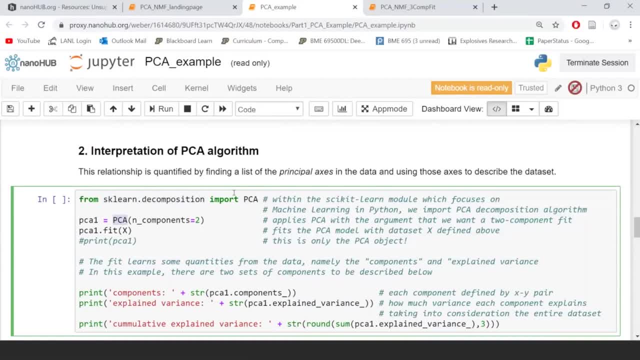 So we're going to go over this toy example where we're only going to address two input variables. But of course, as I stated, you can do PCA on n dimensions. So we're going to go over this toy example where we're only going to address two input. 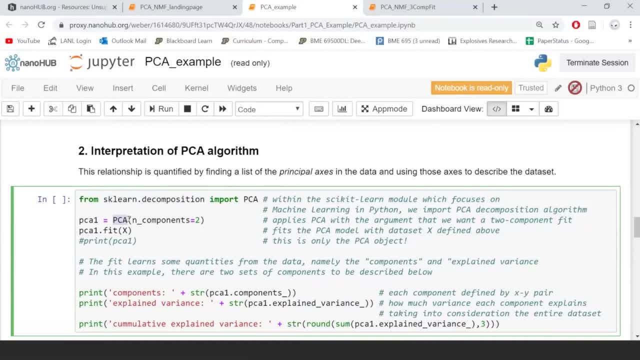 variables, But of course, as I stated, you can do PCA on n dimensions. So we're going to go over this toy example, where we're only going to address two input variables, But of course, as I stated, you can do PCA on n dimensions. 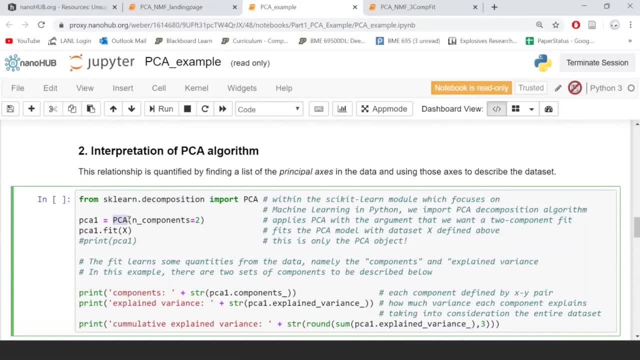 So we're going to go over this toy example where we're only going to address two input variables. But of course, as I stated, you can do PCA on n dimensions. So we're going to go over this toy example where we're only going to address two input. 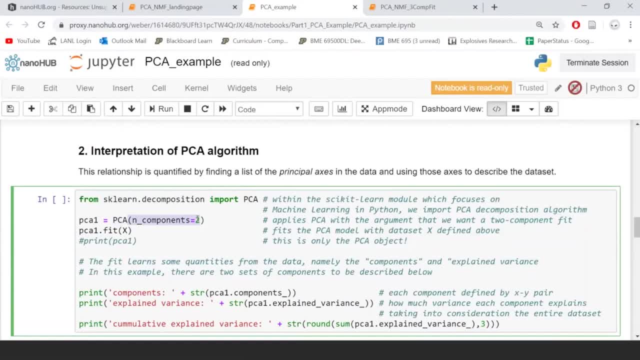 variables, But of course, as I stated, you can do PCA on n dimensions. So we're going to go over this toy example, where we're only going to address two input variables, But of course, as I stated, you can do PCA on n dimensions. 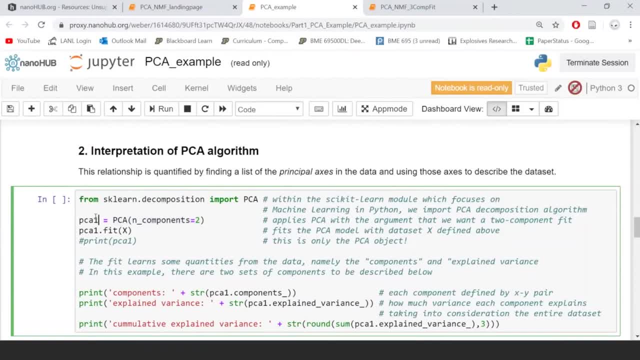 So we're going to go over this toy example where we're only going to address two input variables. But of course, as I stated, you can do PCA on n dimensions. So we're going to go over this toy example where we're only going to address two input. 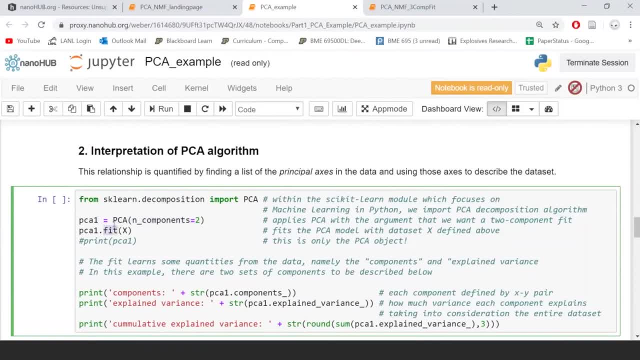 variables, But of course, as I stated, you can do PCA on n dimensions. So we're going to go over this toy example, where we're only going to address two input variables, But of course, as I stated, you can do PCA on n dimensions. 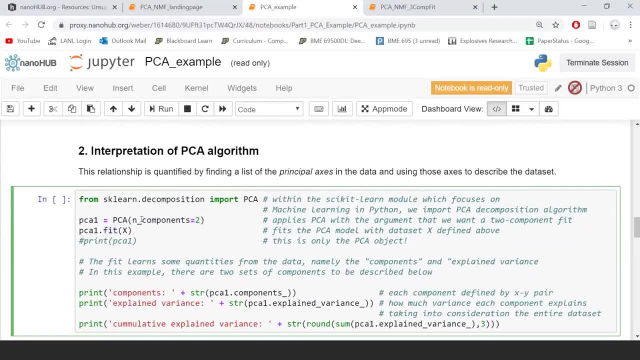 So we're going to go over this toy example where we're only going to address two input variables. But of course, as I stated, you can do PCA on n dimensions. So we're going to go over this toy example where we're only going to address two input. 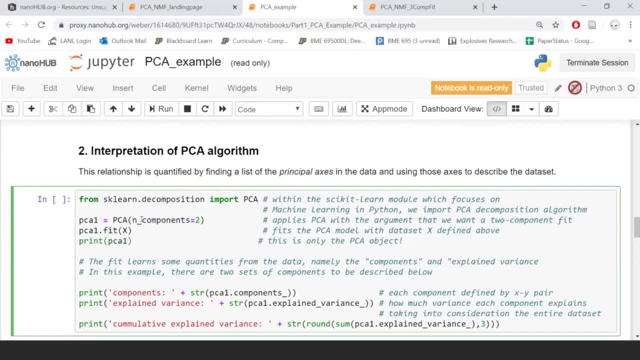 variables, But of course, as I stated, you can do PCA on n dimensions. So we're going to go over this toy example, where we're only going to address two input variables, But of course, as I stated, you can do PCA on n dimensions. 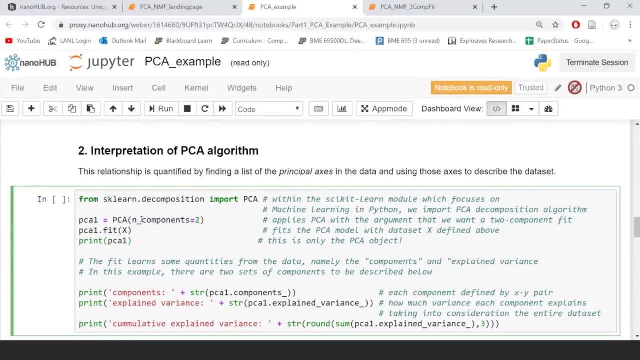 So we're going to go over this toy example where we're only going to address two input variables. But of course, as I stated, you can do PCA on n dimensions. So we're going to go over this toy example where we're only going to address two input. 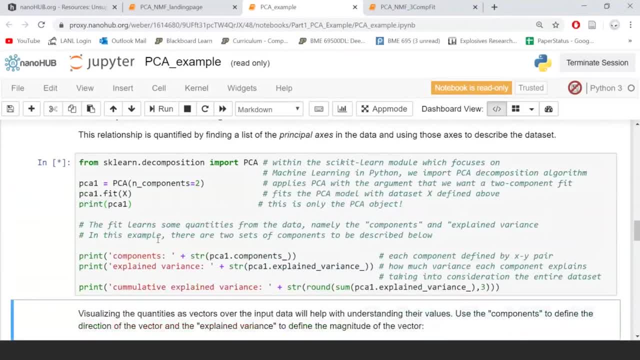 variables, But of course, as I stated, you can do PCA on n dimensions. So we're going to go over this toy example, where we're only going to address two input variables, But of course, as I stated, you can do PCA on n dimensions. 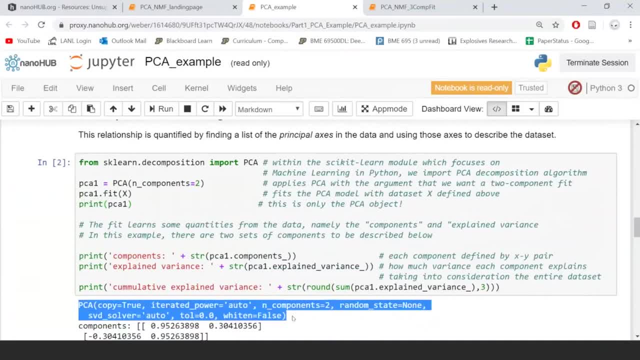 So we're going to go over this toy example where we're only going to address two input variables. But of course, as I stated, you can do PCA on n dimensions. So we're going to go over this toy example where we're only going to address two input. 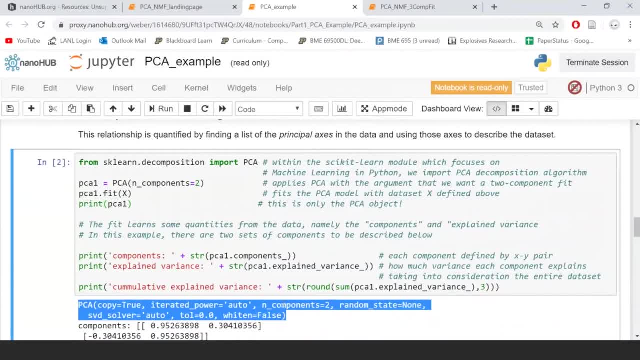 variables, But of course, as I stated, you can do PCA on n dimensions. So we're going to go over this toy example, where we're only going to address two input variables, But of course, as I stated, you can do PCA on n dimensions. 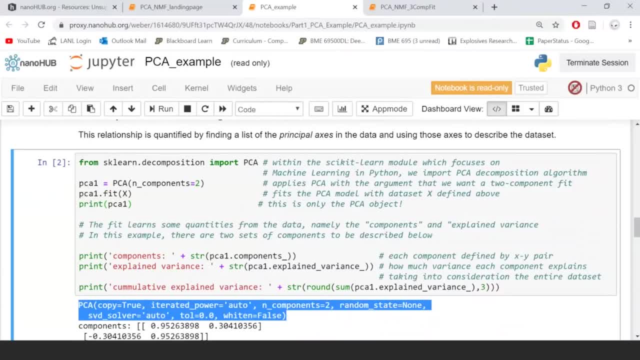 So we're going to go over this toy example where we're only going to address two input variables. But of course, as I stated, you can do PCA on n dimensions. So we're going to go over this toy example where we're only going to address two input. 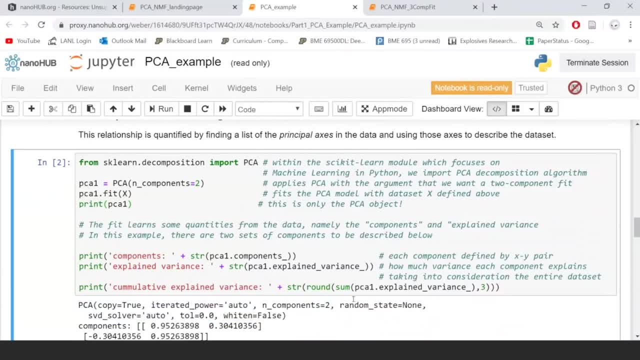 variables, But of course, as I stated, you can do PCA on n dimensions. So we're going to go over this toy example, where we're only going to address two input variables, But of course, as I stated, you can do PCA on n dimensions. 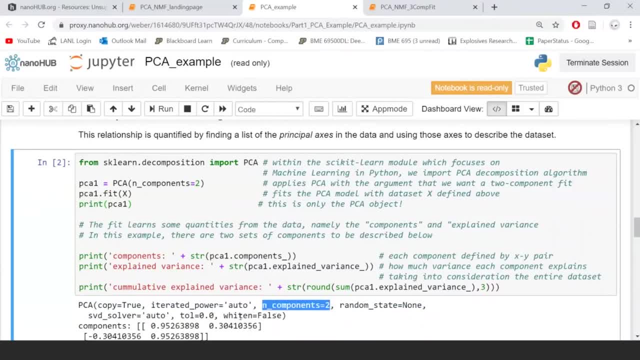 So we're going to go over this toy example where we're only going to address two input variables. But of course, as I stated, you can do PCA on n dimensions. So we're going to go over this toy example where we're only going to address two input. 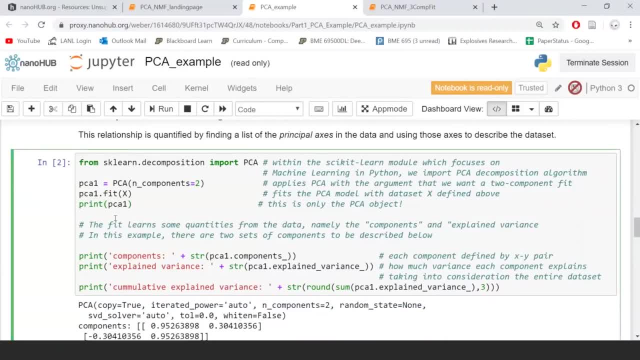 variables, But of course, as I stated, you can do PCA on n dimensions. So we're going to go over this toy example, where we're only going to address two input variables, But of course, as I stated, you can do PCA on n dimensions. 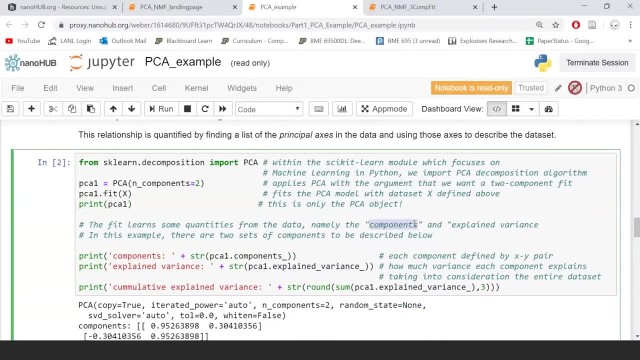 So we're going to go over this toy example where we're only going to address two input variables. But of course, as I stated, you can do PCA on n dimensions. So we're going to go over this toy example where we're only going to address two input. 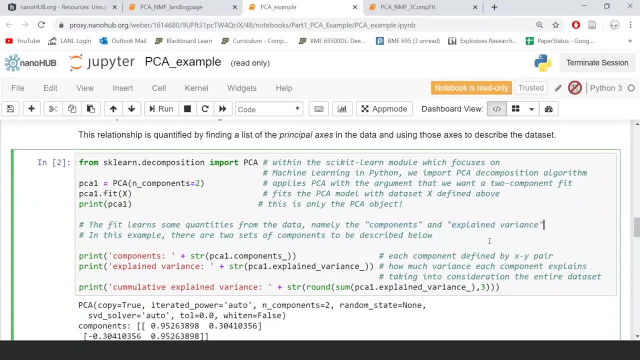 variables, But of course, as I stated, you can do PCA on n dimensions. So we're going to go over this toy example, where we're only going to address two input variables, But of course, as I stated, you can do PCA on n dimensions. 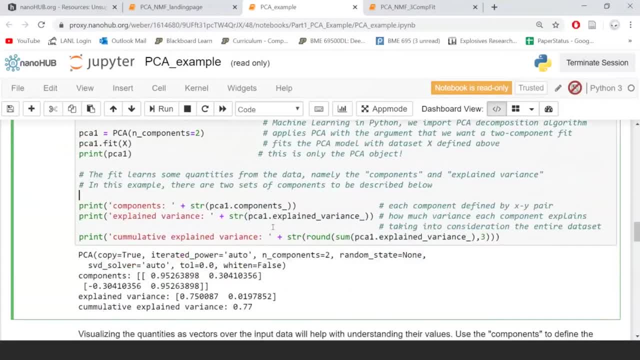 So we're going to go over this toy example where we're only going to address two input variables. But of course, as I stated, you can do PCA on n dimensions. So we're going to go over this toy example where we're only going to address two input. 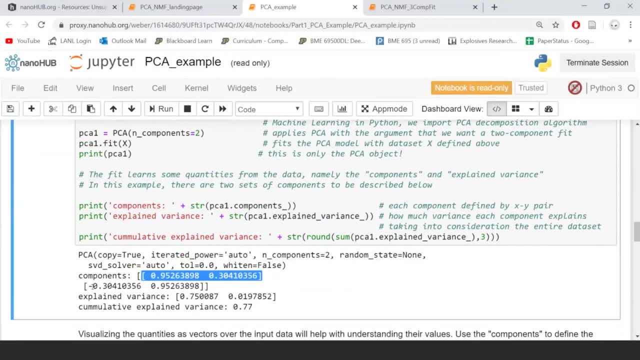 variables, But of course, as I stated, you can do PCA on n dimensions. So we're going to go over this toy example, where we're only going to address two input variables, But of course, as I stated, you can do PCA on n dimensions. 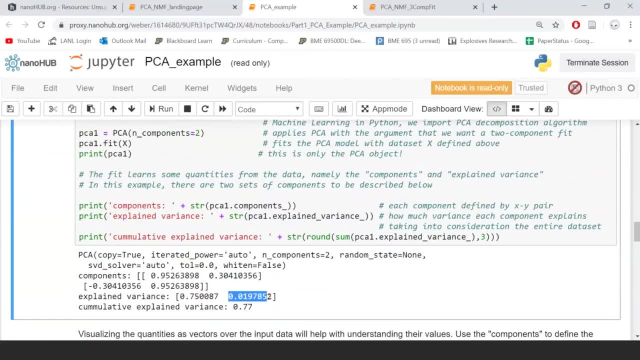 So we're going to go over this toy example where we're only going to address two input variables. But of course, as I stated, you can do PCA on n dimensions. So we're going to go over this toy example where we're only going to address two input. 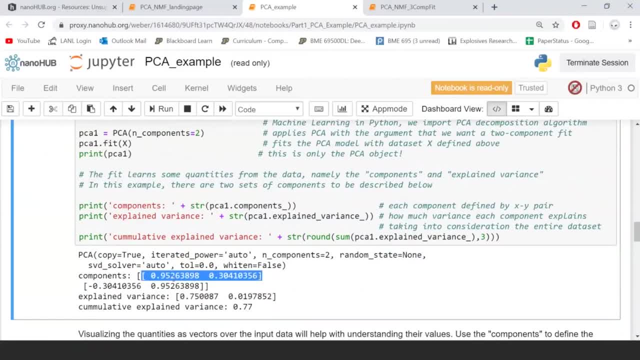 variables, But of course, as I stated, you can do PCA on n dimensions. So we're going to go over this toy example, where we're only going to address two input variables, But of course, as I stated, you can do PCA on n dimensions. 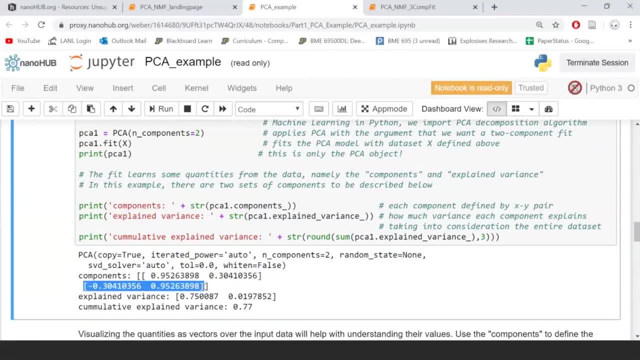 So we're going to go over this toy example where we're only going to address two input variables. But of course, as I stated, you can do PCA on n dimensions. So we're going to go over this toy example where we're only going to address two input. 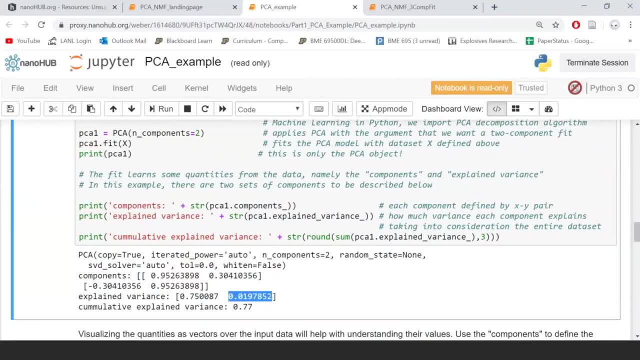 variables, But of course, as I stated, you can do PCA on n dimensions. So we're going to go over this toy example, where we're only going to address two input variables, But of course, as I stated, you can do PCA on n dimensions. 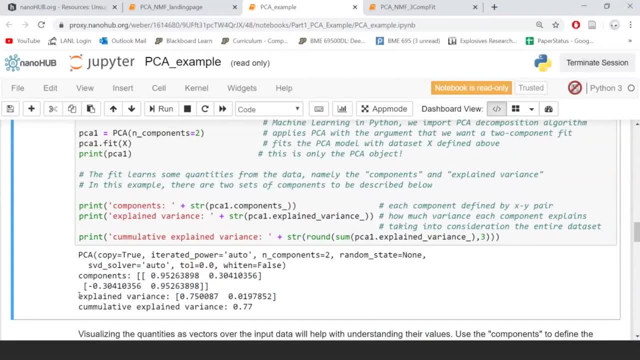 So we're going to go over this toy example where we're only going to address two input variables. But of course, as I stated, you can do PCA on n dimensions. So we're going to go over this toy example where we're only going to address two input. 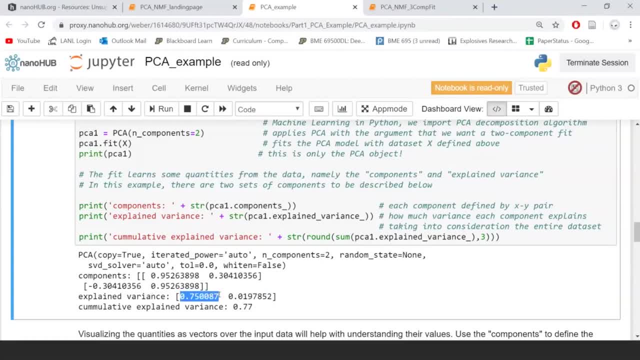 variables, But of course, as I stated, you can do PCA on n dimensions. So we're going to go over this toy example, where we're only going to address two input variables, But of course, as I stated, you can do PCA on n dimensions. 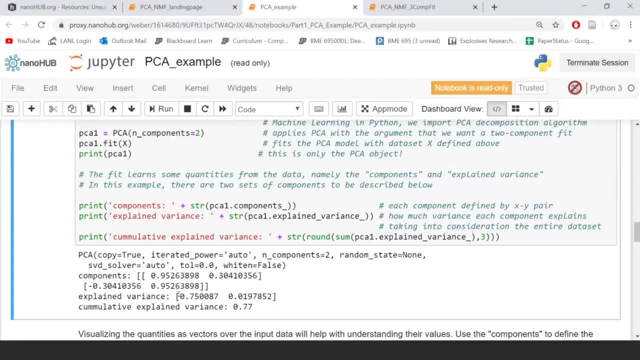 So we're going to go over this toy example where we're only going to address two input variables. But of course, as I stated, you can do PCA on n dimensions. So we're going to go over this toy example where we're only going to address two input. 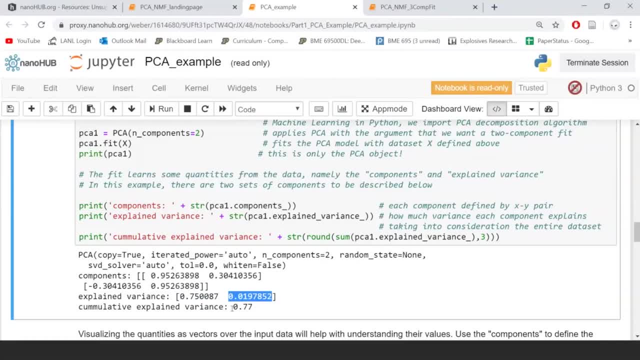 variables, But of course, as I stated, you can do PCA on n dimensions. So we're going to go over this toy example, where we're only going to address two input variables, But of course, as I stated, you can do PCA on n dimensions. 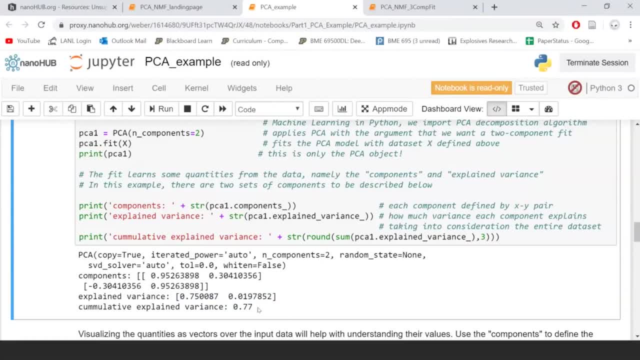 So we're going to go over this toy example where we're only going to address two input variables. But of course, as I stated, you can do PCA on n dimensions. So we're going to go over this toy example where we're only going to address two input. 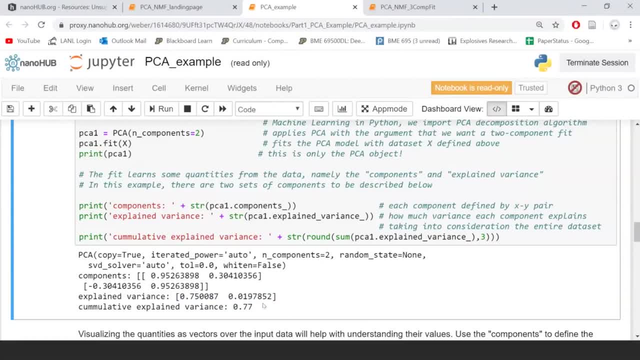 variables, But of course, as I stated, you can do PCA on n dimensions. So we're going to go over this toy example, where we're only going to address two input variables, But of course, as I stated, you can do PCA on n dimensions. 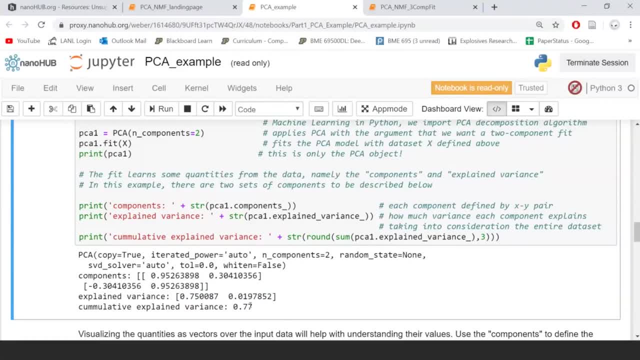 So we're going to go over this toy example where we're only going to address two input variables. But of course, as I stated, you can do PCA on n dimensions. So we're going to go over this toy example where we're only going to address two input. 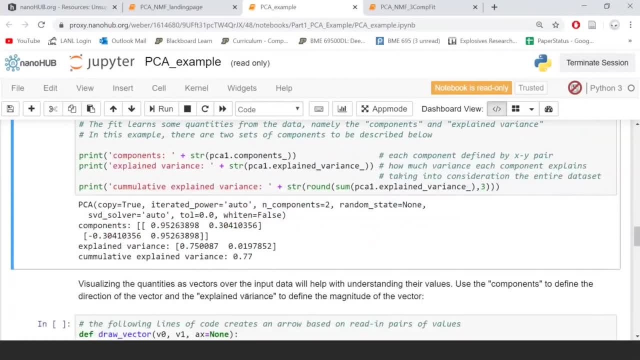 variables, But of course, as I stated, you can do PCA on n dimensions. So we're going to go over this toy example, where we're only going to address two input variables, But of course, as I stated, you can do PCA on n dimensions. 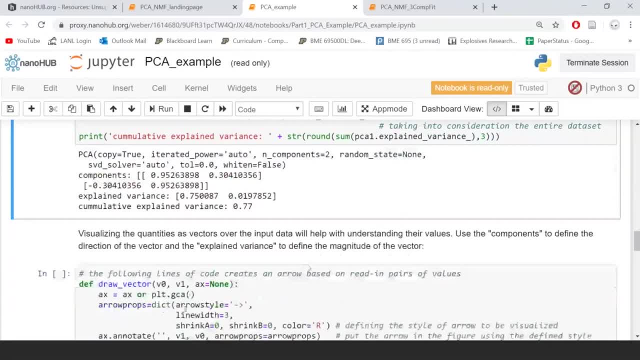 So we're going to go over this toy example where we're only going to address two input variables. But of course, as I stated, you can do PCA on n dimensions. So we're going to go over this toy example where we're only going to address two input. 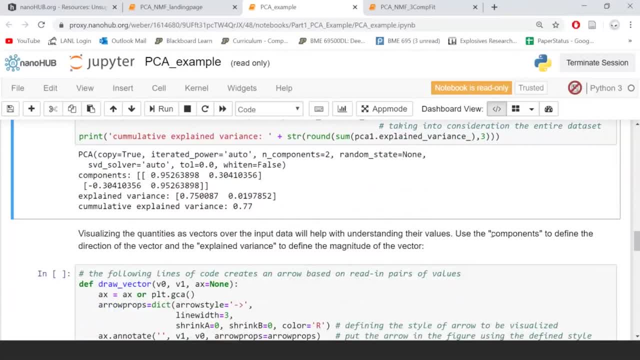 variables, But of course, as I stated, you can do PCA on n dimensions. So we're going to go over this toy example, where we're only going to address two input variables, But of course, as I stated, you can do PCA on n dimensions. 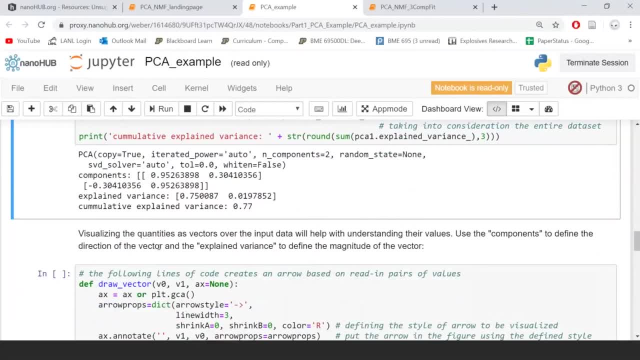 So we're going to go over this toy example where we're only going to address two input variables. But of course, as I stated, you can do PCA on n dimensions. So we're going to go over this toy example where we're only going to address two input. 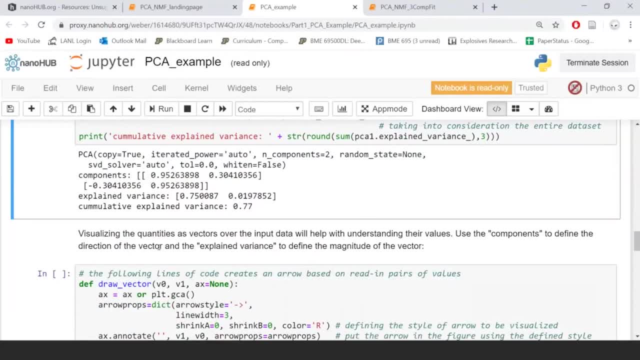 variables, But of course, as I stated, you can do PCA on n dimensions. So we're going to go over this toy example, where we're only going to address two input variables, But of course, as I stated, you can do PCA on n dimensions. 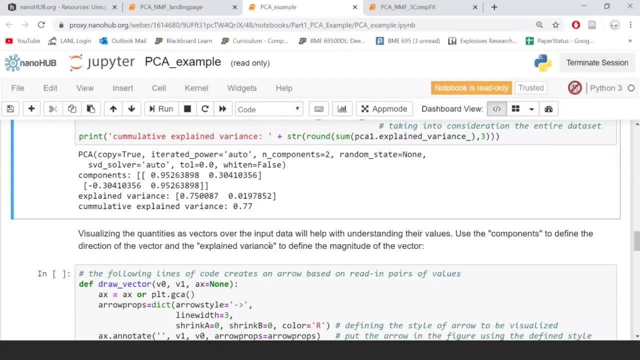 So we're going to go over this toy example where we're only going to address two input variables. But of course, as I stated, you can do PCA on n dimensions. So we're going to go over this toy example where we're only going to address two input. 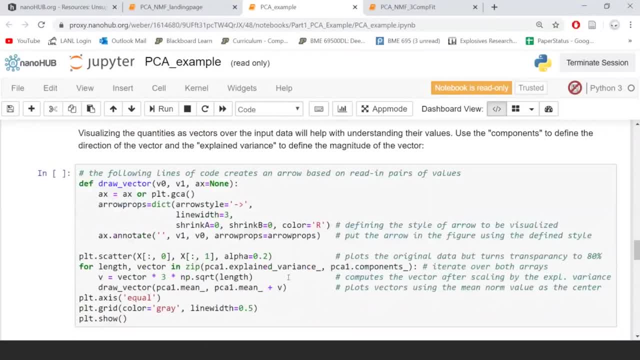 variables, But of course, as I stated, you can do PCA on n dimensions. So we're going to go over this toy example, where we're only going to address two input variables, But of course, as I stated, you can do PCA on n dimensions. 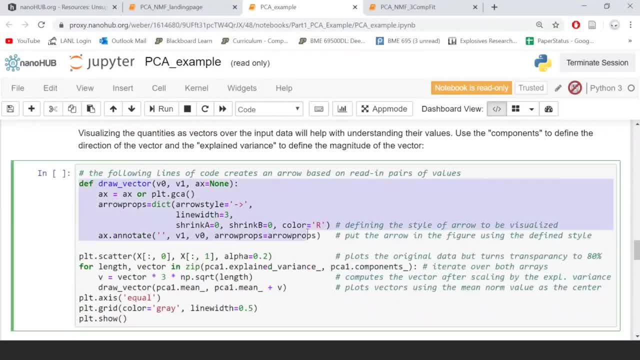 So we're going to go over this toy example where we're only going to address two input variables. But of course, as I stated, you can do PCA on n dimensions. So we're going to go over this toy example where we're only going to address two input. 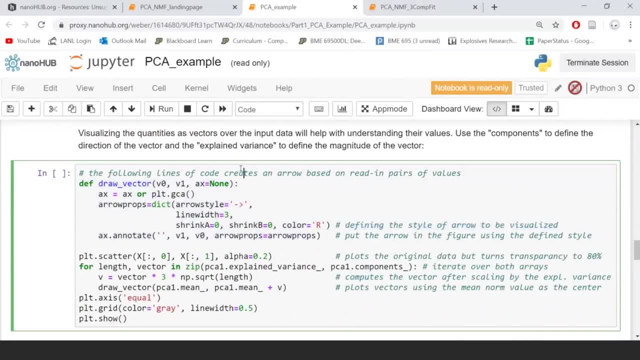 variables, But of course, as I stated, you can do PCA on n dimensions. So we're going to go over this toy example, where we're only going to address two input variables, But of course, as I stated, you can do PCA on n dimensions. 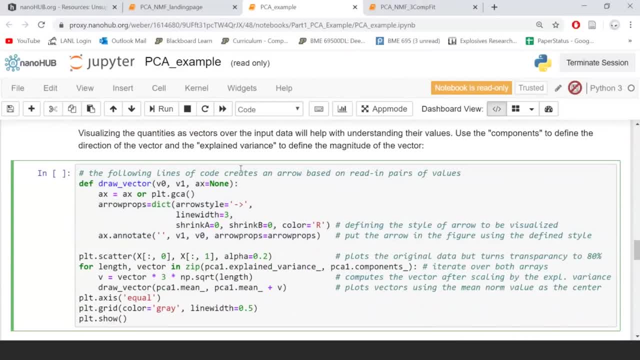 So we're going to go over this toy example where we're only going to address two input variables. But of course, as I stated, you can do PCA on n dimensions. So we're going to go over this toy example where we're only going to address two input. 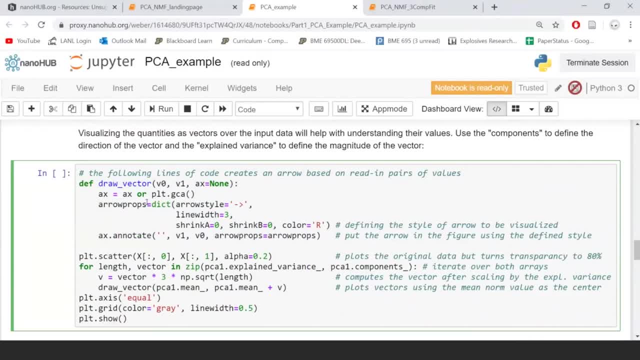 variables, But of course, as I stated, you can do PCA on n dimensions. So we're going to go over this toy example, where we're only going to address two input variables, But of course, as I stated, you can do PCA on n dimensions. 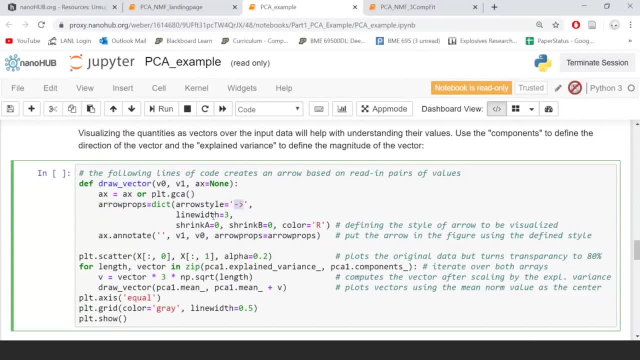 So we're going to go over this toy example where we're only going to address two input variables. But of course, as I stated, you can do PCA on n dimensions. So we're going to go over this toy example where we're only going to address two input. 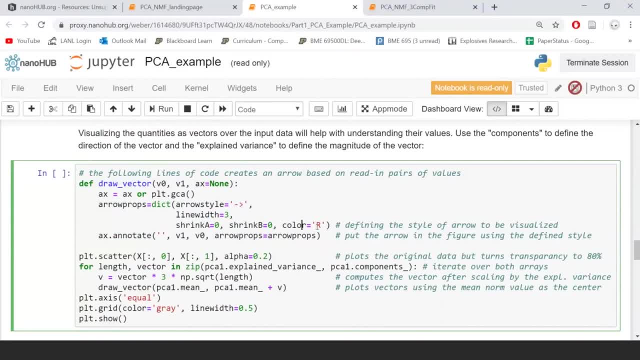 variables, But of course, as I stated, you can do PCA on n dimensions. So we're going to go over this toy example, where we're only going to address two input variables, But of course, as I stated, you can do PCA on n dimensions. 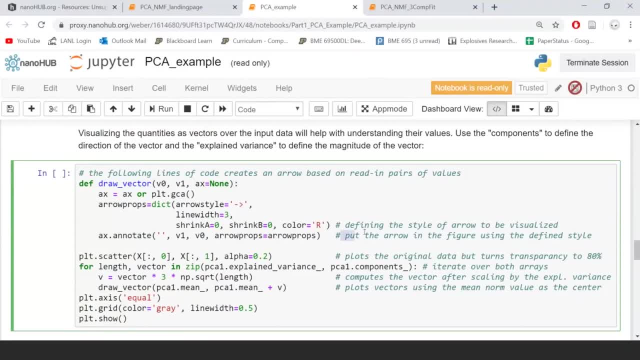 So we're going to go over this toy example where we're only going to address two input variables. But of course, as I stated, you can do PCA on n dimensions. So we're going to go over this toy example where we're only going to address two input. 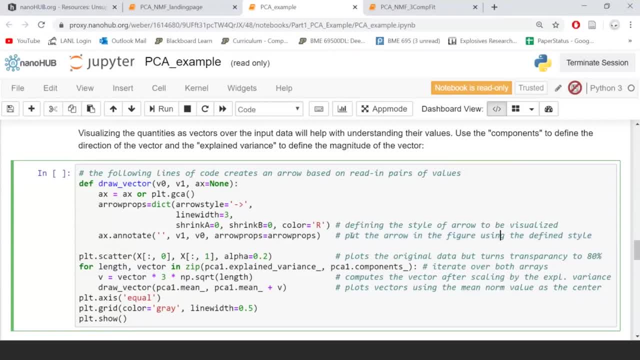 variables, But of course, as I stated, you can do PCA on n dimensions. So we're going to go over this toy example, where we're only going to address two input variables, But of course, as I stated, you can do PCA on n dimensions. 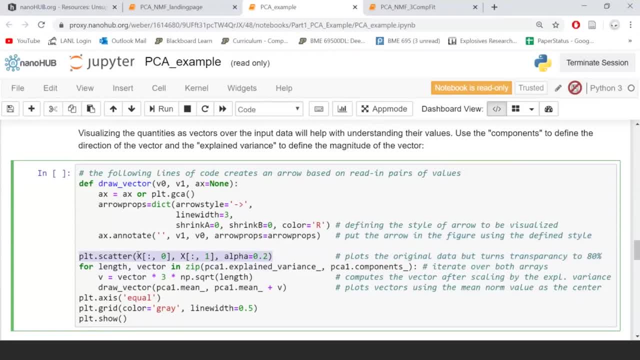 So we're going to go over this toy example where we're only going to address two input variables. But of course, as I stated, you can do PCA on n dimensions. So we're going to go over this toy example where we're only going to address two input. 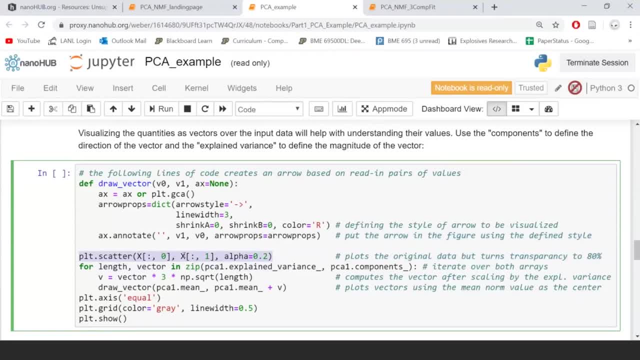 variables, But of course, as I stated, you can do PCA on n dimensions. So we're going to go over this toy example, where we're only going to address two input variables, But of course, as I stated, you can do PCA on n dimensions. 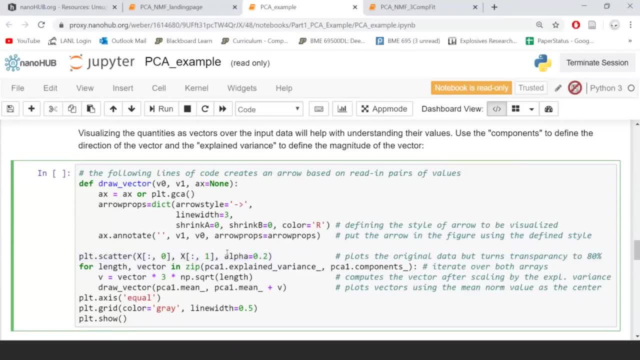 So we're going to go over this toy example where we're only going to address two input variables. But of course, as I stated, you can do PCA on n dimensions. So we're going to go over this toy example where we're only going to address two input. 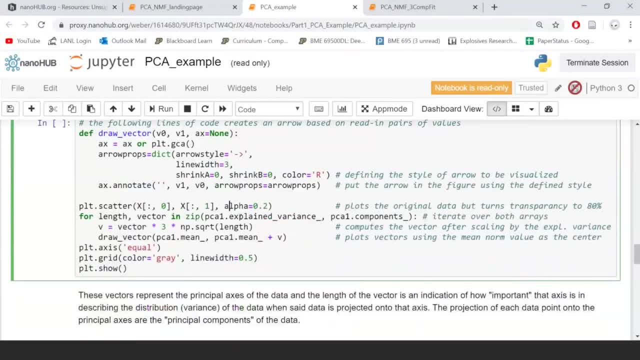 variables, But of course, as I stated, you can do PCA on n dimensions. So we're going to go over this toy example, where we're only going to address two input variables, But of course, as I stated, you can do PCA on n dimensions. 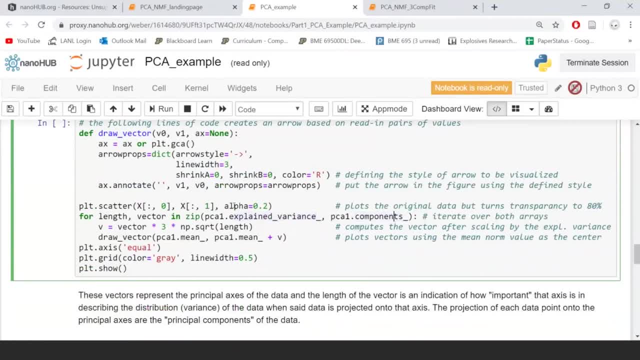 So we're going to go over this toy example where we're only going to address two input variables. But of course, as I stated, you can do PCA on n dimensions. So we're going to go over this toy example where we're only going to address two input. 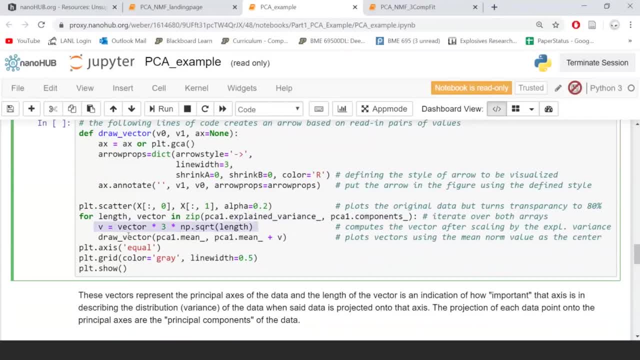 variables, But of course, as I stated, you can do PCA on n dimensions. So we're going to go over this toy example, where we're only going to address two input variables, But of course, as I stated, you can do PCA on n dimensions. 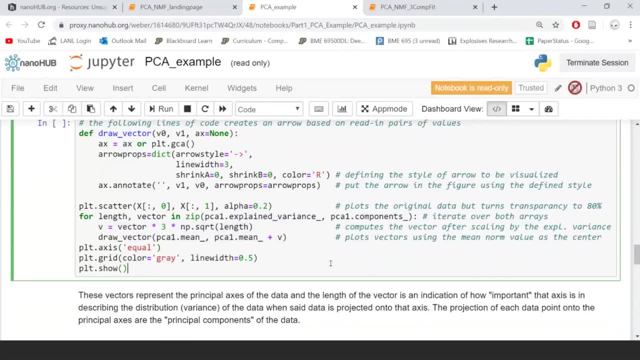 So we're going to go over this toy example where we're only going to address two input variables. But of course, as I stated, you can do PCA on n dimensions. So we're going to go over this toy example where we're only going to address two input. 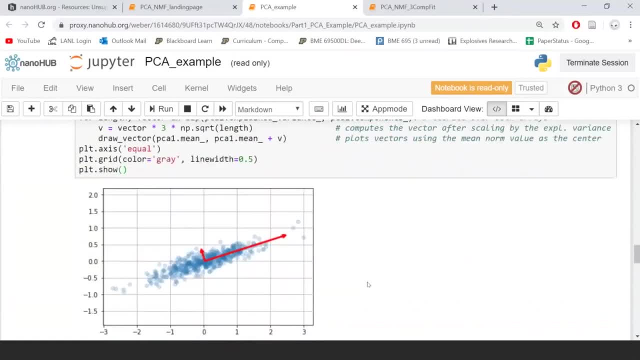 variables, But of course, as I stated, you can do PCA on n dimensions. So we're going to go over this toy example, where we're only going to address two input variables, But of course, as I stated, you can do PCA on n dimensions. 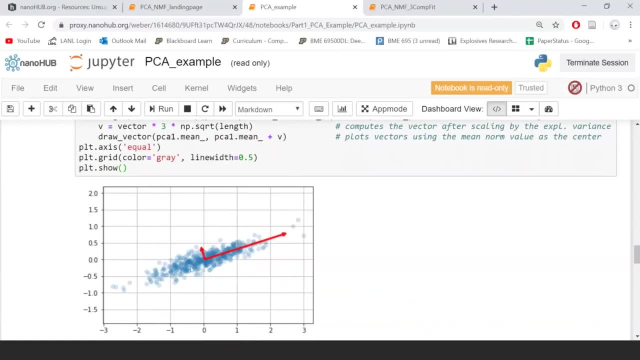 So we're going to go over this toy example where we're only going to address two input variables. But of course, as I stated, you can do PCA on n dimensions. So we're going to go over this toy example where we're only going to address two input. 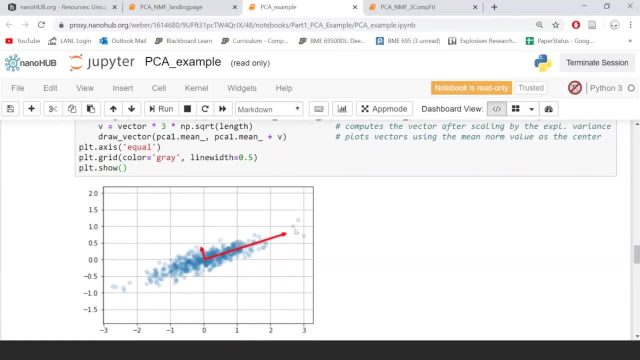 variables, But of course, as I stated, you can do PCA on n dimensions. So we're going to go over this toy example, where we're only going to address two input variables, But of course, as I stated, you can do PCA on n dimensions. 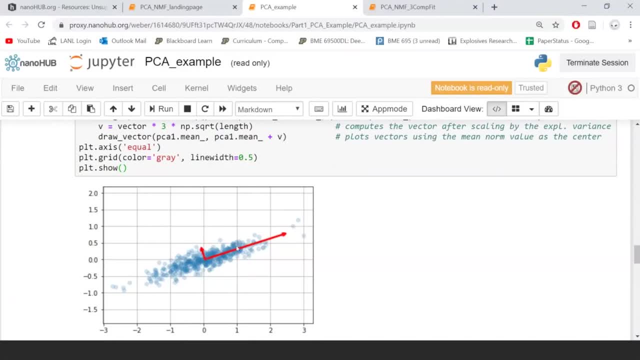 So we're going to go over this toy example where we're only going to address two input variables. But of course, as I stated, you can do PCA on n dimensions. So we're going to go over this toy example where we're only going to address two input. 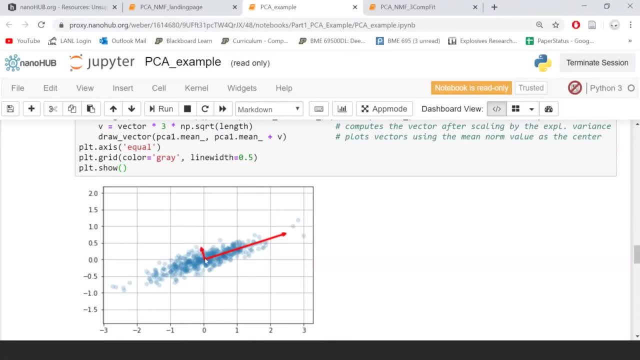 variables, But of course, as I stated, you can do PCA on n dimensions. So we're going to go over this toy example, where we're only going to address two input variables, But of course, as I stated, you can do PCA on n dimensions. 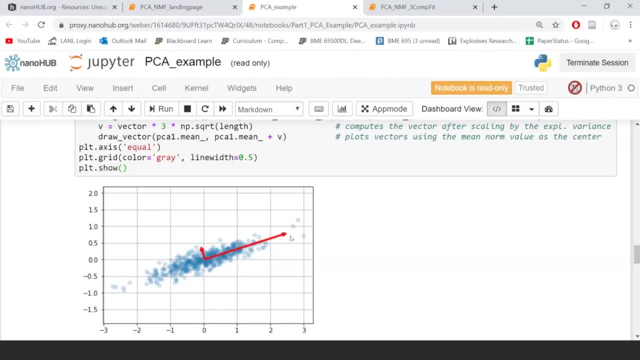 So we're going to go over this toy example where we're only going to address two input variables. But of course, as I stated, you can do PCA on n dimensions. So we're going to go over this toy example where we're only going to address two input. 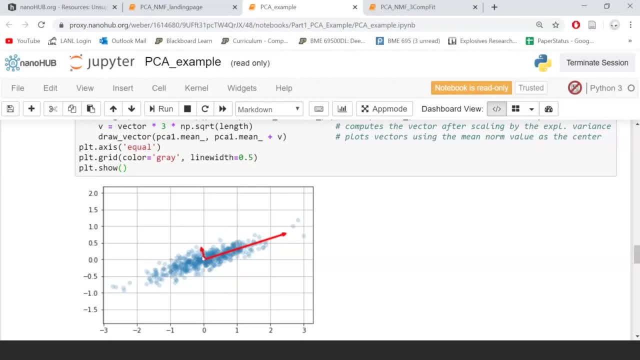 variables, But of course, as I stated, you can do PCA on n dimensions. So we're going to go over this toy example, where we're only going to address two input variables, But of course, as I stated, you can do PCA on n dimensions. 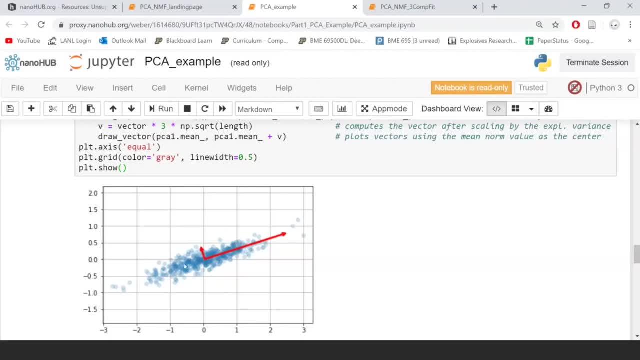 So we're going to go over this toy example where we're only going to address two input variables. But of course, as I stated, you can do PCA on n dimensions. So we're going to go over this toy example where we're only going to address two input. 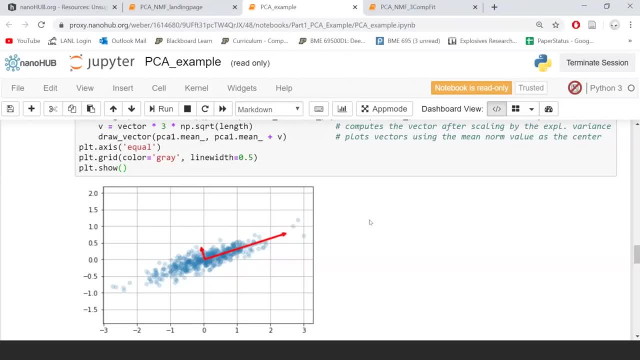 variables, But of course, as I stated, you can do PCA on n dimensions. So we're going to go over this toy example, where we're only going to address two input variables, But of course, as I stated, you can do PCA on n dimensions. 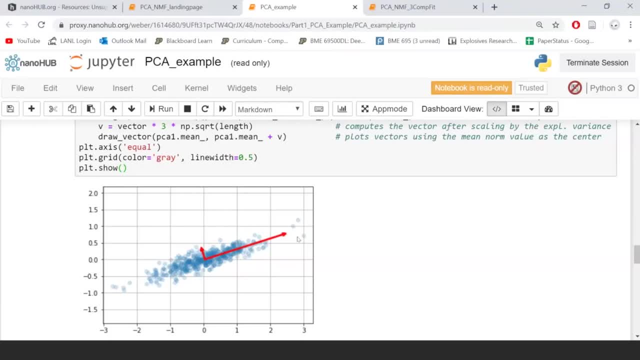 So we're going to go over this toy example where we're only going to address two input variables. But of course, as I stated, you can do PCA on n dimensions. So we're going to go over this toy example where we're only going to address two input. 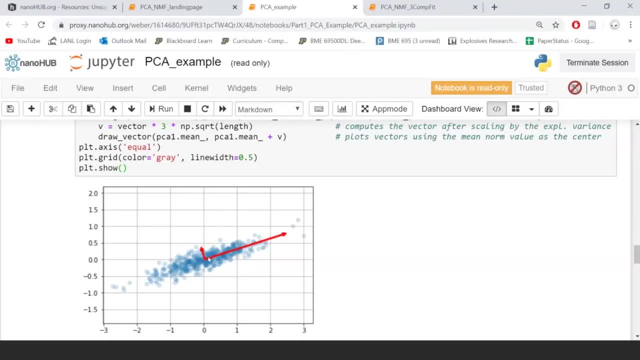 variables, But of course, as I stated, you can do PCA on n dimensions. So we're going to go over this toy example, where we're only going to address two input variables, But of course, as I stated, you can do PCA on n dimensions. 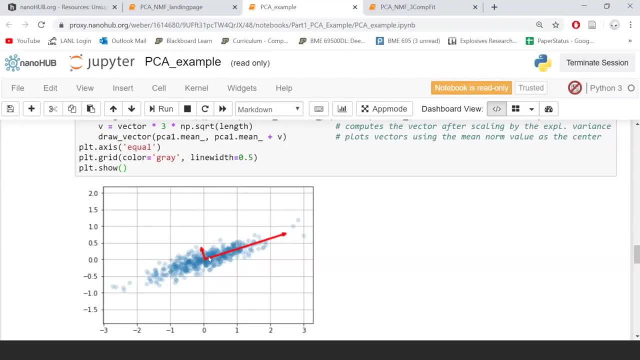 So we're going to go over this toy example where we're only going to address two input variables. But of course, as I stated, you can do PCA on n dimensions. So we're going to go over this toy example where we're only going to address two input. 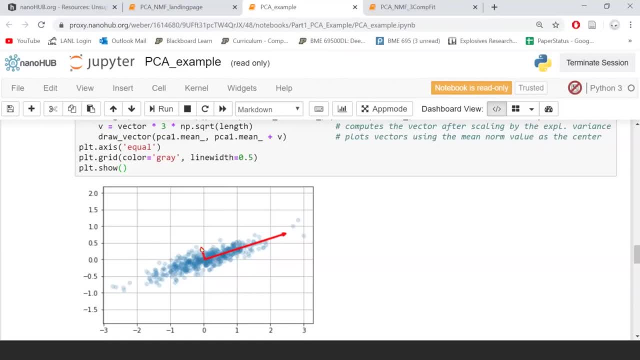 variables, But of course, as I stated, you can do PCA on n dimensions. So we're going to go over this toy example, where we're only going to address two input variables, But of course, as I stated, you can do PCA on n dimensions. 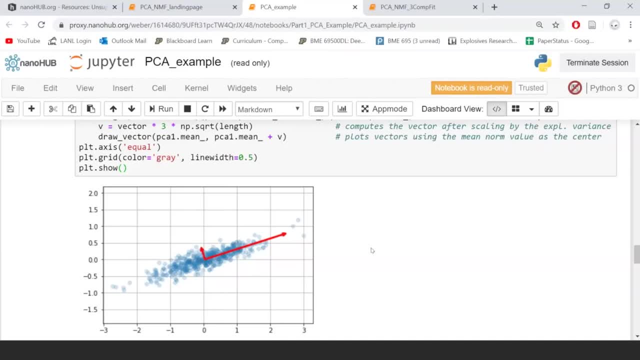 So we're going to go over this toy example where we're only going to address two input variables. But of course, as I stated, you can do PCA on n dimensions. So we're going to go over this toy example where we're only going to address two input. 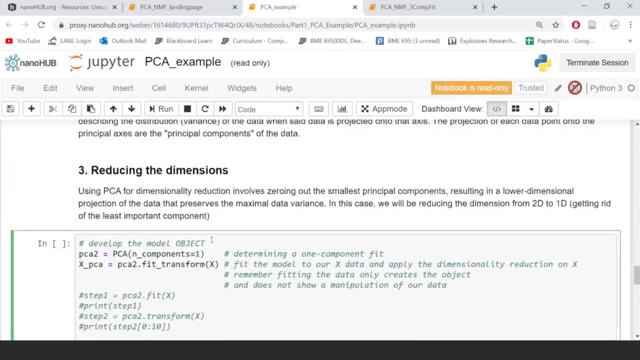 variables, But of course, as I stated, you can do PCA on n dimensions. So we're going to go over this toy example, where we're only going to address two input variables, But of course, as I stated, you can do PCA on n dimensions. 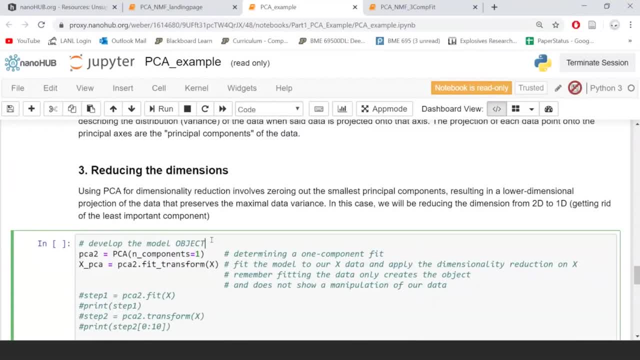 So we're going to go over this toy example where we're only going to address two input variables. But of course, as I stated, you can do PCA on n dimensions. So we're going to go over this toy example where we're only going to address two input. 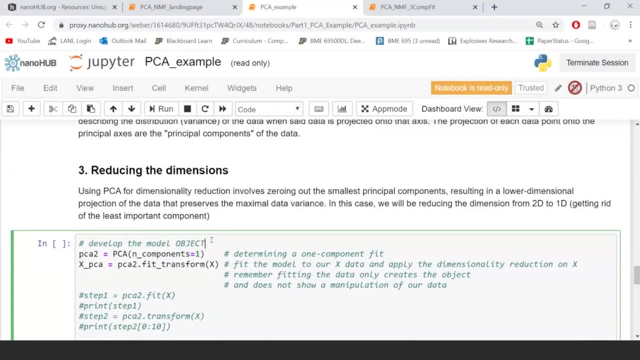 variables, But of course, as I stated, you can do PCA on n dimensions. So we're going to go over this toy example, where we're only going to address two input variables, But of course, as I stated, you can do PCA on n dimensions. 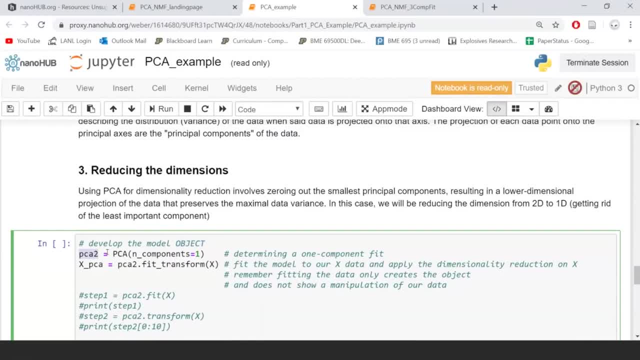 So we're going to go over this toy example where we're only going to address two input variables. But of course, as I stated, you can do PCA on n dimensions. So we're going to go over this toy example where we're only going to address two input. 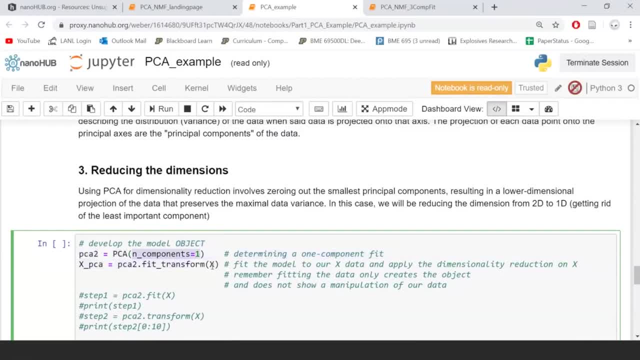 variables, But of course, as I stated, you can do PCA on n dimensions. So we're going to go over this toy example, where we're only going to address two input variables, But of course, as I stated, you can do PCA on n dimensions. 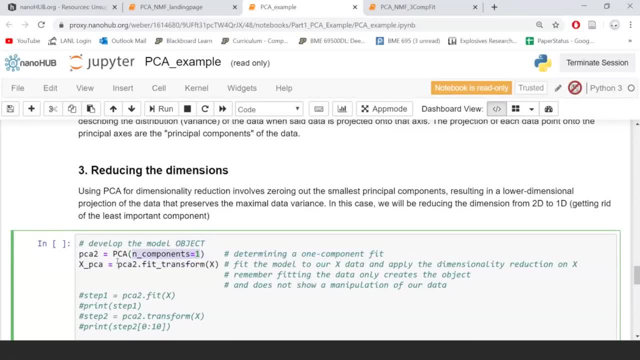 So we're going to go over this toy example where we're only going to address two input variables. But of course, as I stated, you can do PCA on n dimensions. So we're going to go over this toy example where we're only going to address two input. 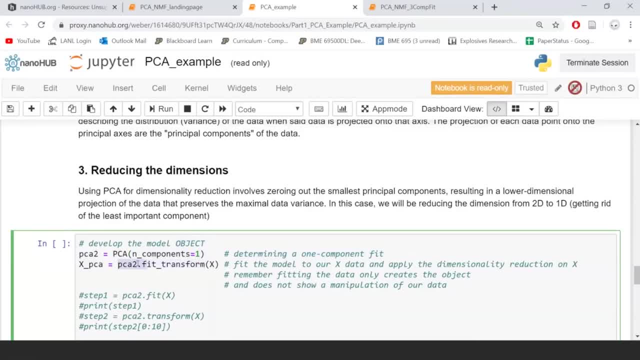 variables, But of course, as I stated, you can do PCA on n dimensions. So we're going to go over this toy example, where we're only going to address two input variables, But of course, as I stated, you can do PCA on n dimensions. 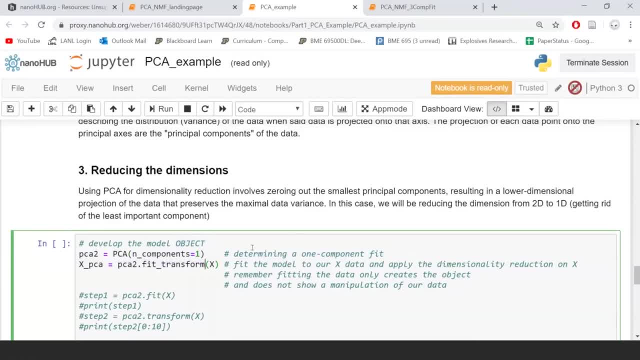 So we're going to go over this toy example where we're only going to address two input variables. But of course, as I stated, you can do PCA on n dimensions. So we're going to go over this toy example where we're only going to address two input. 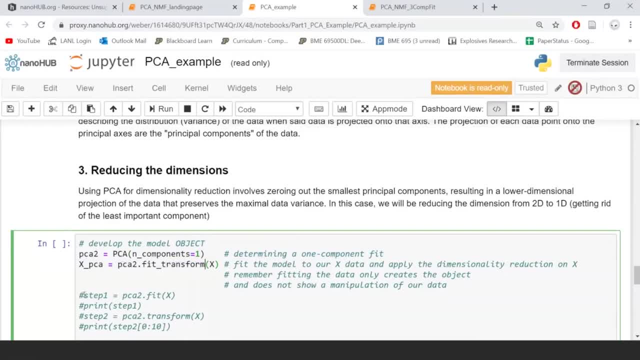 variables, But of course, as I stated, you can do PCA on n dimensions. So we're going to go over this toy example, where we're only going to address two input variables, But of course, as I stated, you can do PCA on n dimensions. 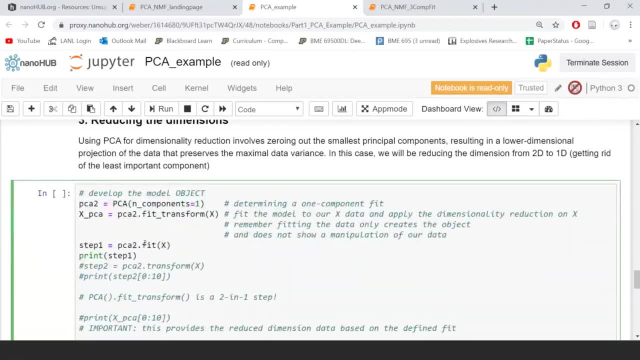 So we're going to go over this toy example where we're only going to address two input variables. But of course, as I stated, you can do PCA on n dimensions. So we're going to go over this toy example where we're only going to address two input. 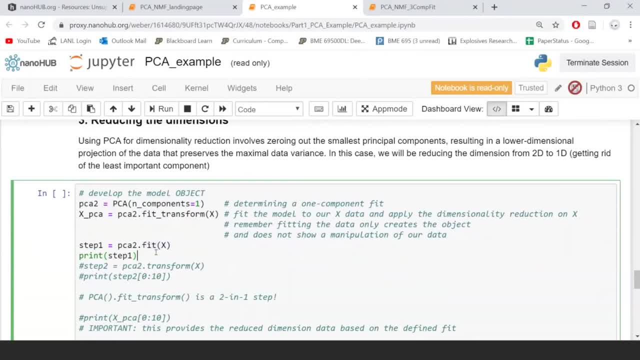 variables, But of course, as I stated, you can do PCA on n dimensions. So we're going to go over this toy example, where we're only going to address two input variables, But of course, as I stated, you can do PCA on n dimensions. 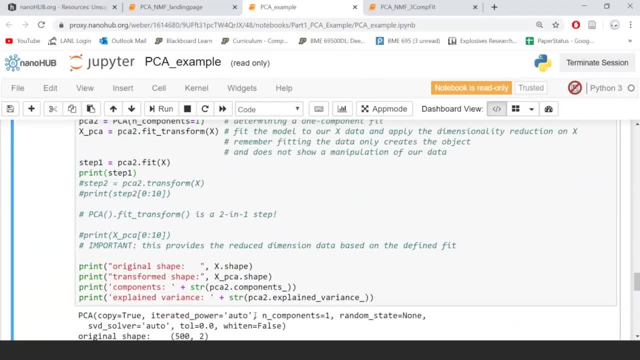 So we're going to go over this toy example where we're only going to address two input variables. But of course, as I stated, you can do PCA on n dimensions. So we're going to go over this toy example where we're only going to address two input. 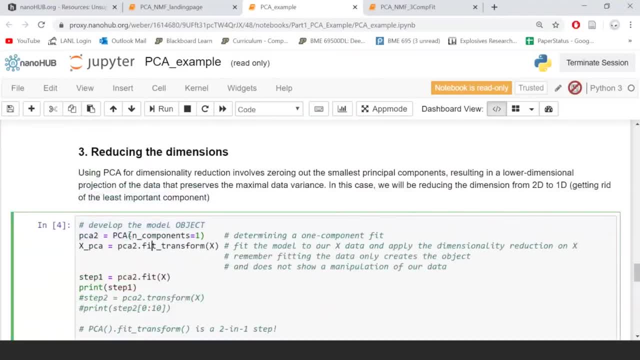 variables, But of course, as I stated, you can do PCA on n dimensions. So we're going to go over this toy example, where we're only going to address two input variables, But of course, as I stated, you can do PCA on n dimensions. 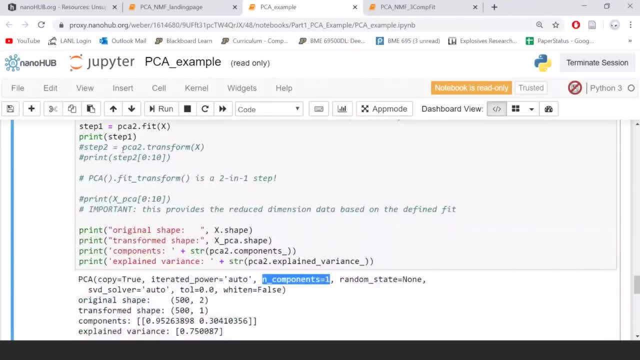 So we're going to go over this toy example where we're only going to address two input variables. But of course, as I stated, you can do PCA on n dimensions. So we're going to go over this toy example where we're only going to address two input. 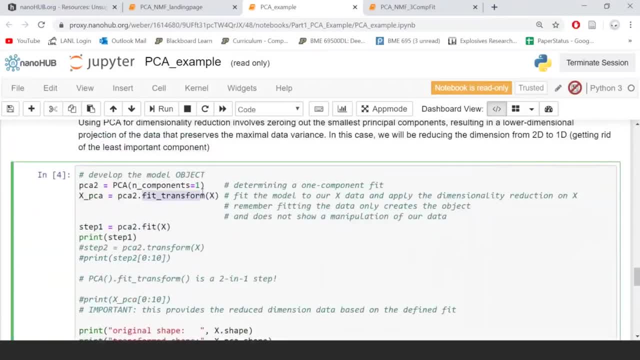 variables, But of course, as I stated, you can do PCA on n dimensions. So we're going to go over this toy example, where we're only going to address two input variables, But of course, as I stated, you can do PCA on n dimensions. 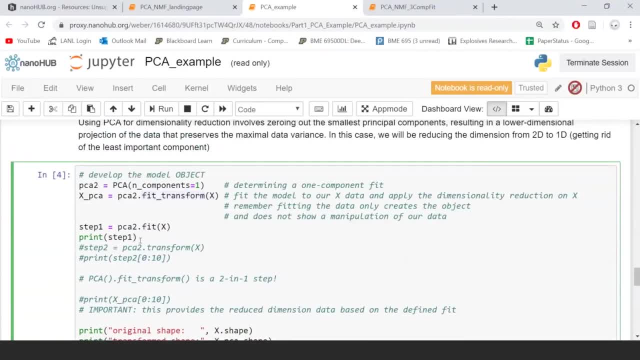 So we're going to go over this toy example where we're only going to address two input variables. But of course, as I stated, you can do PCA on n dimensions. So we're going to go over this toy example where we're only going to address two input. 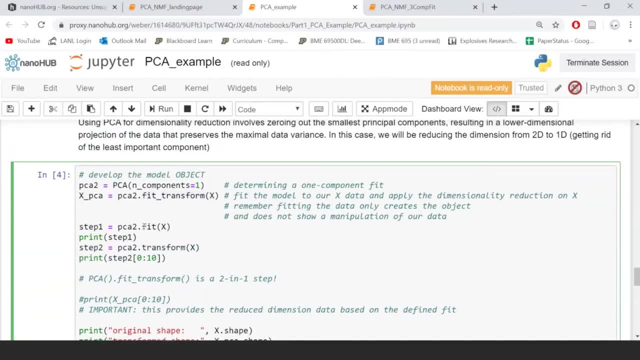 variables, But of course, as I stated, you can do PCA on n dimensions. So we're going to go over this toy example, where we're only going to address two input variables, But of course, as I stated, you can do PCA on n dimensions. 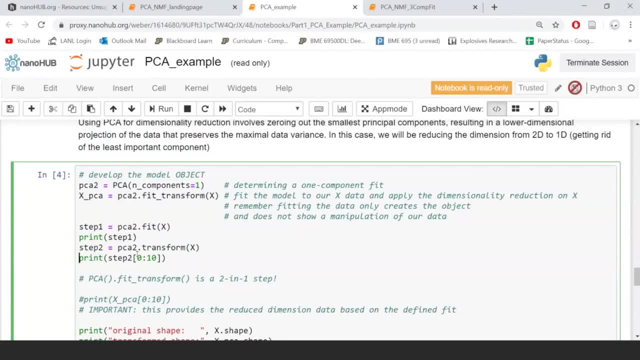 So we're going to go over this toy example where we're only going to address two input variables. But of course, as I stated, you can do PCA on n dimensions. So we're going to go over this toy example where we're only going to address two input. 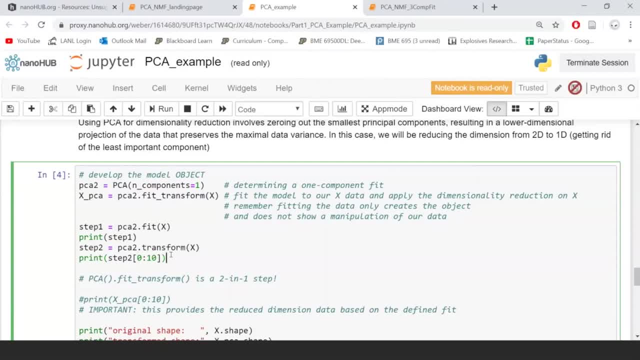 variables, But of course, as I stated, you can do PCA on n dimensions. So we're going to go over this toy example, where we're only going to address two input variables, But of course, as I stated, you can do PCA on n dimensions. 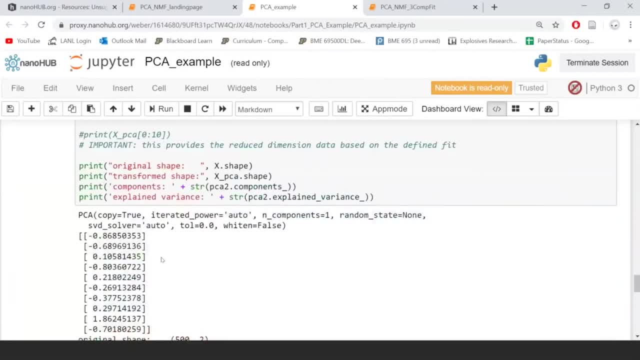 So we're going to go over this toy example where we're only going to address two input variables. But of course, as I stated, you can do PCA on n dimensions. So we're going to go over this toy example where we're only going to address two input. 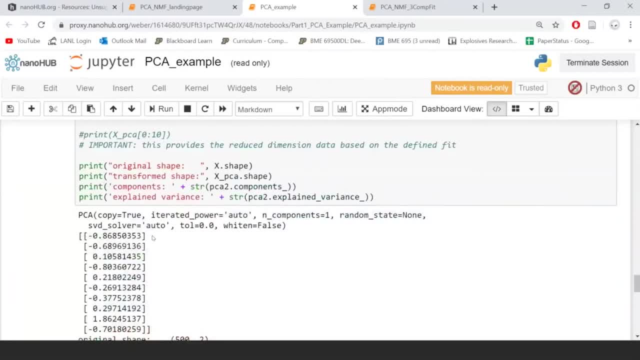 variables, But of course, as I stated, you can do PCA on n dimensions. So we're going to go over this toy example, where we're only going to address two input variables, But of course, as I stated, you can do PCA on n dimensions. 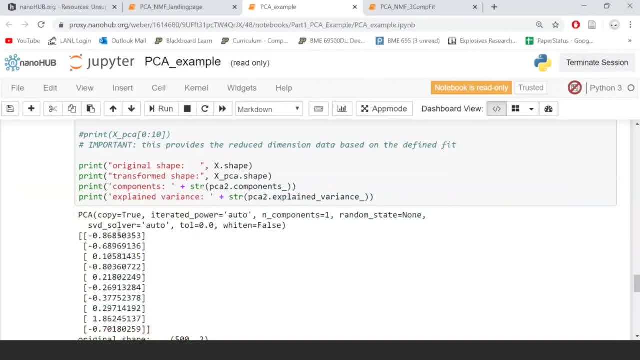 So we're going to go over this toy example where we're only going to address two input variables. But of course, as I stated, you can do PCA on n dimensions. So we're going to go over this toy example where we're only going to address two input. 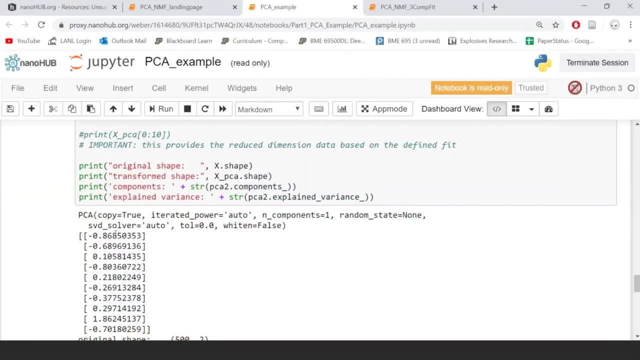 variables, But of course, as I stated, you can do PCA on n dimensions. So we're going to go over this toy example, where we're only going to address two input variables, But of course, as I stated, you can do PCA on n dimensions. 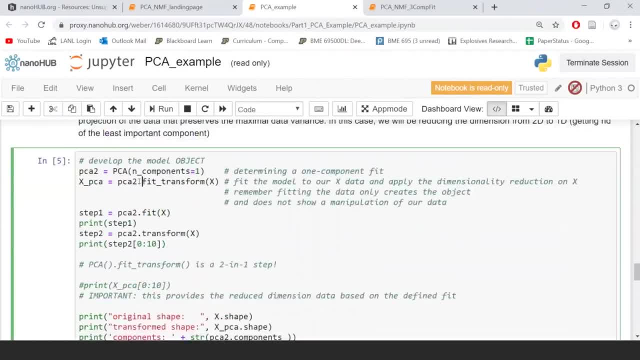 So we're going to go over this toy example where we're only going to address two input variables. But of course, as I stated, you can do PCA on n dimensions. So we're going to go over this toy example where we're only going to address two input. 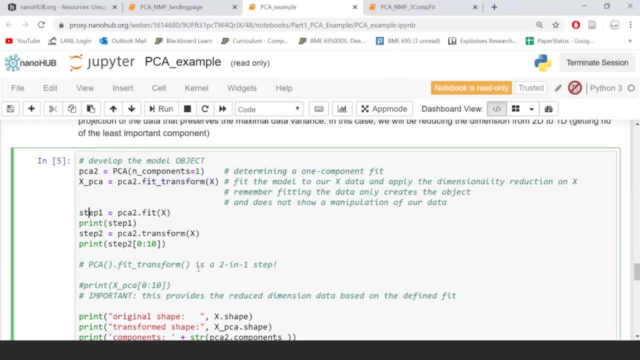 variables, But of course, as I stated, you can do PCA on n dimensions. So we're going to go over this toy example, where we're only going to address two input variables, But of course, as I stated, you can do PCA on n dimensions. 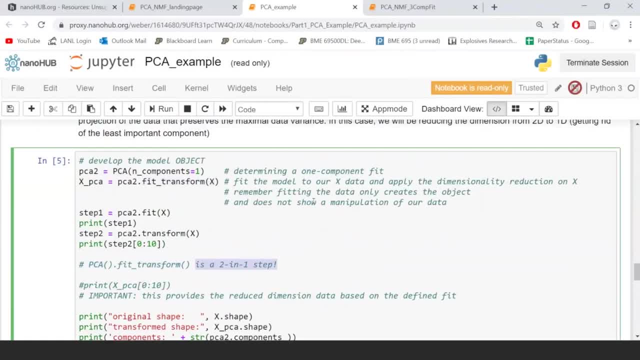 So we're going to go over this toy example where we're only going to address two input variables. But of course, as I stated, you can do PCA on n dimensions. So we're going to go over this toy example where we're only going to address two input. 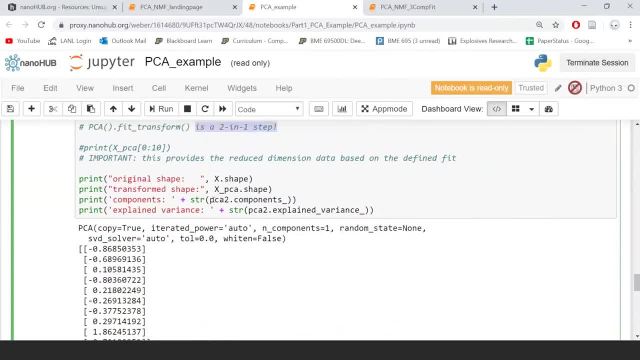 variables, But of course, as I stated, you can do PCA on n dimensions. So we're going to go over this toy example, where we're only going to address two input variables, But of course, as I stated, you can do PCA on n dimensions. 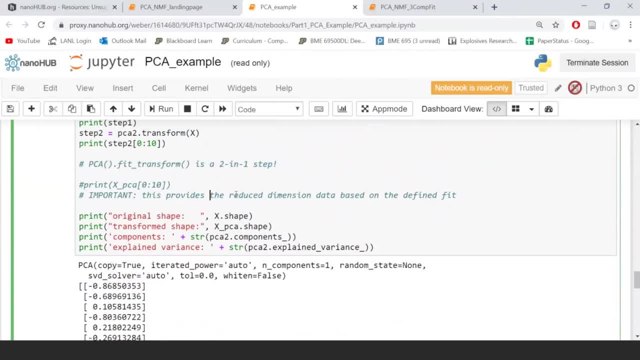 So we're going to go over this toy example where we're only going to address two input variables. But of course, as I stated, you can do PCA on n dimensions. So we're going to go over this toy example where we're only going to address two input. 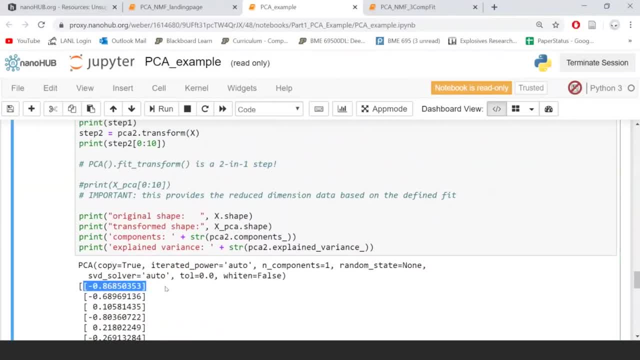 variables, But of course, as I stated, you can do PCA on n dimensions. So we're going to go over this toy example, where we're only going to address two input variables, But of course, as I stated, you can do PCA on n dimensions. 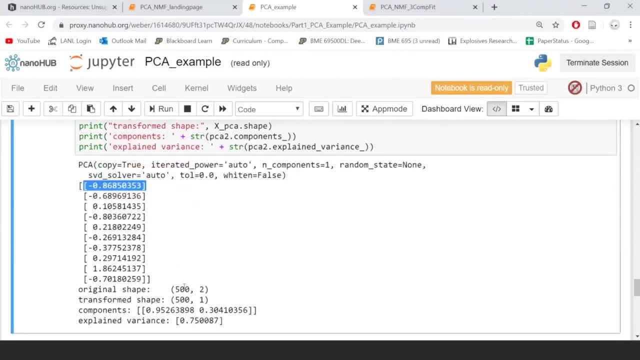 So we're going to go over this toy example where we're only going to address two input variables. But of course, as I stated, you can do PCA on n dimensions. So we're going to go over this toy example where we're only going to address two input. 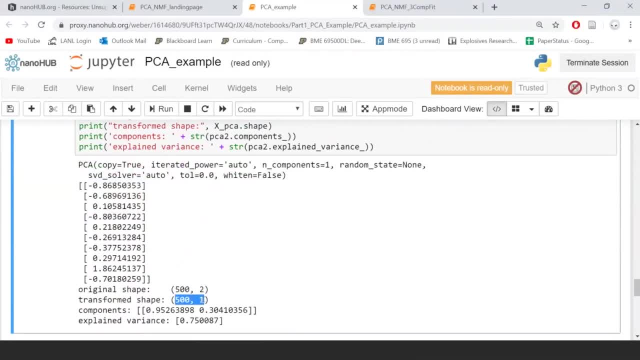 variables, But of course, as I stated, you can do PCA on n dimensions. So we're going to go over this toy example, where we're only going to address two input variables, But of course, as I stated, you can do PCA on n dimensions. 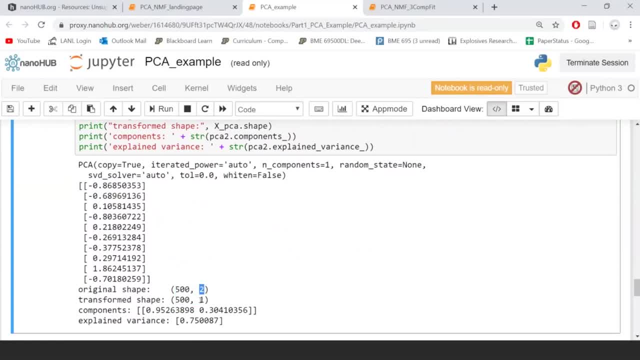 So we're going to go over this toy example where we're only going to address two input variables. But of course, as I stated, you can do PCA on n dimensions. So we're going to go over this toy example where we're only going to address two input. 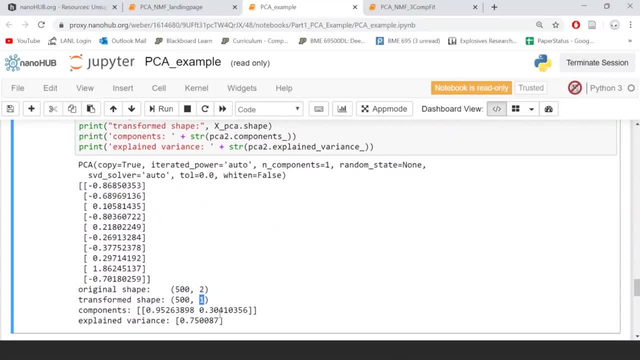 variables, But of course, as I stated, you can do PCA on n dimensions. So we're going to go over this toy example, where we're only going to address two input variables, But of course, as I stated, you can do PCA on n dimensions. 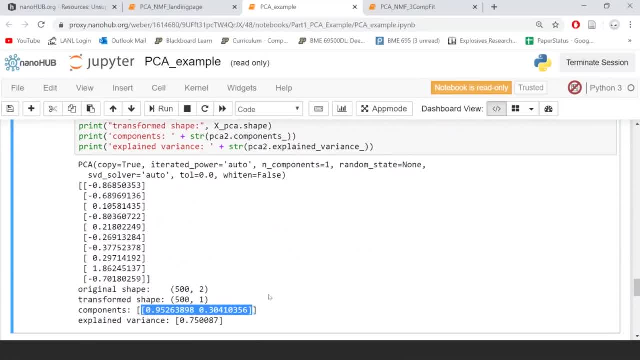 So we're going to go over this toy example where we're only going to address two input variables. But of course, as I stated, you can do PCA on n dimensions. So we're going to go over this toy example where we're only going to address two input. 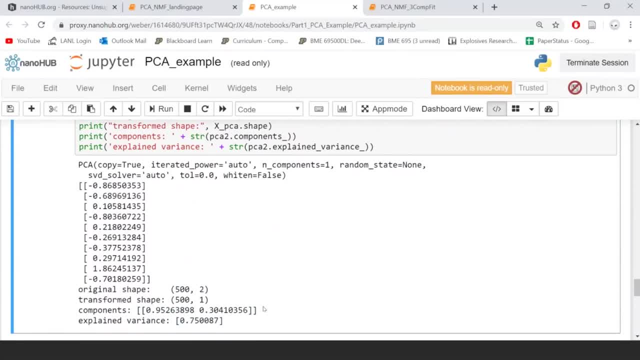 variables, But of course, as I stated, you can do PCA on n dimensions. So we're going to go over this toy example, where we're only going to address two input variables, But of course, as I stated, you can do PCA on n dimensions. 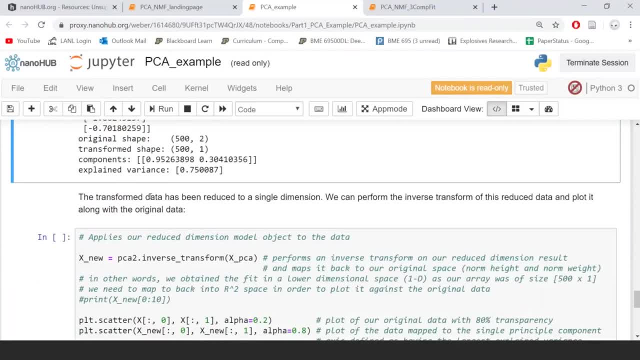 So we're going to go over this toy example where we're only going to address two input variables. But of course, as I stated, you can do PCA on n dimensions. So we're going to go over this toy example where we're only going to address two input. 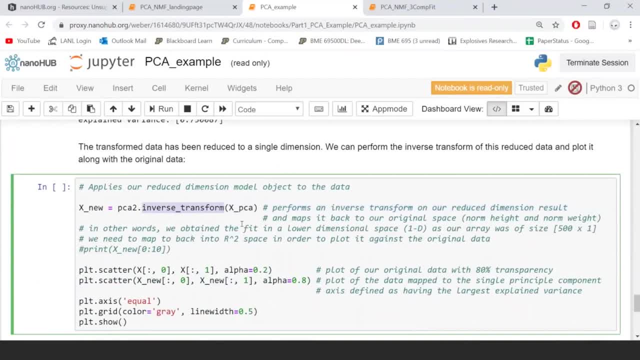 variables, But of course, as I stated, you can do PCA on n dimensions. So we're going to go over this toy example, where we're only going to address two input variables, But of course, as I stated, you can do PCA on n dimensions. 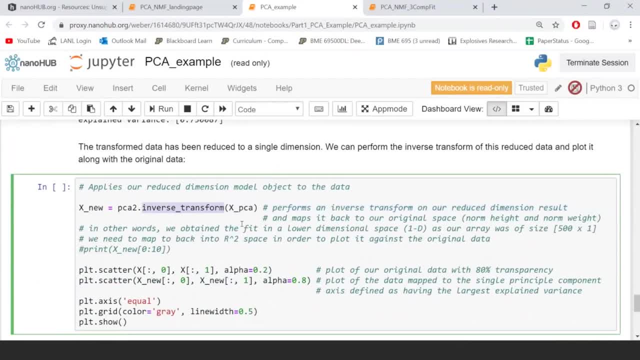 So we're going to go over this toy example where we're only going to address two input variables. But of course, as I stated, you can do PCA on n dimensions. So we're going to go over this toy example where we're only going to address two input. 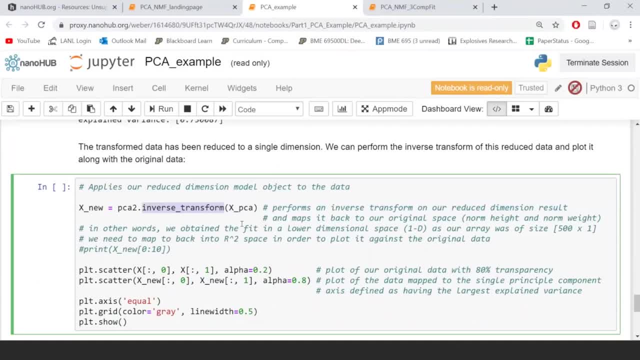 variables, But of course, as I stated, you can do PCA on n dimensions. So we're going to go over this toy example, where we're only going to address two input variables, But of course, as I stated, you can do PCA on n dimensions. 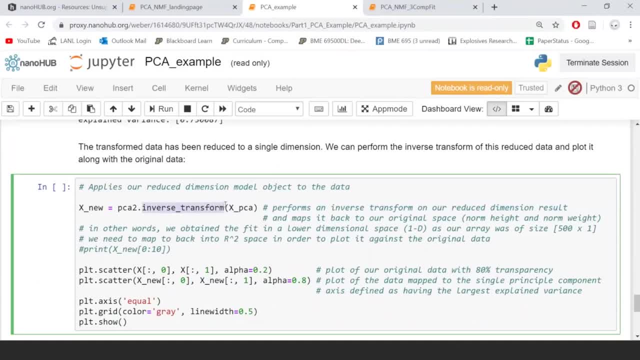 So we're going to go over this toy example where we're only going to address two input variables. But of course, as I stated, you can do PCA on n dimensions. So we're going to go over this toy example where we're only going to address two input. 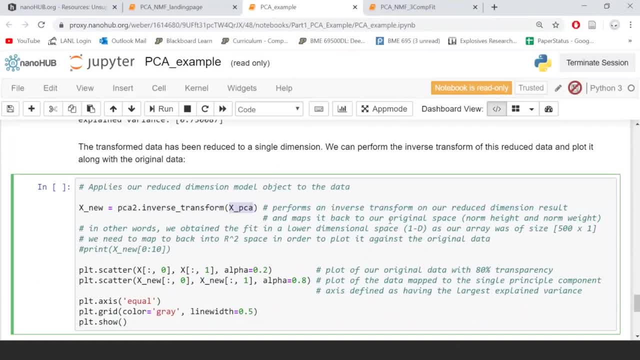 variables, But of course, as I stated, you can do PCA on n dimensions. So we're going to go over this toy example, where we're only going to address two input variables, But of course, as I stated, you can do PCA on n dimensions. 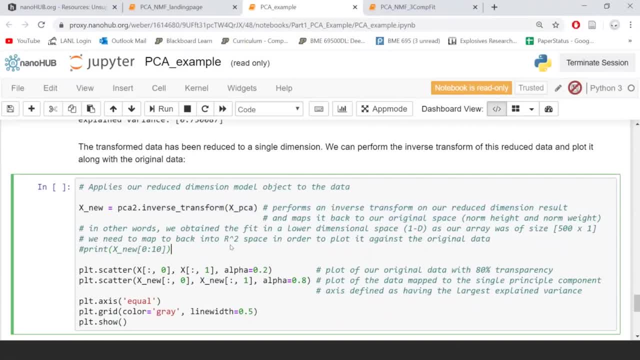 So we're going to go over this toy example where we're only going to address two input variables. But of course, as I stated, you can do PCA on n dimensions. So we're going to go over this toy example where we're only going to address two input. 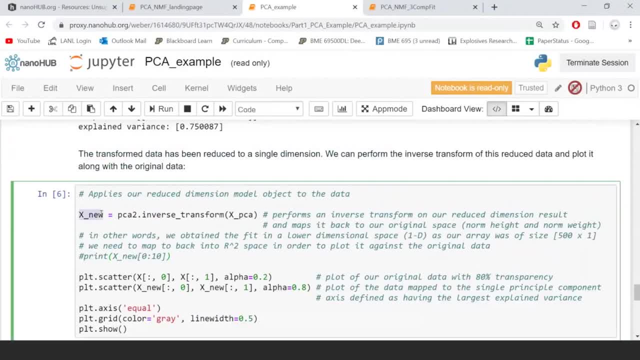 variables, But of course, as I stated, you can do PCA on n dimensions. So we're going to go over this toy example, where we're only going to address two input variables, But of course, as I stated, you can do PCA on n dimensions. 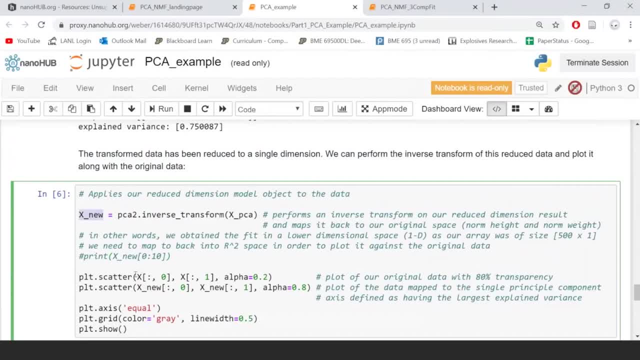 So we're going to go over this toy example where we're only going to address two input variables. But of course, as I stated, you can do PCA on n dimensions. So we're going to go over this toy example where we're only going to address two input. 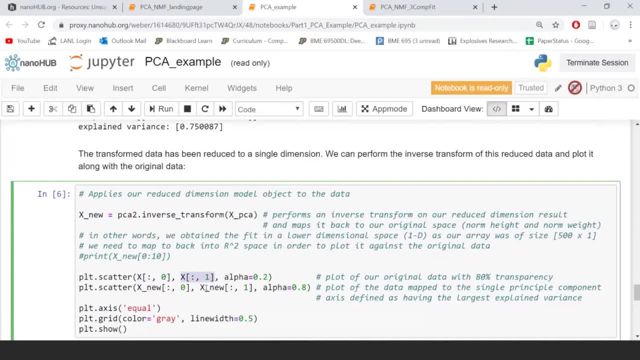 variables, But of course, as I stated, you can do PCA on n dimensions. So we're going to go over this toy example, where we're only going to address two input variables, But of course, as I stated, you can do PCA on n dimensions. 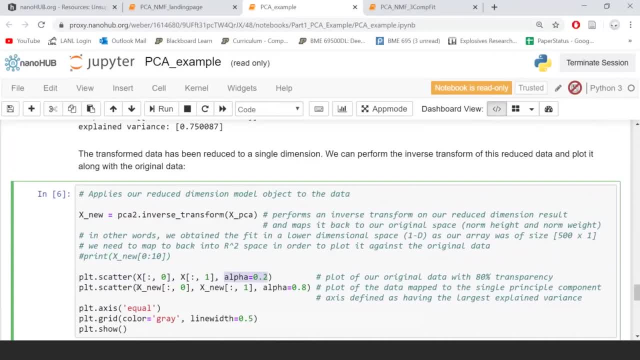 So we're going to go over this toy example where we're only going to address two input variables. But of course, as I stated, you can do PCA on n dimensions. So we're going to go over this toy example where we're only going to address two input. 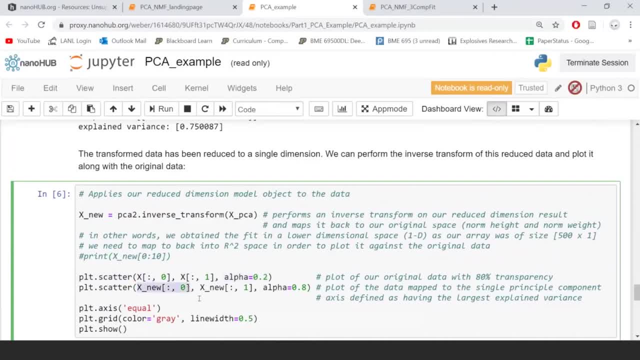 variables, But of course, as I stated, you can do PCA on n dimensions. So we're going to go over this toy example, where we're only going to address two input variables, But of course, as I stated, you can do PCA on n dimensions. 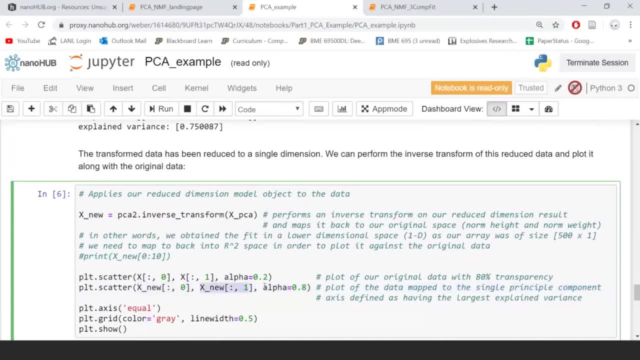 So we're going to go over this toy example where we're only going to address two input variables. But of course, as I stated, you can do PCA on n dimensions. So we're going to go over this toy example where we're only going to address two input. 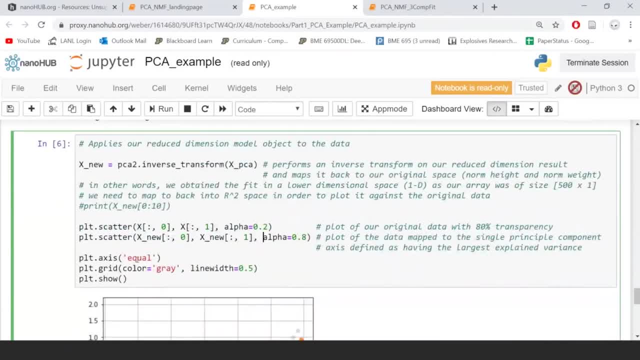 variables, But of course, as I stated, you can do PCA on n dimensions. So we're going to go over this toy example, where we're only going to address two input variables, But of course, as I stated, you can do PCA on n dimensions. 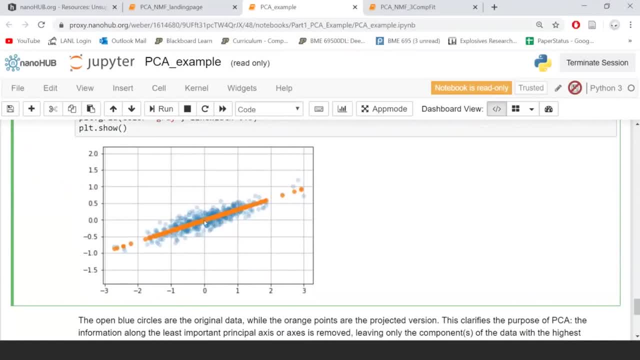 So we're going to go over this toy example where we're only going to address two input variables. But of course, as I stated, you can do PCA on n dimensions. So we're going to go over this toy example where we're only going to address two input. 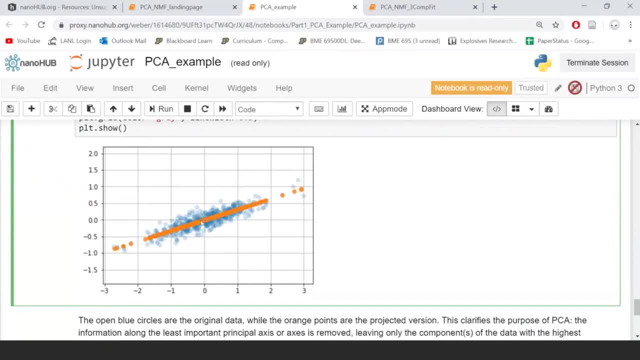 variables, But of course, as I stated, you can do PCA on n dimensions. So we're going to go over this toy example, where we're only going to address two input variables, But of course, as I stated, you can do PCA on n dimensions. 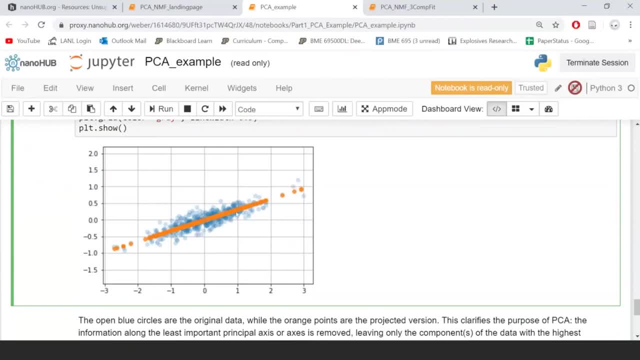 So we're going to go over this toy example where we're only going to address two input variables. But of course, as I stated, you can do PCA on n dimensions. So we're going to go over this toy example where we're only going to address two input. 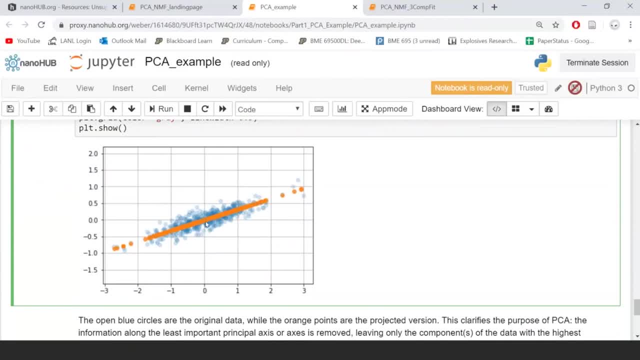 variables, But of course, as I stated, you can do PCA on n dimensions. So we're going to go over this toy example, where we're only going to address two input variables, But of course, as I stated, you can do PCA on n dimensions. 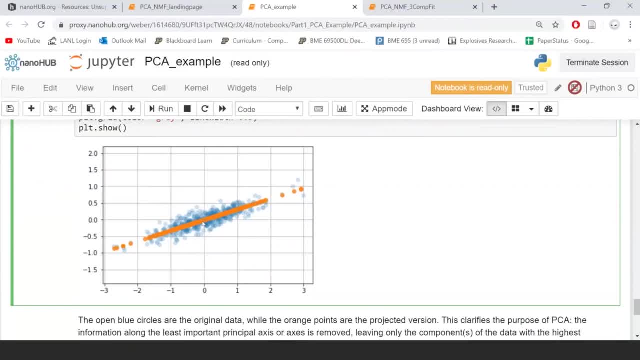 So we're going to go over this toy example where we're only going to address two input variables. But of course, as I stated, you can do PCA on n dimensions. So we're going to go over this toy example where we're only going to address two input. 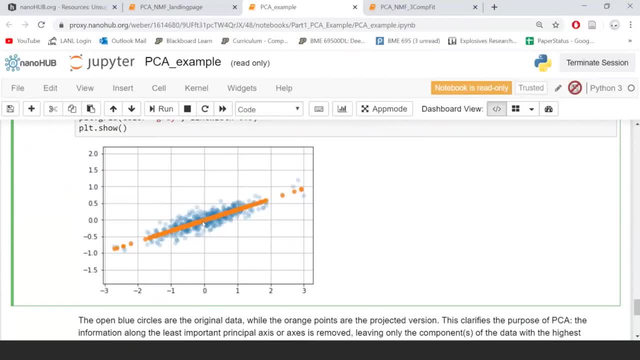 variables, But of course, as I stated, you can do PCA on n dimensions. So we're going to go over this toy example, where we're only going to address two input variables, But of course, as I stated, you can do PCA on n dimensions. 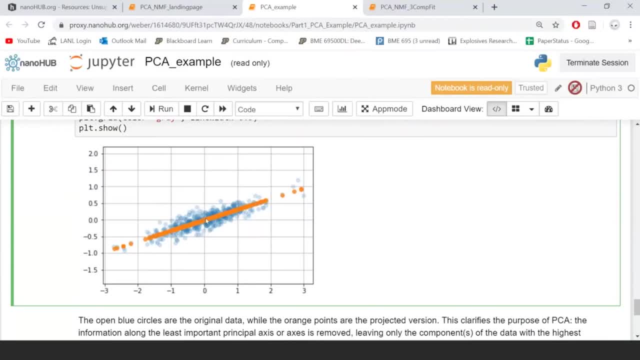 So we're going to go over this toy example where we're only going to address two input variables. But of course, as I stated, you can do PCA on n dimensions. So we're going to go over this toy example where we're only going to address two input. 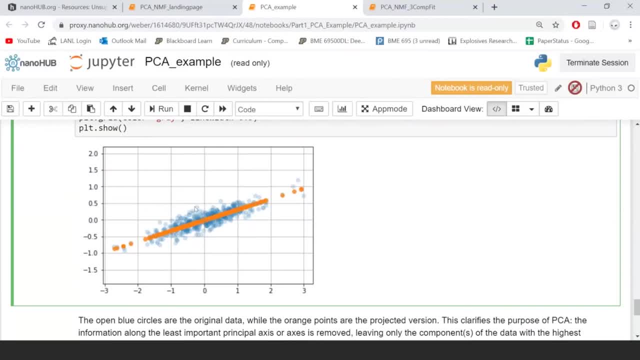 variables, But of course, as I stated, you can do PCA on n dimensions. So we're going to go over this toy example, where we're only going to address two input variables, But of course, as I stated, you can do PCA on n dimensions. 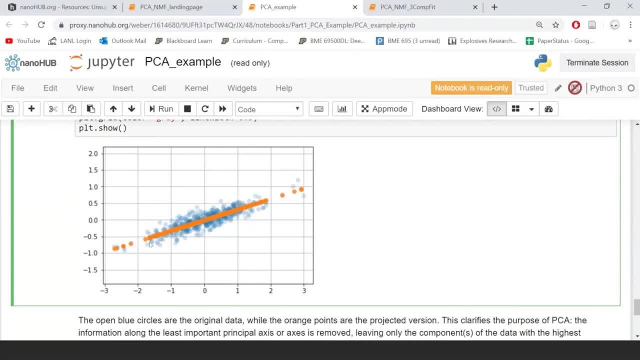 So we're going to go over this toy example where we're only going to address two input variables. But of course, as I stated, you can do PCA on n dimensions. So we're going to go over this toy example where we're only going to address two input. 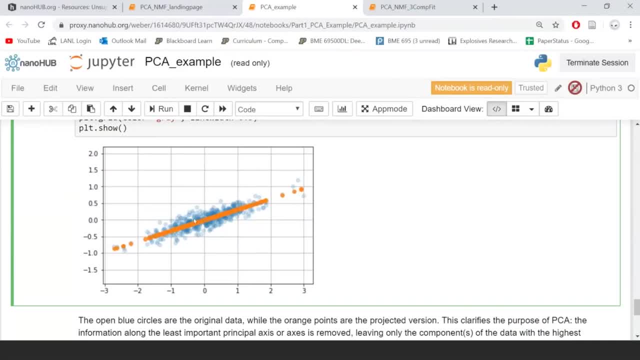 variables, But of course, as I stated, you can do PCA on n dimensions. So we're going to go over this toy example, where we're only going to address two input variables, But of course, as I stated, you can do PCA on n dimensions. 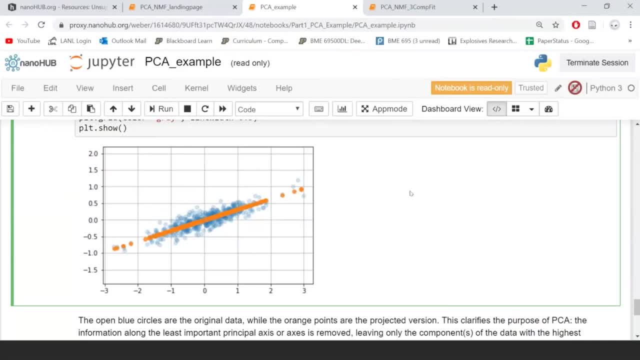 So we're going to go over this toy example where we're only going to address two input variables. But of course, as I stated, you can do PCA on n dimensions. So we're going to go over this toy example where we're only going to address two input. 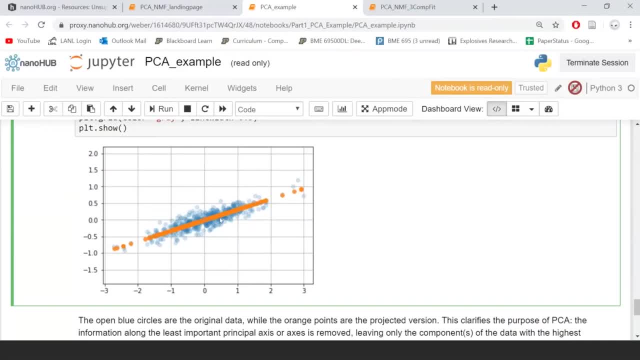 variables, But of course, as I stated, you can do PCA on n dimensions. So we're going to go over this toy example, where we're only going to address two input variables, But of course, as I stated, you can do PCA on n dimensions. 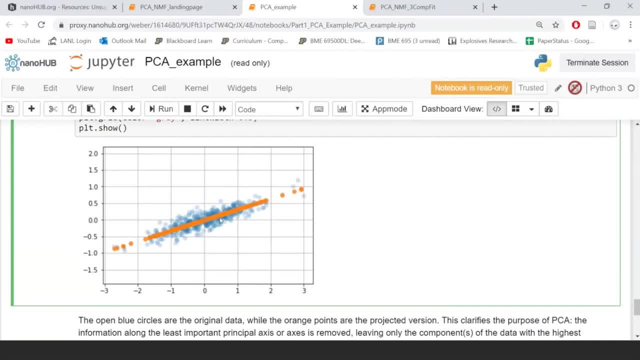 So we're going to go over this toy example where we're only going to address two input variables. But of course, as I stated, you can do PCA on n dimensions. So we're going to go over this toy example where we're only going to address two input. 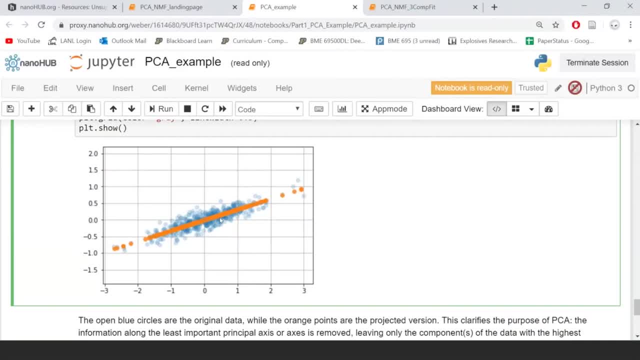 variables, But of course, as I stated, you can do PCA on n dimensions. So we're going to go over this toy example, where we're only going to address two input variables, But of course, as I stated, you can do PCA on n dimensions. 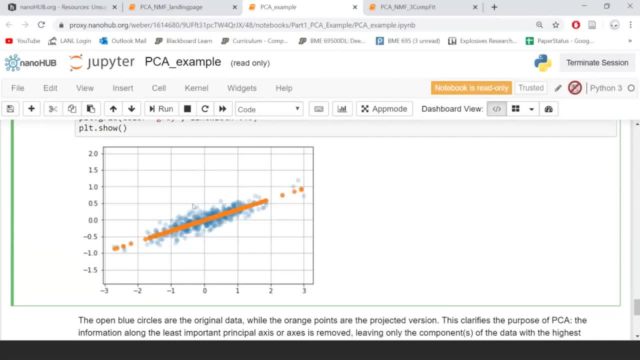 So we're going to go over this toy example where we're only going to address two input variables. But of course, as I stated, you can do PCA on n dimensions. So we're going to go over this toy example where we're only going to address two input. 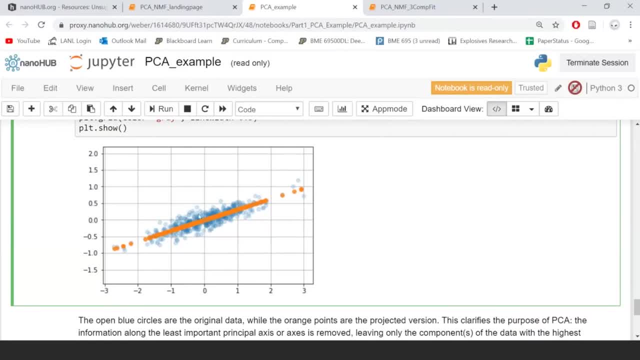 variables, But of course, as I stated, you can do PCA on n dimensions. So we're going to go over this toy example, where we're only going to address two input variables, But of course, as I stated, you can do PCA on n dimensions. 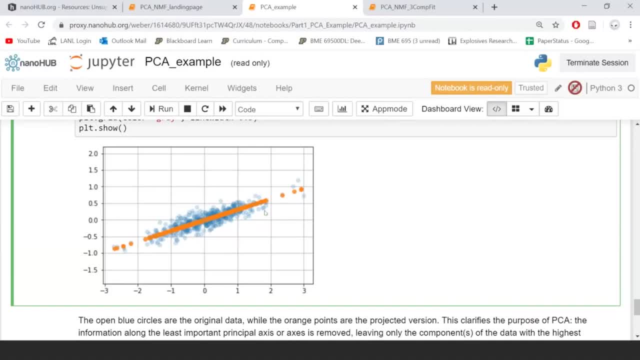 So we're going to go over this toy example where we're only going to address two input variables. But of course, as I stated, you can do PCA on n dimensions. So we're going to go over this toy example where we're only going to address two input. 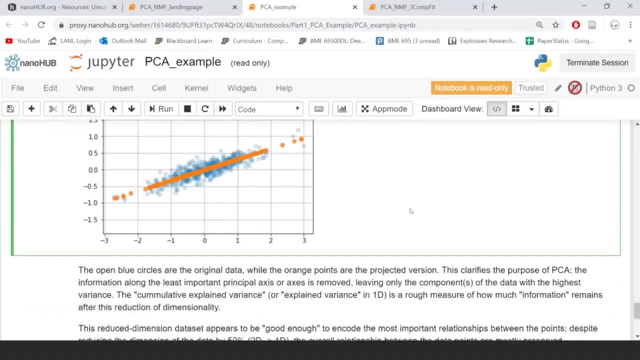 variables, But of course, as I stated, you can do PCA on n dimensions. So we're going to go over this toy example, where we're only going to address two input variables, But of course, as I stated, you can do PCA on n dimensions. 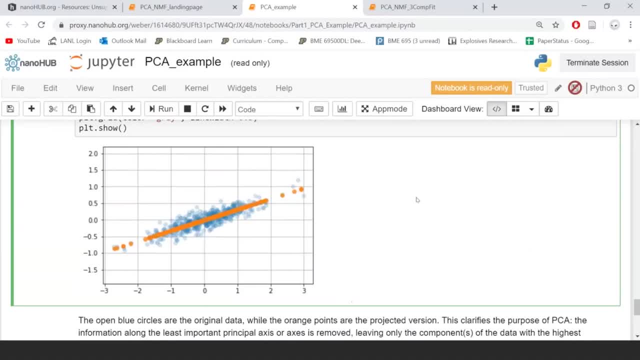 So we're going to go over this toy example where we're only going to address two input variables. But of course, as I stated, you can do PCA on n dimensions. So we're going to go over this toy example where we're only going to address two input. 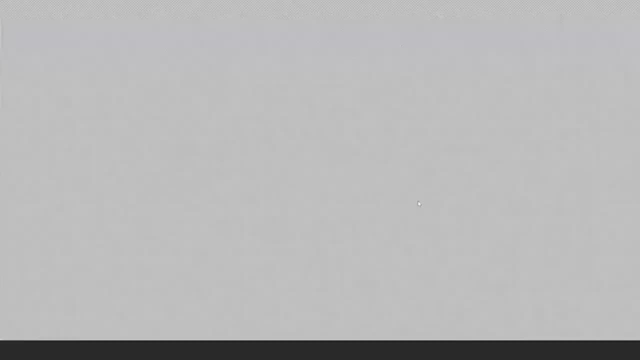 variables, But of course, as I stated, you can do PCA on n dimensions. So we're going to go over this toy example, where we're only going to address two input variables, But of course, as I stated, you can do PCA on n dimensions. 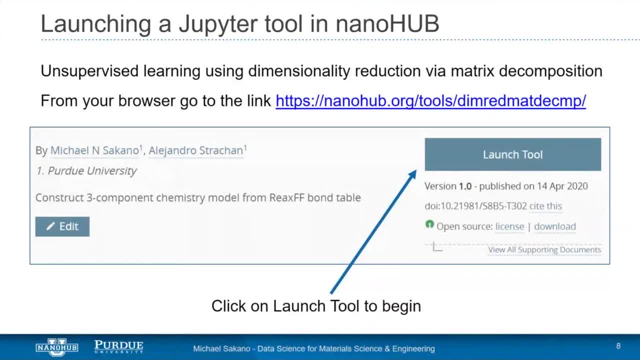 So we're going to go over this toy example where we're only going to address two input variables. But of course, as I stated, you can do PCA on n dimensions. So we're going to go over this toy example where we're only going to address two input. 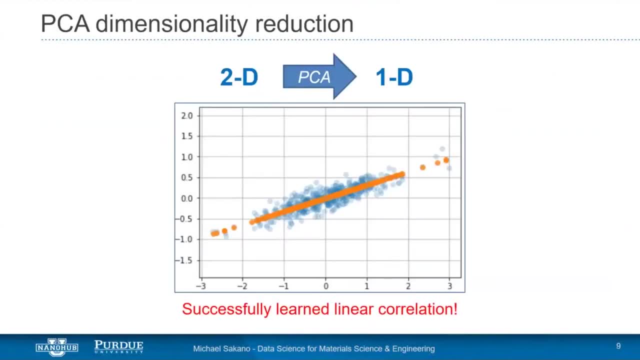 variables, But of course, as I stated, you can do PCA on n dimensions. So we're going to go over this toy example, where we're only going to address two input variables, But of course, as I stated, you can do PCA on n dimensions. 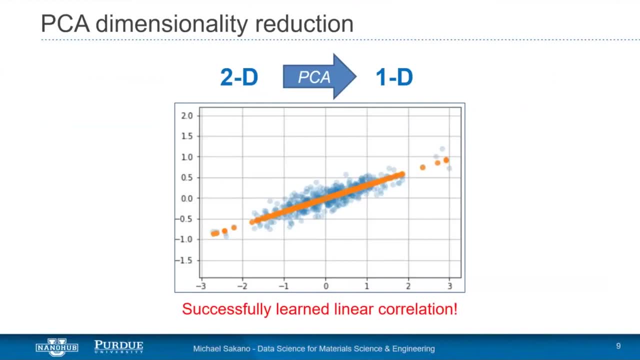 So we're going to go over this toy example where we're only going to address two input variables. But of course, as I stated, you can do PCA on n dimensions. So we're going to go over this toy example where we're only going to address two input. 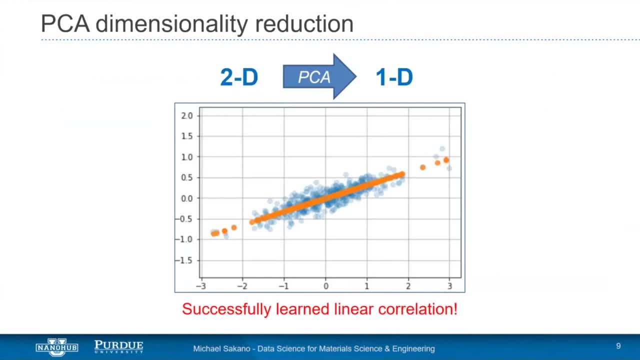 variables, But of course, as I stated, you can do PCA on n dimensions. So we're going to go over this toy example, where we're only going to address two input variables, But of course, as I stated, you can do PCA on n dimensions. 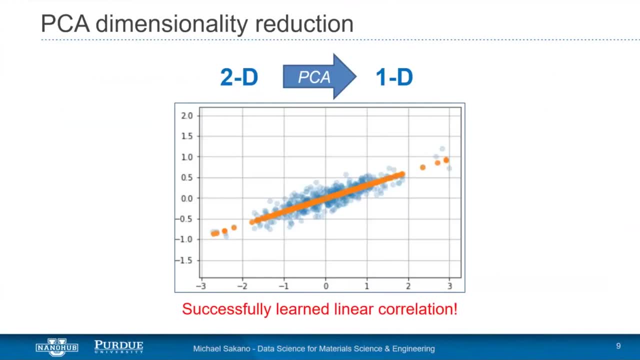 So we're going to go over this toy example where we're only going to address two input variables. But of course, as I stated, you can do PCA on n dimensions. So we're going to go over this toy example where we're only going to address two input. 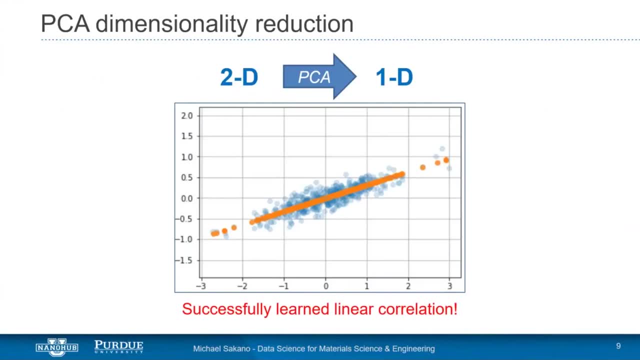 variables, But of course, as I stated, you can do PCA on n dimensions. So we're going to go over this toy example, where we're only going to address two input variables, But of course, as I stated, you can do PCA on n dimensions. 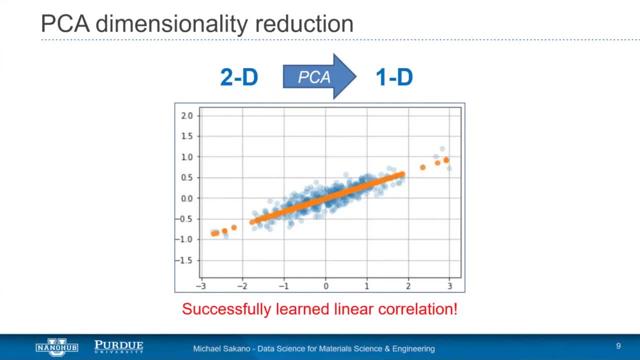 So we're going to go over this toy example where we're only going to address two input variables. But of course, as I stated, you can do PCA on n dimensions. So we're going to go over this toy example where we're only going to address two input. 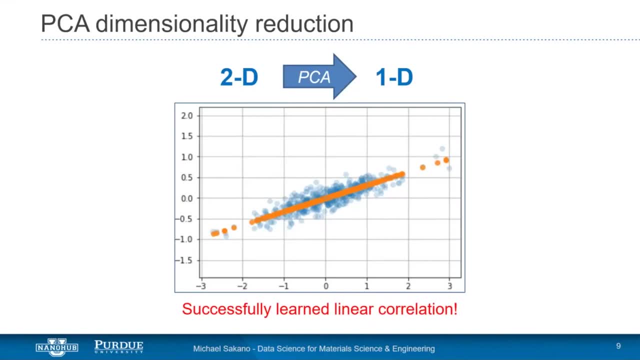 variables, But of course, as I stated, you can do PCA on n dimensions. So we're going to go over this toy example, where we're only going to address two input variables, But of course, as I stated, you can do PCA on n dimensions. 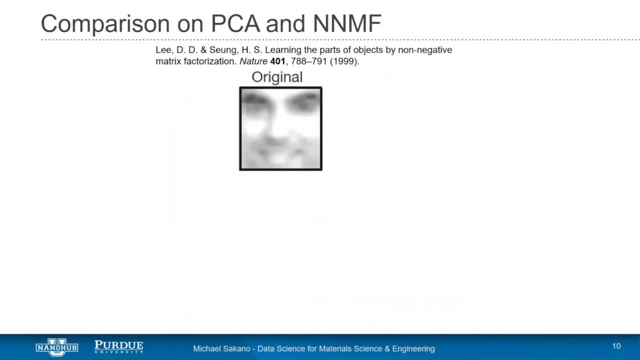 So we're going to go over this toy example where we're only going to address two input variables. But of course, as I stated, you can do PCA on n dimensions. So we're going to go over this toy example where we're only going to address two input. 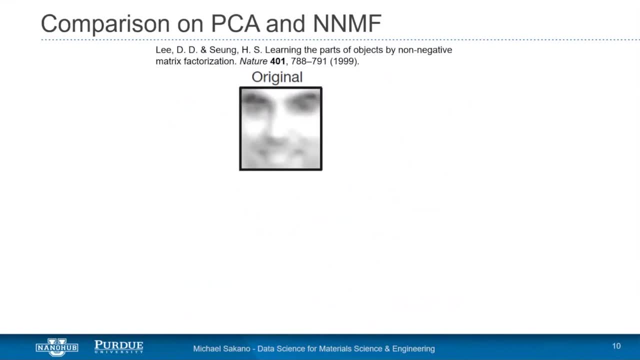 variables, But of course, as I stated, you can do PCA on n dimensions. So we're going to go over this toy example, where we're only going to address two input variables, But of course, as I stated, you can do PCA on n dimensions. 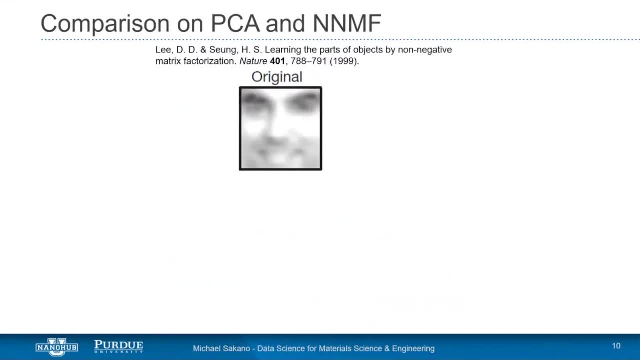 So we're going to go over this toy example where we're only going to address two input variables. But of course, as I stated, you can do PCA on n dimensions. So we're going to go over this toy example where we're only going to address two input. 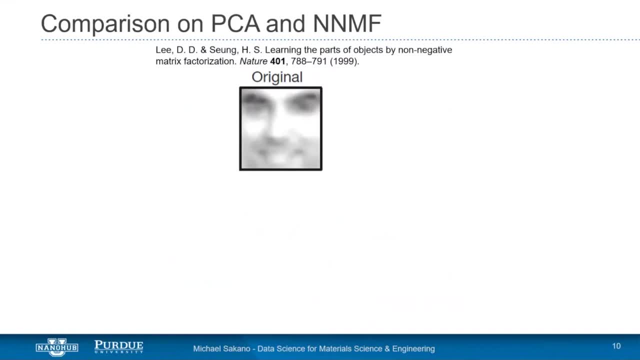 variables, But of course, as I stated, you can do PCA on n dimensions. So we're going to go over this toy example, where we're only going to address two input variables, But of course, as I stated, you can do PCA on n dimensions. 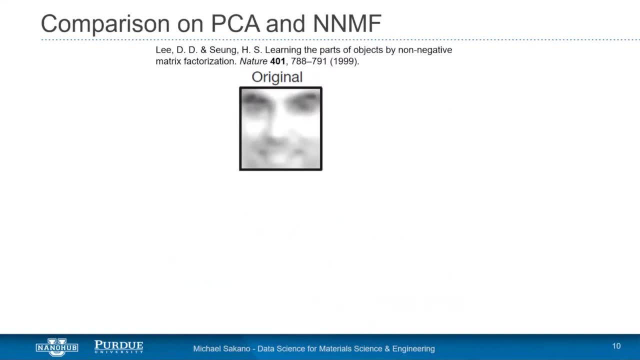 So we're going to go over this toy example where we're only going to address two input variables. But of course, as I stated, you can do PCA on n dimensions. So we're going to go over this toy example where we're only going to address two input. 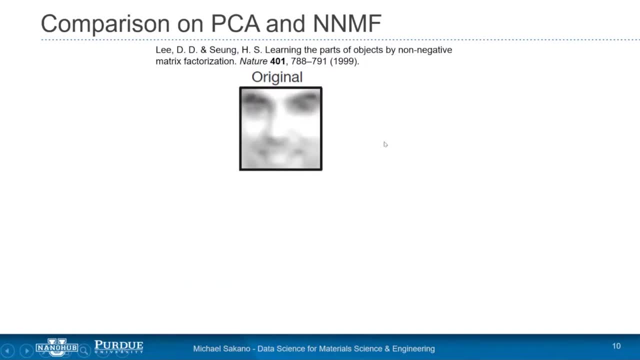 variables, But of course, as I stated, you can do PCA on n dimensions. So we're going to go over this toy example, where we're only going to address two input variables, But of course, as I stated, you can do PCA on n dimensions. 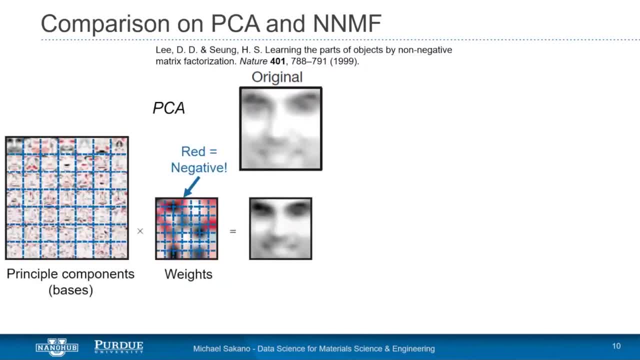 So we're going to go over this toy example where we're only going to address two input variables. But of course, as I stated, you can do PCA on n dimensions. So we're going to go over this toy example where we're only going to address two input. 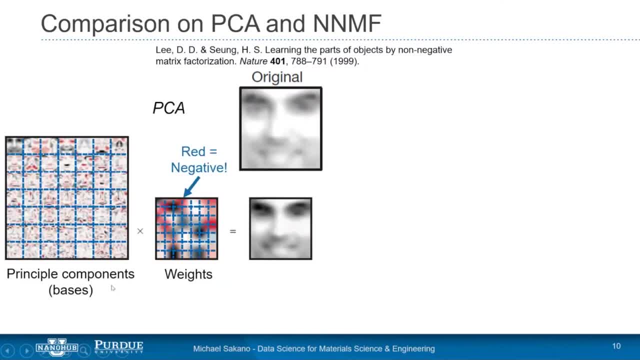 variables, But of course, as I stated, you can do PCA on n dimensions. So we're going to go over this toy example, where we're only going to address two input variables, But of course, as I stated, you can do PCA on n dimensions. 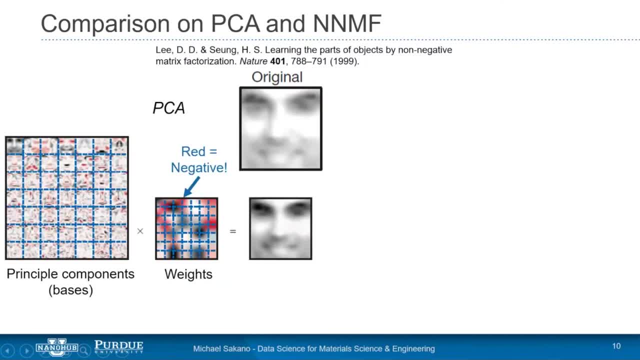 So we're going to go over this toy example where we're only going to address two input variables. But of course, as I stated, you can do PCA on n dimensions. So we're going to go over this toy example where we're only going to address two input. 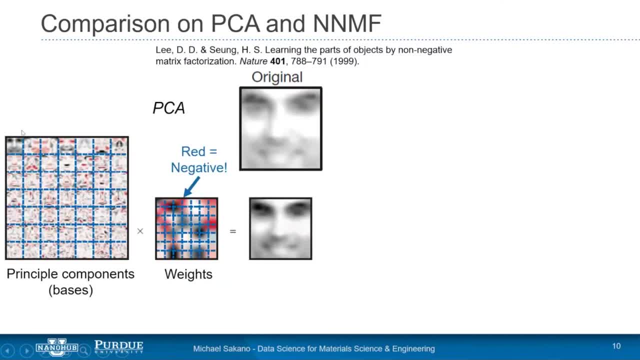 variables, But of course, as I stated, you can do PCA on n dimensions. So we're going to go over this toy example, where we're only going to address two input variables, But of course, as I stated, you can do PCA on n dimensions. 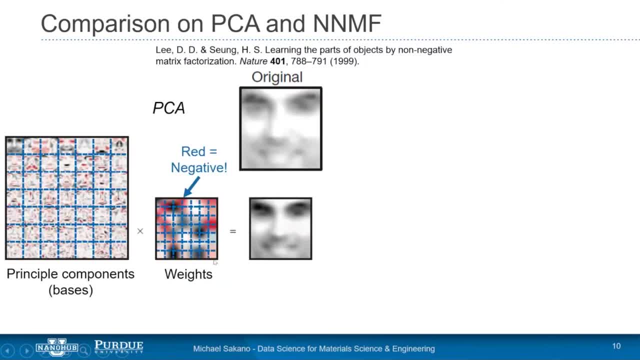 So we're going to go over this toy example where we're only going to address two input variables. But of course, as I stated, you can do PCA on n dimensions. So we're going to go over this toy example where we're only going to address two input. 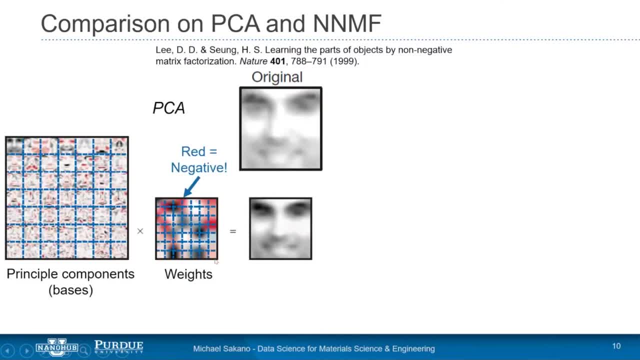 variables, But of course, as I stated, you can do PCA on n dimensions. So we're going to go over this toy example, where we're only going to address two input variables, But of course, as I stated, you can do PCA on n dimensions. 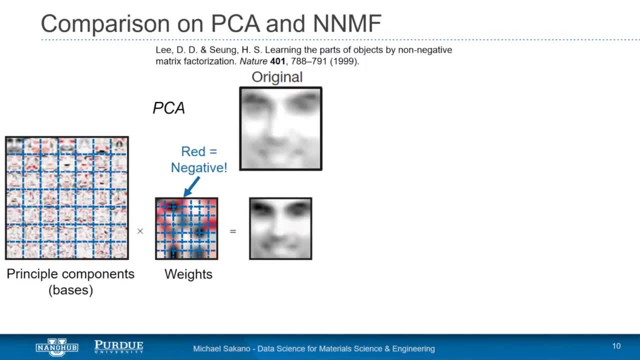 So we're going to go over this toy example where we're only going to address two input variables. But of course, as I stated, you can do PCA on n dimensions. So we're going to go over this toy example where we're only going to address two input. 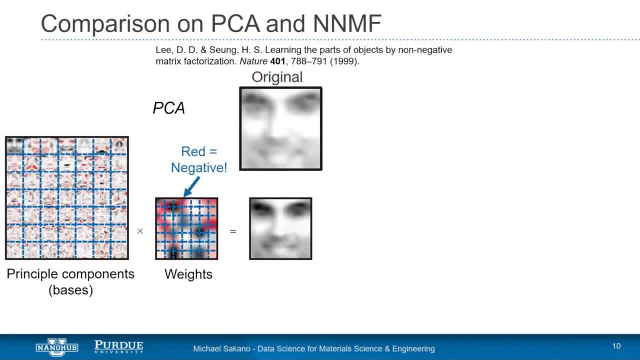 variables, But of course, as I stated, you can do PCA on n dimensions. So we're going to go over this toy example, where we're only going to address two input variables, But of course, as I stated, you can do PCA on n dimensions. 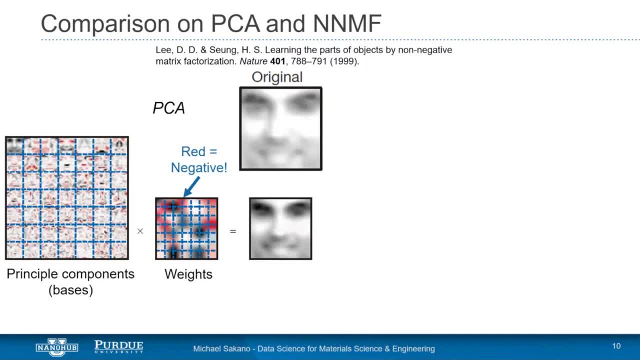 So we're going to go over this toy example where we're only going to address two input variables. But of course, as I stated, you can do PCA on n dimensions. So we're going to go over this toy example where we're only going to address two input. 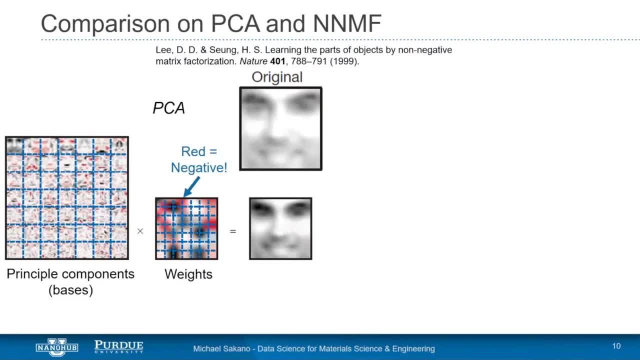 variables, But of course, as I stated, you can do PCA on n dimensions. So we're going to go over this toy example, where we're only going to address two input variables, But of course, as I stated, you can do PCA on n dimensions. 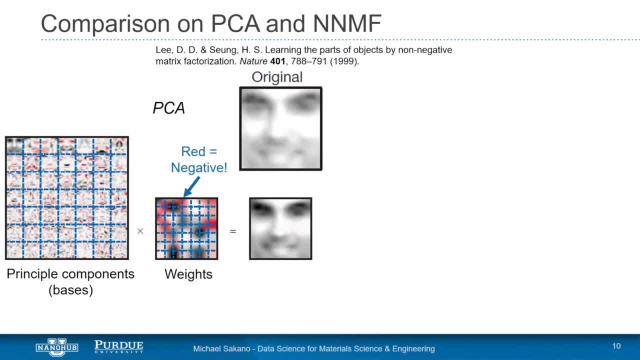 So we're going to go over this toy example where we're only going to address two input variables. But of course, as I stated, you can do PCA on n dimensions. So we're going to go over this toy example where we're only going to address two input. 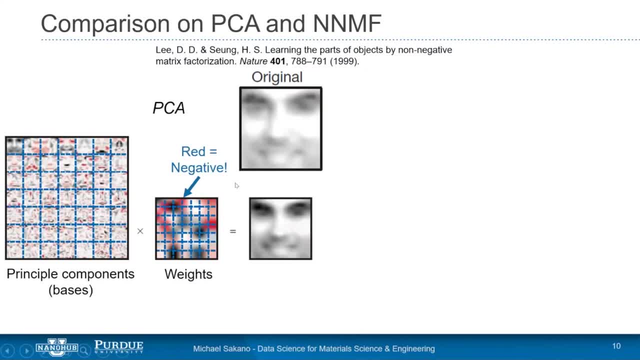 variables, But of course, as I stated, you can do PCA on n dimensions. So we're going to go over this toy example, where we're only going to address two input variables, But of course, as I stated, you can do PCA on n dimensions. 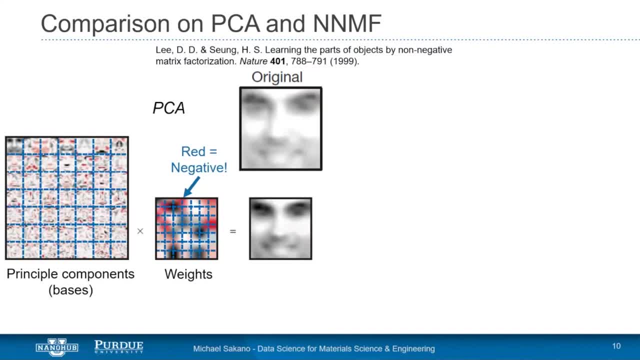 So we're going to go over this toy example where we're only going to address two input variables. But of course, as I stated, you can do PCA on n dimensions. So we're going to go over this toy example where we're only going to address two input. 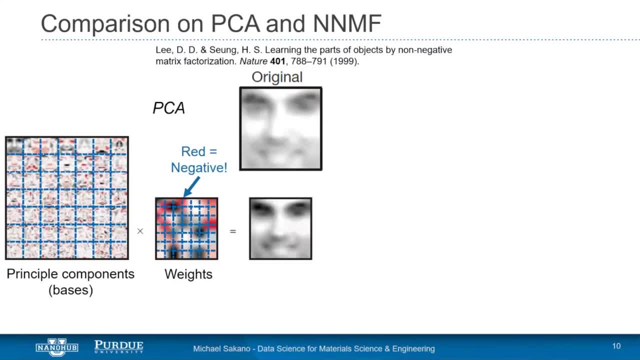 variables, But of course, as I stated, you can do PCA on n dimensions. So we're going to go over this toy example, where we're only going to address two input variables, But of course, as I stated, you can do PCA on n dimensions. 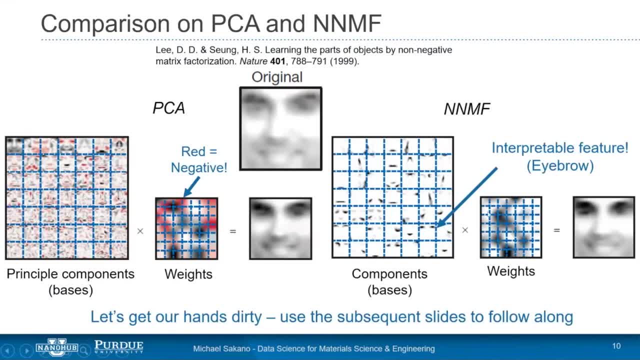 So we're going to go over this toy example where we're only going to address two input variables. But of course, as I stated, you can do PCA on n dimensions. So we're going to go over this toy example where we're only going to address two input. 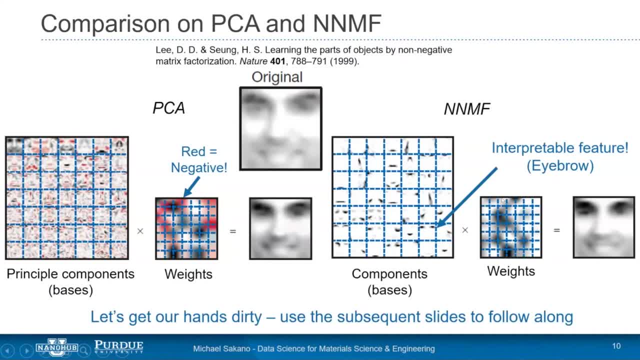 variables, But of course, as I stated, you can do PCA on n dimensions. So we're going to go over this toy example, where we're only going to address two input variables, But of course, as I stated, you can do PCA on n dimensions. 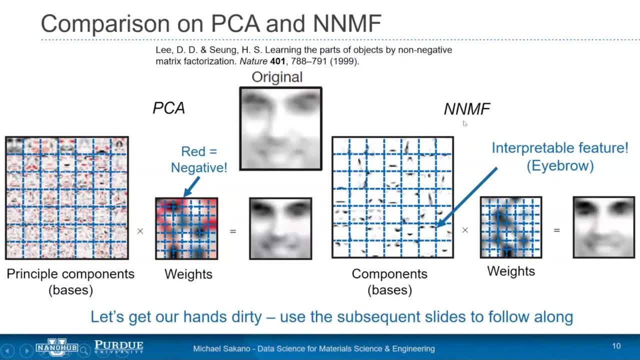 So we're going to go over this toy example where we're only going to address two input variables. But of course, as I stated, you can do PCA on n dimensions. So we're going to go over this toy example where we're only going to address two input. 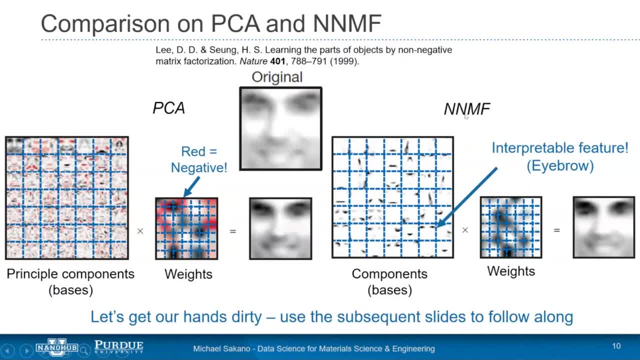 variables, But of course, as I stated, you can do PCA on n dimensions. So we're going to go over this toy example, where we're only going to address two input variables, But of course, as I stated, you can do PCA on n dimensions. 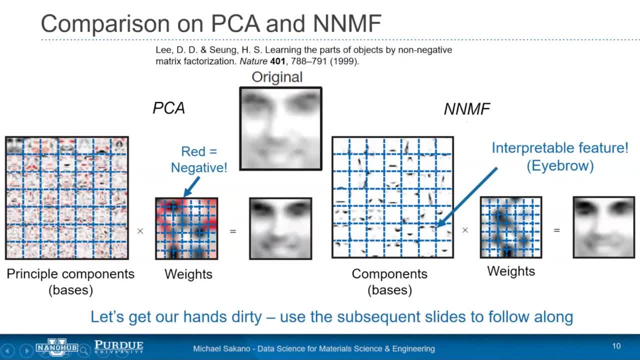 So we're going to go over this toy example where we're only going to address two input variables. But of course, as I stated, you can do PCA on n dimensions. So we're going to go over this toy example where we're only going to address two input. 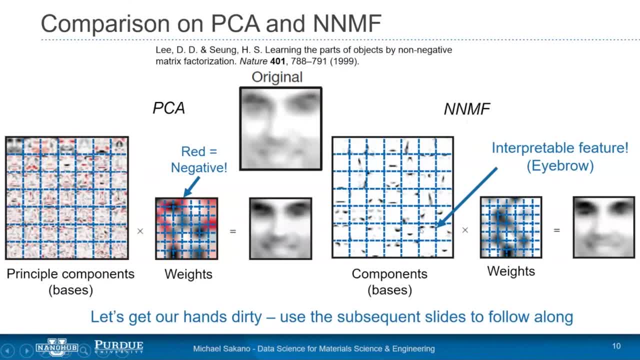 variables, But of course, as I stated, you can do PCA on n dimensions. So we're going to go over this toy example, where we're only going to address two input variables, But of course, as I stated, you can do PCA on n dimensions. 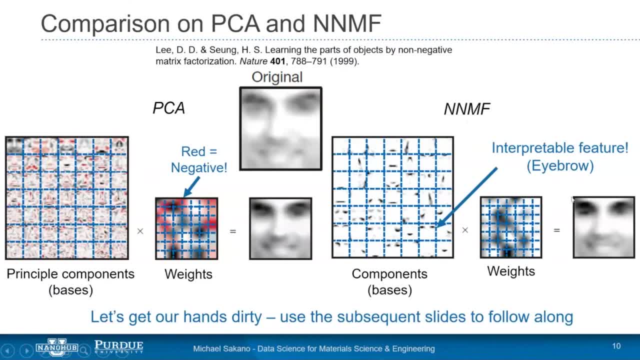 So we're going to go over this toy example where we're only going to address two input variables. But of course, as I stated, you can do PCA on n dimensions. So we're going to go over this toy example where we're only going to address two input. 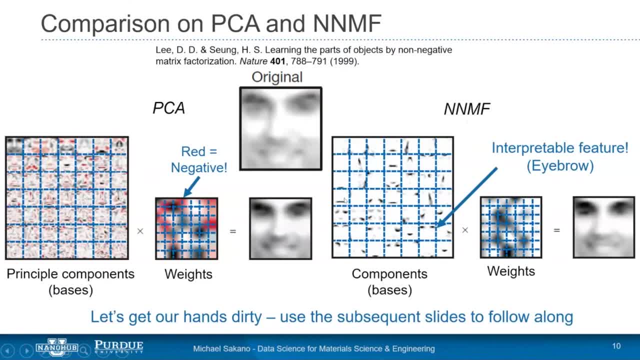 variables, But of course, as I stated, you can do PCA on n dimensions. So we're going to go over this toy example, where we're only going to address two input variables, But of course, as I stated, you can do PCA on n dimensions. 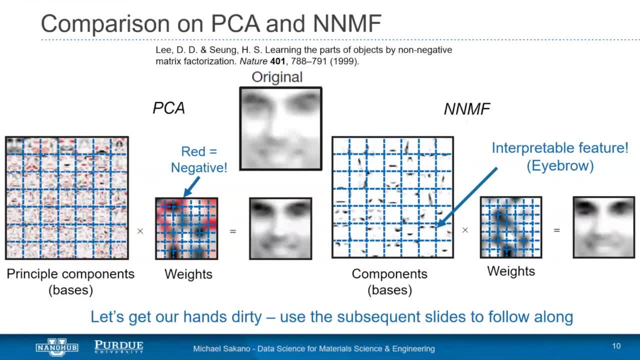 So we're going to go over this toy example where we're only going to address two input variables. But of course, as I stated, you can do PCA on n dimensions. So we're going to go over this toy example where we're only going to address two input. 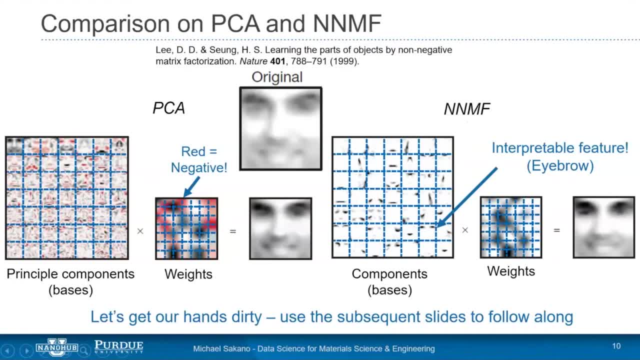 variables, But of course, as I stated, you can do PCA on n dimensions. So we're going to go over this toy example, where we're only going to address two input variables, But of course, as I stated, you can do PCA on n dimensions. 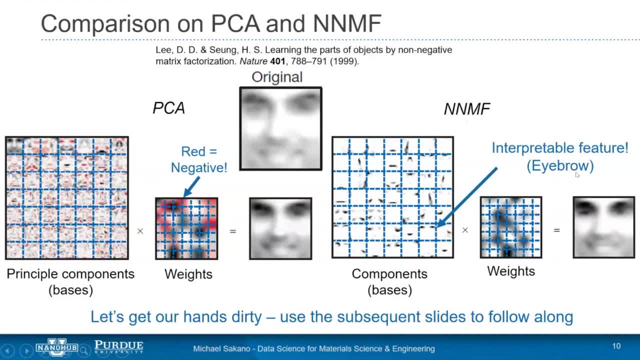 So we're going to go over this toy example where we're only going to address two input variables. But of course, as I stated, you can do PCA on n dimensions. So we're going to go over this toy example where we're only going to address two input. 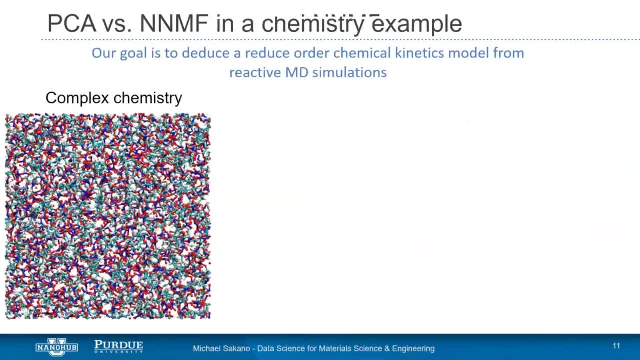 variables, But of course, as I stated, you can do PCA on n dimensions. So we're going to go over this toy example, where we're only going to address two input variables, But of course, as I stated, you can do PCA on n dimensions. 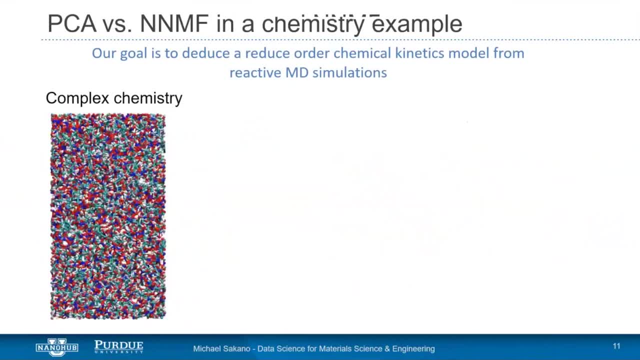 So we're going to go over this toy example where we're only going to address two input variables. But of course, as I stated, you can do PCA on n dimensions. So we're going to go over this toy example where we're only going to address two input. 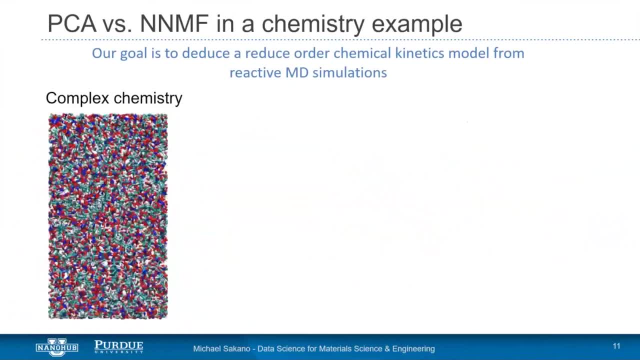 variables, But of course, as I stated, you can do PCA on n dimensions. So we're going to go over this toy example, where we're only going to address two input variables, But of course, as I stated, you can do PCA on n dimensions. 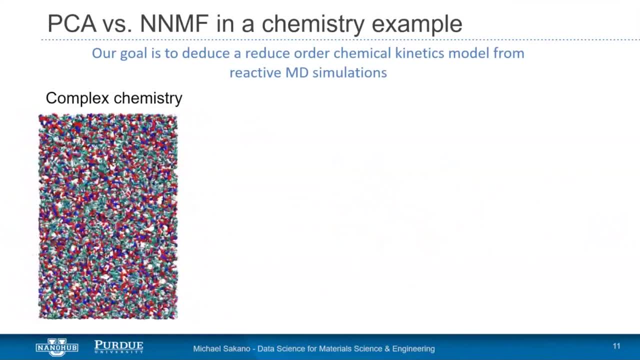 So we're going to go over this toy example where we're only going to address two input variables. But of course, as I stated, you can do PCA on n dimensions. So we're going to go over this toy example where we're only going to address two input. 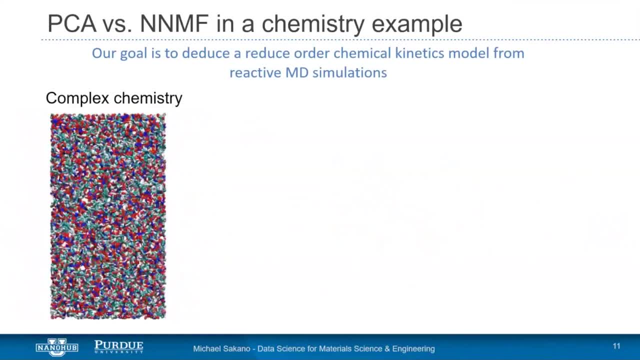 variables, But of course, as I stated, you can do PCA on n dimensions. So we're going to go over this toy example, where we're only going to address two input variables, But of course, as I stated, you can do PCA on n dimensions. 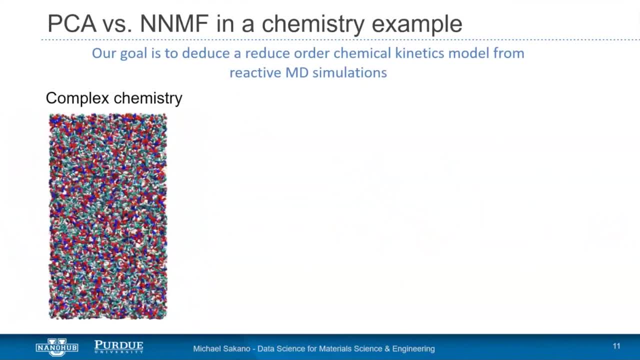 So we're going to go over this toy example where we're only going to address two input variables. But of course, as I stated, you can do PCA on n dimensions. So we're going to go over this toy example where we're only going to address two input. 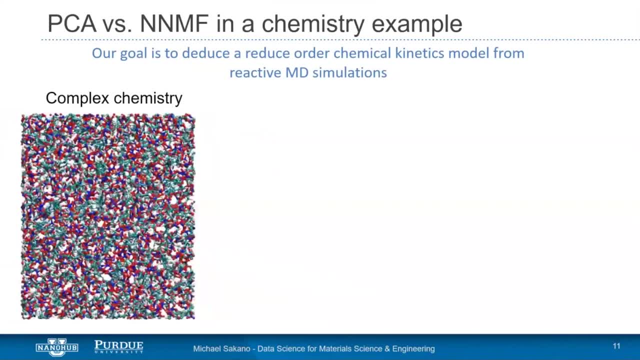 variables, But of course, as I stated, you can do PCA on n dimensions. So we're going to go over this toy example, where we're only going to address two input variables, But of course, as I stated, you can do PCA on n dimensions. 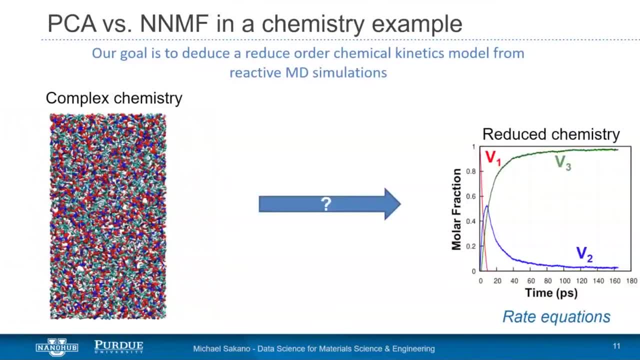 So we're going to go over this toy example where we're only going to address two input variables. But of course, as I stated, you can do PCA on n dimensions. So we're going to go over this toy example where we're only going to address two input. 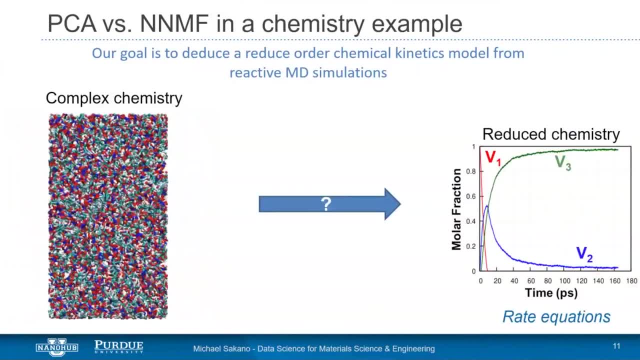 variables, But of course, as I stated, you can do PCA on n dimensions. So we're going to go over this toy example, where we're only going to address two input variables, But of course, as I stated, you can do PCA on n dimensions. 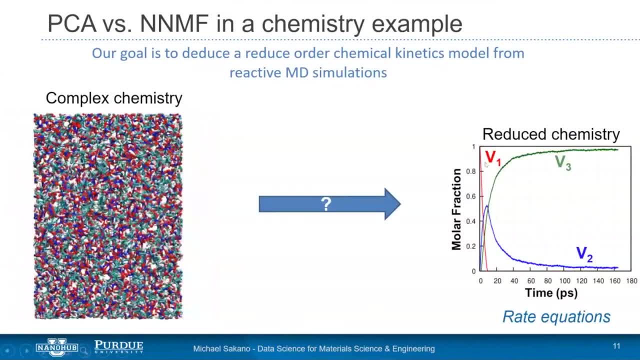 So we're going to go over this toy example where we're only going to address two input variables. But of course, as I stated, you can do PCA on n dimensions. So we're going to go over this toy example where we're only going to address two input. 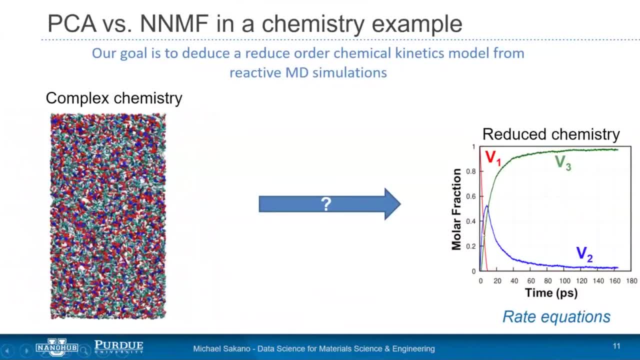 variables, But of course, as I stated, you can do PCA on n dimensions. So we're going to go over this toy example, where we're only going to address two input variables, But of course, as I stated, you can do PCA on n dimensions. 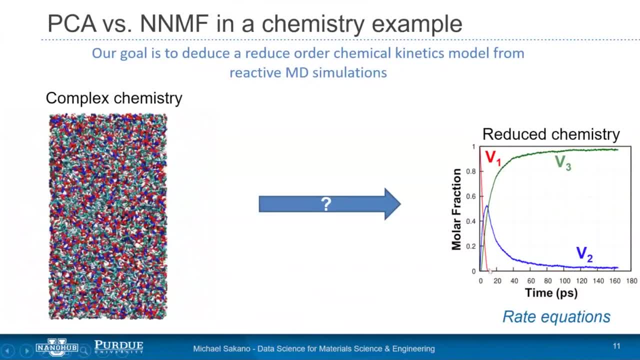 So we're going to go over this toy example where we're only going to address two input variables. But of course, as I stated, you can do PCA on n dimensions. So we're going to go over this toy example where we're only going to address two input. 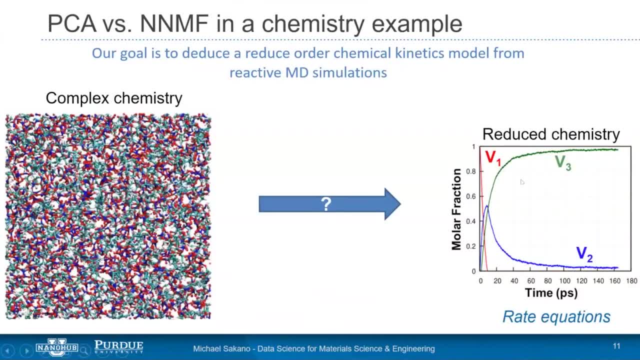 variables, But of course, as I stated, you can do PCA on n dimensions. So we're going to go over this toy example, where we're only going to address two input variables, But of course, as I stated, you can do PCA on n dimensions. 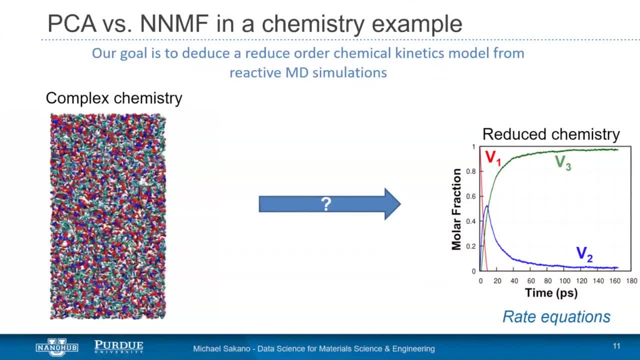 So we're going to go over this toy example where we're only going to address two input variables. But of course, as I stated, you can do PCA on n dimensions. So we're going to go over this toy example where we're only going to address two input. 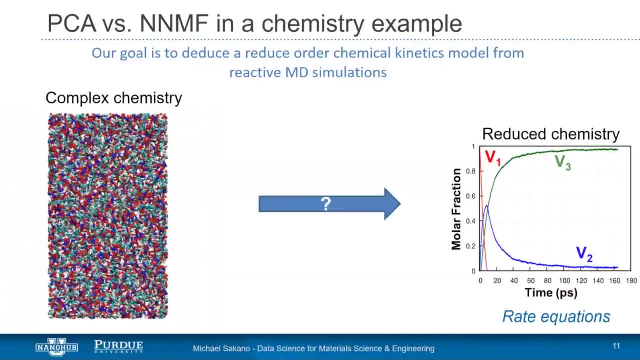 variables, But of course, as I stated, you can do PCA on n dimensions. So we're going to go over this toy example, where we're only going to address two input variables, But of course, as I stated, you can do PCA on n dimensions. 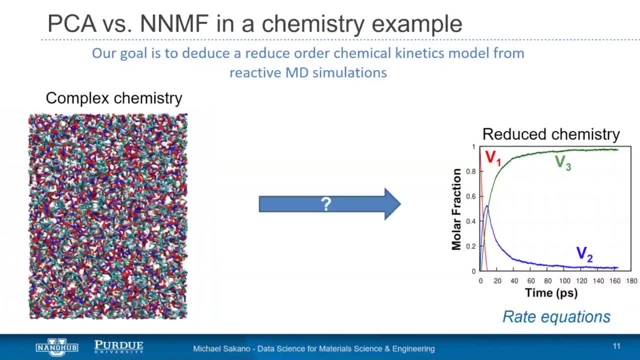 So we're going to go over this toy example where we're only going to address two input variables. But of course, as I stated, you can do PCA on n dimensions. So we're going to go over this toy example where we're only going to address two input. 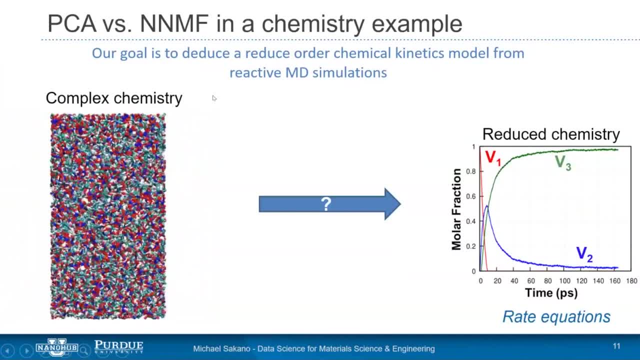 variables, But of course, as I stated, you can do PCA on n dimensions. So we're going to go over this toy example, where we're only going to address two input variables, But of course, as I stated, you can do PCA on n dimensions. 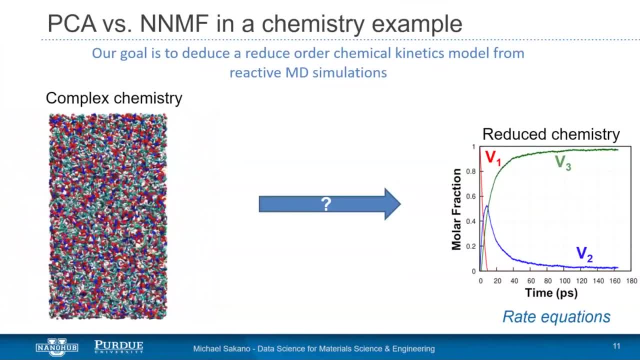 So we're going to go over this toy example where we're only going to address two input variables. But of course, as I stated, you can do PCA on n dimensions. So we're going to go over this toy example where we're only going to address two input. 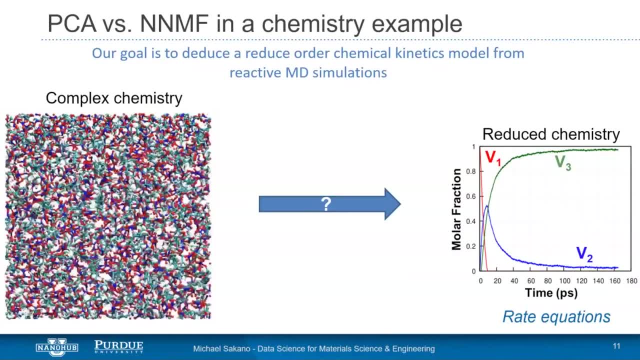 variables, But of course, as I stated, you can do PCA on n dimensions. So we're going to go over this toy example, where we're only going to address two input variables, But of course, as I stated, you can do PCA on n dimensions. 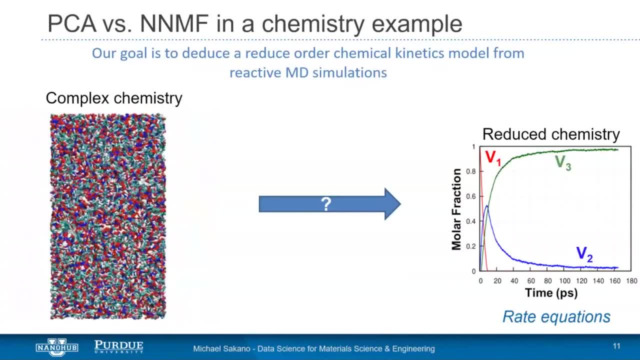 So we're going to go over this toy example where we're only going to address two input variables. But of course, as I stated, you can do PCA on n dimensions. So we're going to go over this toy example where we're only going to address two input. 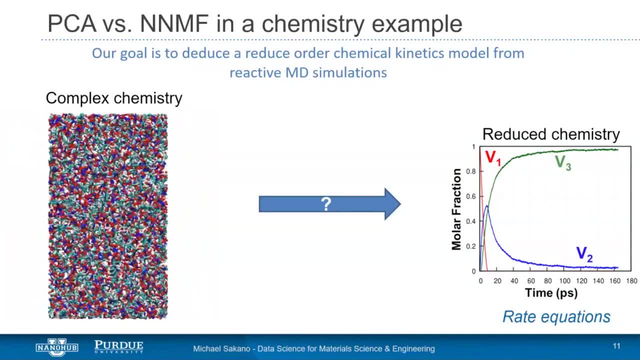 variables, But of course, as I stated, you can do PCA on n dimensions. So we're going to go over this toy example, where we're only going to address two input variables, But of course, as I stated, you can do PCA on n dimensions. 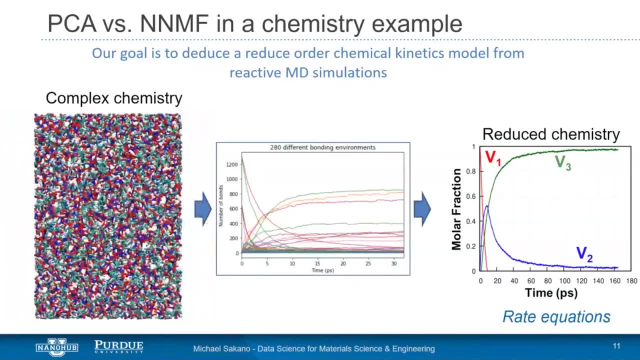 So we're going to go over this toy example where we're only going to address two input variables. But of course, as I stated, you can do PCA on n dimensions. So we're going to go over this toy example where we're only going to address two input. 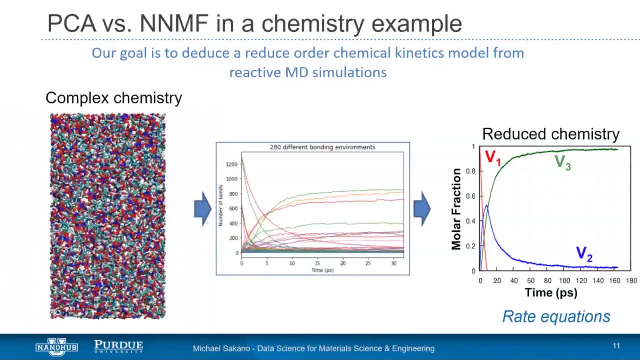 variables, But of course, as I stated, you can do PCA on n dimensions. So we're going to go over this toy example, where we're only going to address two input variables, But of course, as I stated, you can do PCA on n dimensions. 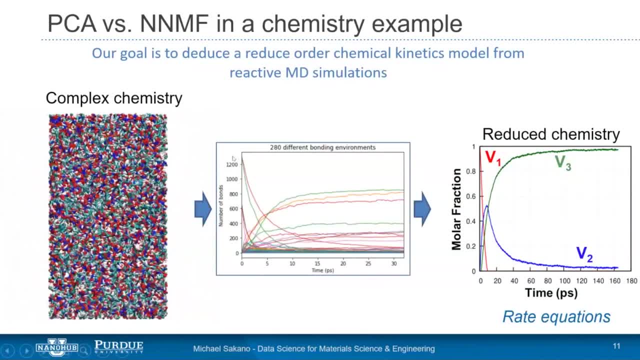 So we're going to go over this toy example where we're only going to address two input variables. But of course, as I stated, you can do PCA on n dimensions. So we're going to go over this toy example where we're only going to address two input. 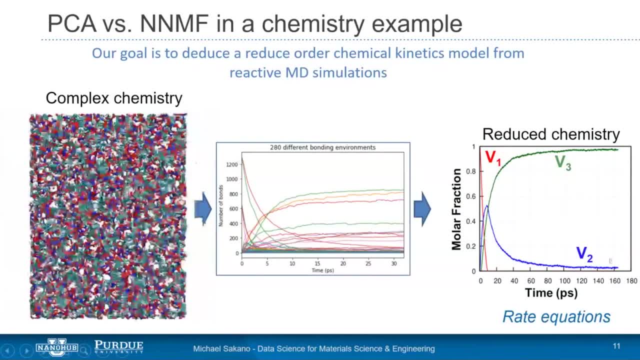 variables, But of course, as I stated, you can do PCA on n dimensions. So we're going to go over this toy example, where we're only going to address two input variables, But of course, as I stated, you can do PCA on n dimensions. 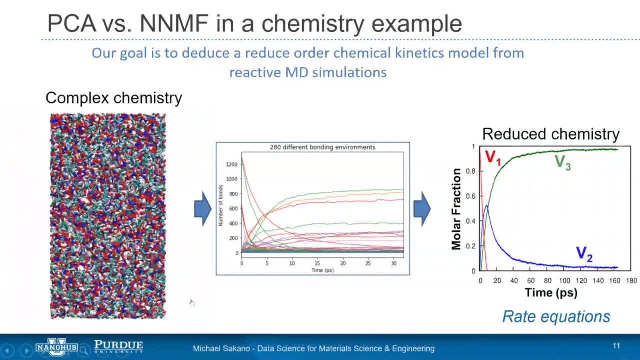 So we're going to go over this toy example where we're only going to address two input variables. But of course, as I stated, you can do PCA on n dimensions. So we're going to go over this toy example where we're only going to address two input. 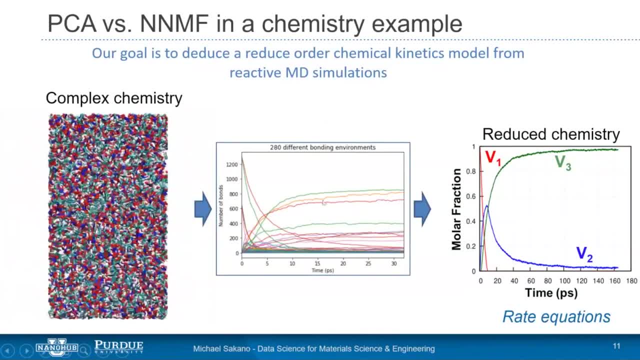 variables, But of course, as I stated, you can do PCA on n dimensions. So we're going to go over this toy example, where we're only going to address two input variables, But of course, as I stated, you can do PCA on n dimensions. 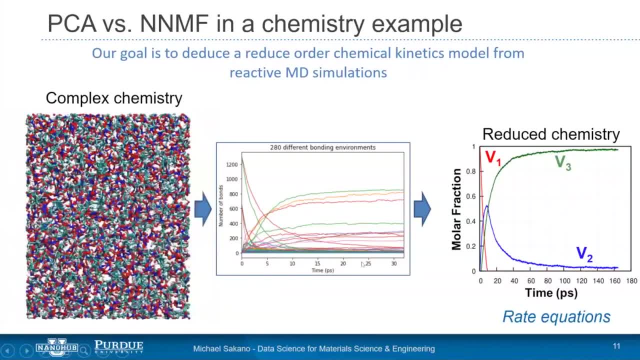 So we're going to go over this toy example where we're only going to address two input variables. But of course, as I stated, you can do PCA on n dimensions. So we're going to go over this toy example where we're only going to address two input. 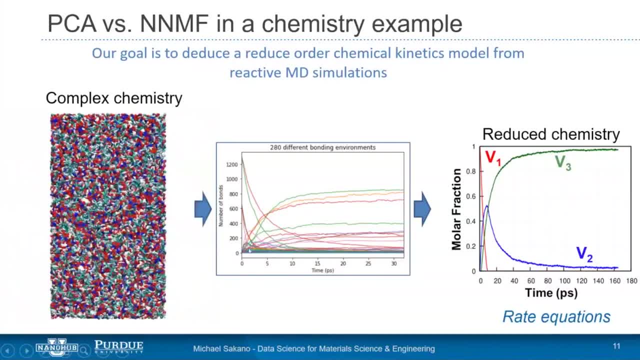 variables, But of course, as I stated, you can do PCA on n dimensions. So we're going to go over this toy example, where we're only going to address two input variables, But of course, as I stated, you can do PCA on n dimensions. 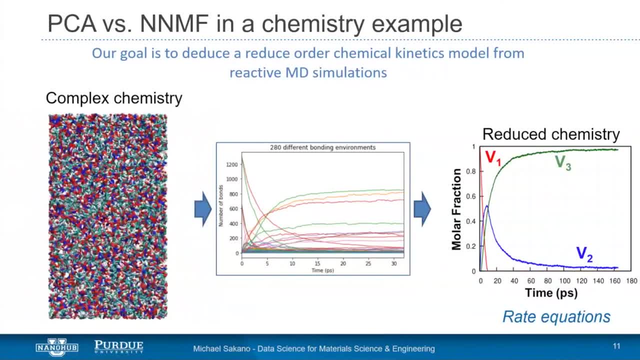 So we're going to go over this toy example where we're only going to address two input variables. But of course, as I stated, you can do PCA on n dimensions. So we're going to go over this toy example where we're only going to address two input. 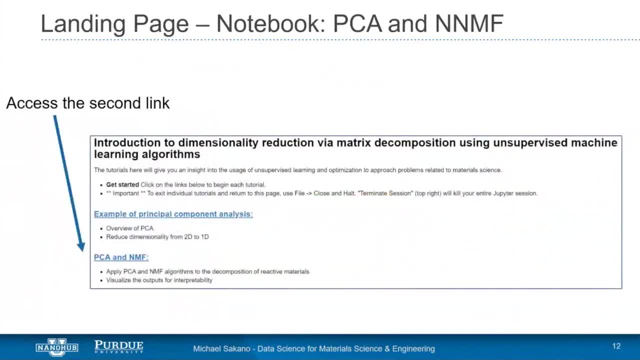 variables, But of course, as I stated, you can do PCA on n dimensions. So we're going to go over this toy example, where we're only going to address two input variables, But of course, as I stated, you can do PCA on n dimensions. 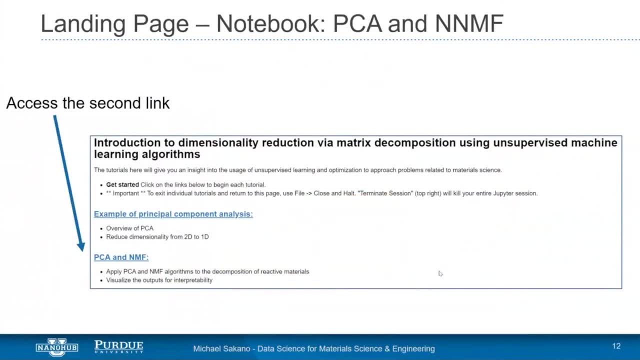 So we're going to go over this toy example where we're only going to address two input variables. But of course, as I stated, you can do PCA on n dimensions. So we're going to go over this toy example where we're only going to address two input. 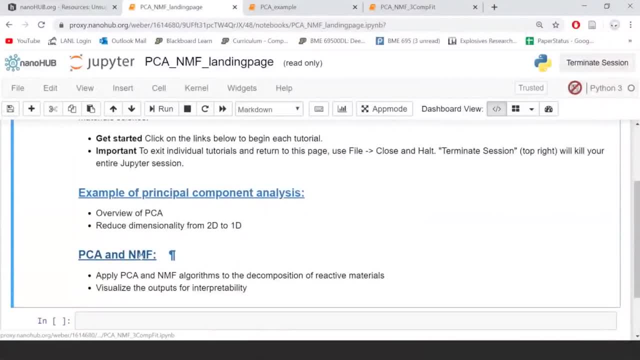 variables, But of course, as I stated, you can do PCA on n dimensions. So we're going to go over this toy example, where we're only going to address two input variables, But of course, as I stated, you can do PCA on n dimensions. 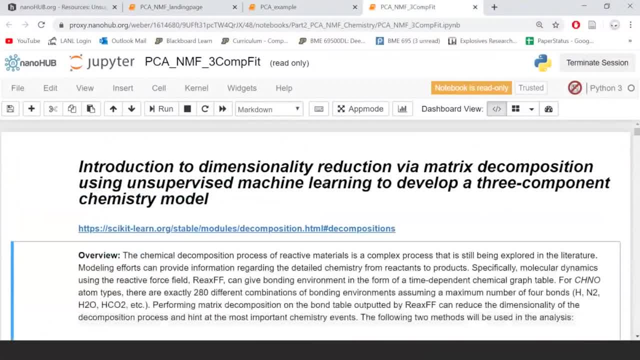 So we're going to go over this toy example where we're only going to address two input variables. But of course, as I stated, you can do PCA on n dimensions. So we're going to go over this toy example where we're only going to address two input. 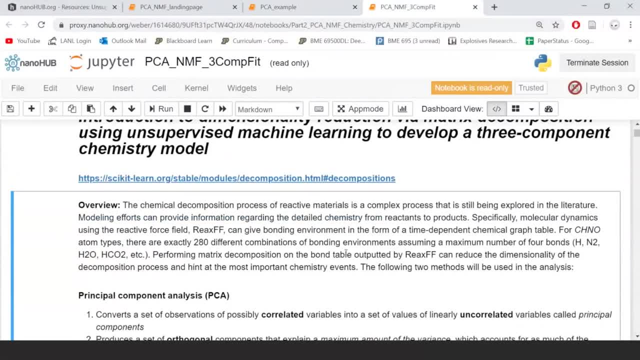 variables, But of course, as I stated, you can do PCA on n dimensions. So we're going to go over this toy example, where we're only going to address two input variables, But of course, as I stated, you can do PCA on n dimensions. 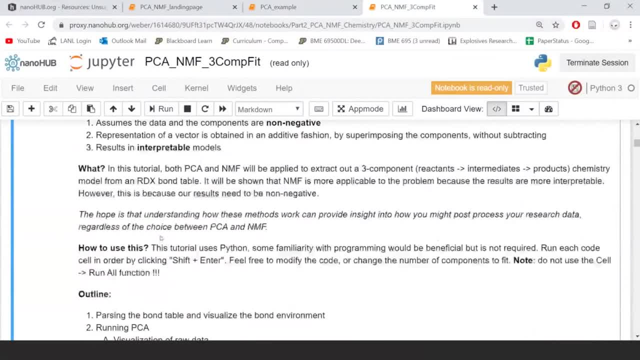 So we're going to go over this toy example where we're only going to address two input variables. But of course, as I stated, you can do PCA on n dimensions. So we're going to go over this toy example where we're only going to address two input. 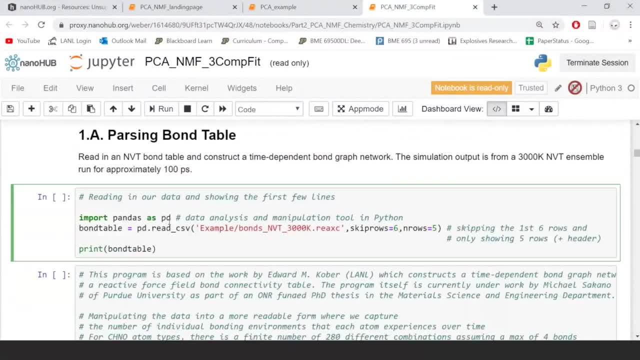 variables, But of course, as I stated, you can do PCA on n dimensions. So we're going to go over this toy example, where we're only going to address two input variables, But of course, as I stated, you can do PCA on n dimensions. 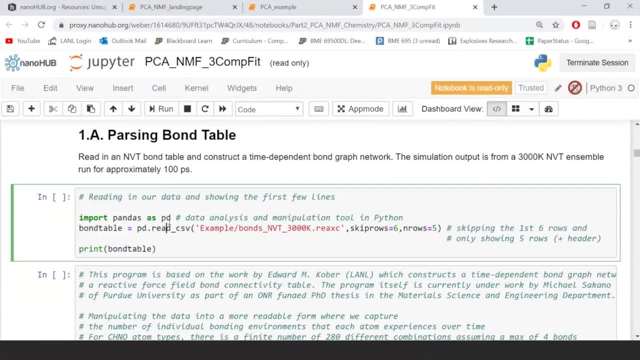 So we're going to go over this toy example where we're only going to address two input variables. But of course, as I stated, you can do PCA on n dimensions. So we're going to go over this toy example where we're only going to address two input. 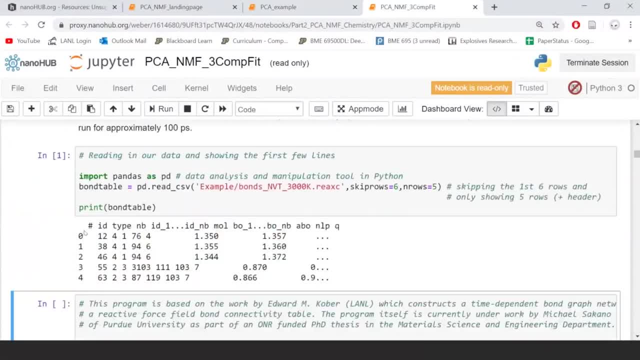 variables, But of course, as I stated, you can do PCA on n dimensions. So we're going to go over this toy example, where we're only going to address two input variables, But of course, as I stated, you can do PCA on n dimensions. 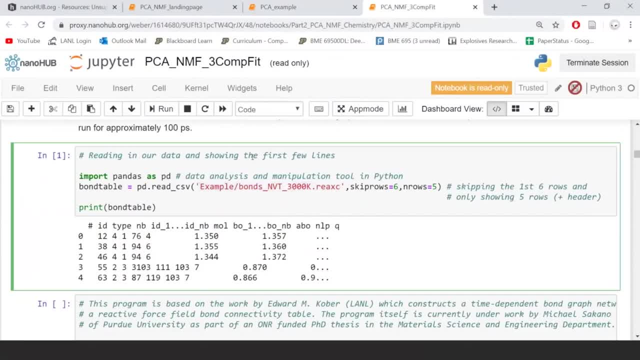 So we're going to go over this toy example where we're only going to address two input variables. But of course, as I stated, you can do PCA on n dimensions. So we're going to go over this toy example where we're only going to address two input. 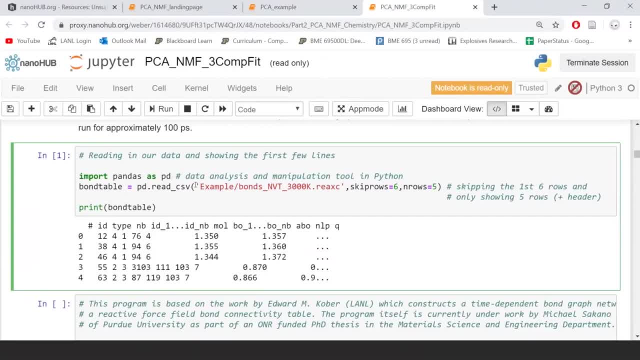 variables, But of course, as I stated, you can do PCA on n dimensions. So we're going to go over this toy example, where we're only going to address two input variables, But of course, as I stated, you can do PCA on n dimensions. 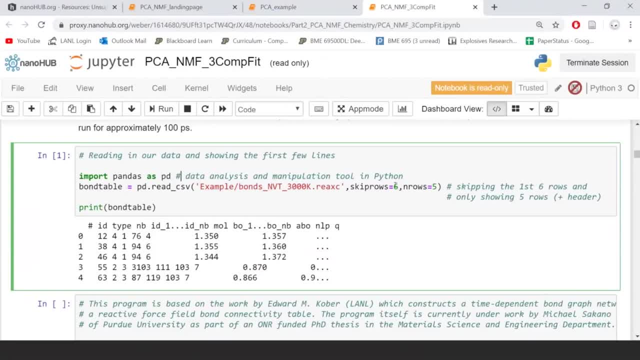 So we're going to go over this toy example where we're only going to address two input variables. But of course, as I stated, you can do PCA on n dimensions. So we're going to go over this toy example where we're only going to address two input. 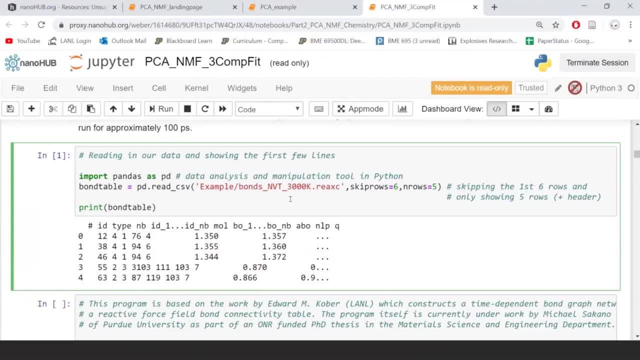 variables, But of course, as I stated, you can do PCA on n dimensions. So we're going to go over this toy example, where we're only going to address two input variables, But of course, as I stated, you can do PCA on n dimensions. 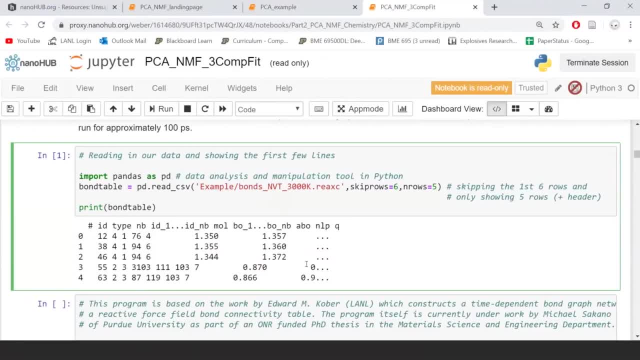 So we're going to go over this toy example where we're only going to address two input variables. But of course, as I stated, you can do PCA on n dimensions. So we're going to go over this toy example where we're only going to address two input. 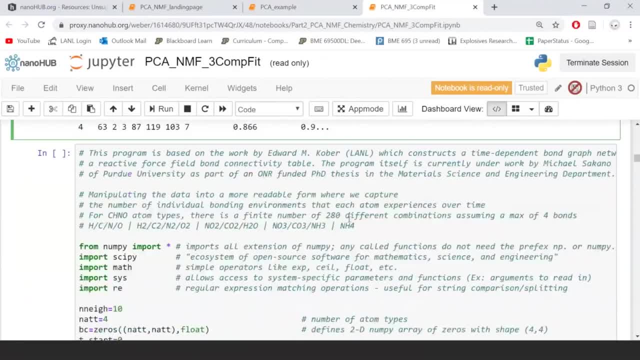 variables, But of course, as I stated, you can do PCA on n dimensions. So we're going to go over this toy example, where we're only going to address two input variables, But of course, as I stated, you can do PCA on n dimensions. 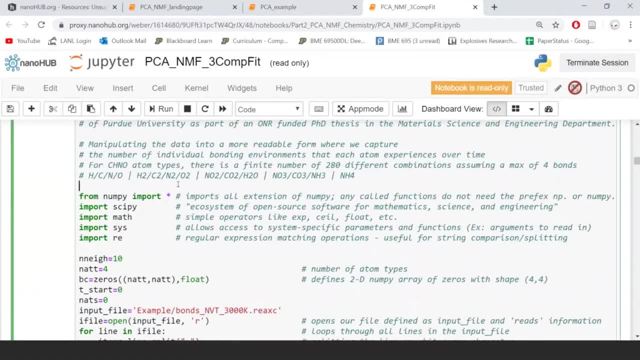 So we're going to go over this toy example where we're only going to address two input variables. But of course, as I stated, you can do PCA on n dimensions. So we're going to go over this toy example where we're only going to address two input. 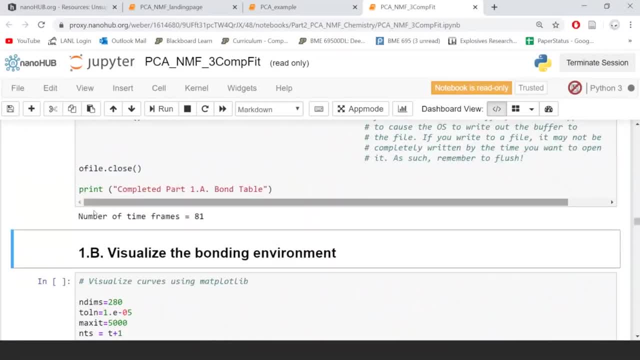 variables, But of course, as I stated, you can do PCA on n dimensions. So we're going to go over this toy example, where we're only going to address two input variables, But of course, as I stated, you can do PCA on n dimensions. 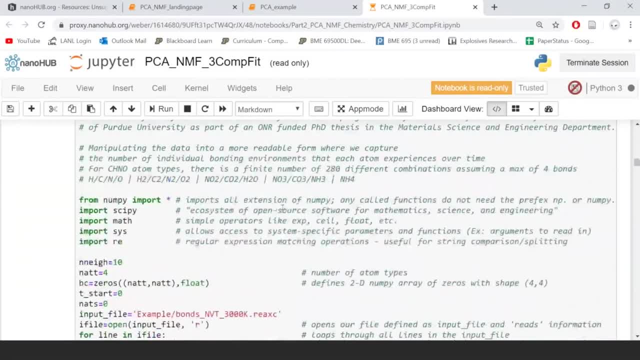 So we're going to go over this toy example where we're only going to address two input variables. But of course, as I stated, you can do PCA on n dimensions. So we're going to go over this toy example where we're only going to address two input. 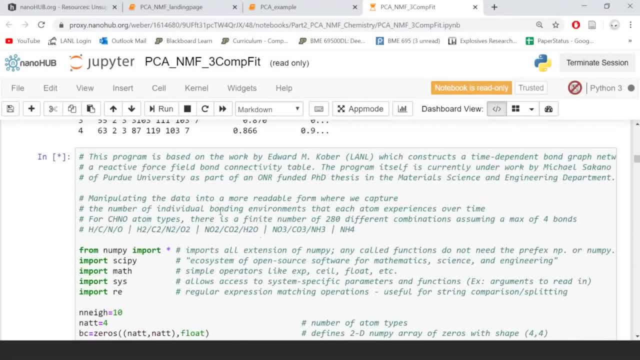 variables, But of course, as I stated, you can do PCA on n dimensions. So we're going to go over this toy example, where we're only going to address two input variables, But of course, as I stated, you can do PCA on n dimensions. 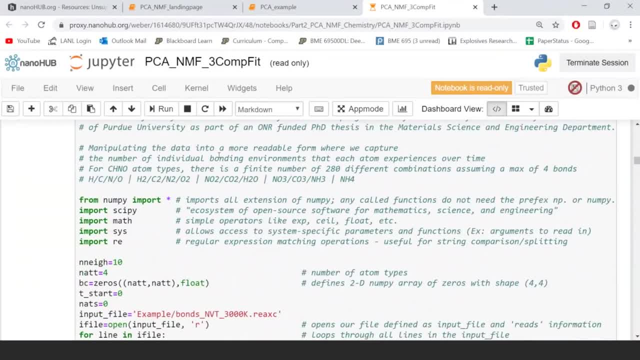 So we're going to go over this toy example where we're only going to address two input variables. But of course, as I stated, you can do PCA on n dimensions. So we're going to go over this toy example where we're only going to address two input. 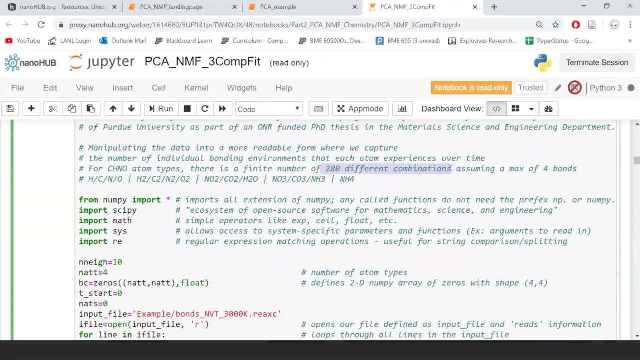 variables, But of course, as I stated, you can do PCA on n dimensions. So we're going to go over this toy example, where we're only going to address two input variables, But of course, as I stated, you can do PCA on n dimensions. 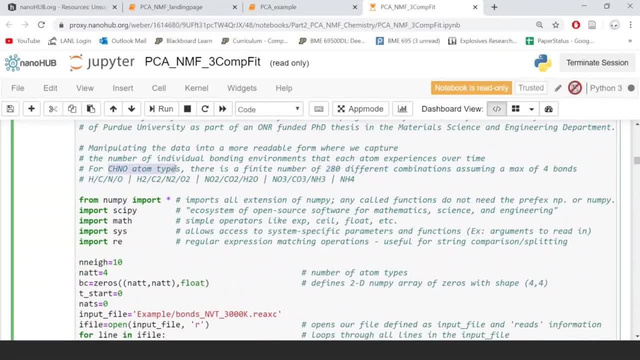 So we're going to go over this toy example where we're only going to address two input variables. But of course, as I stated, you can do PCA on n dimensions. So we're going to go over this toy example where we're only going to address two input. 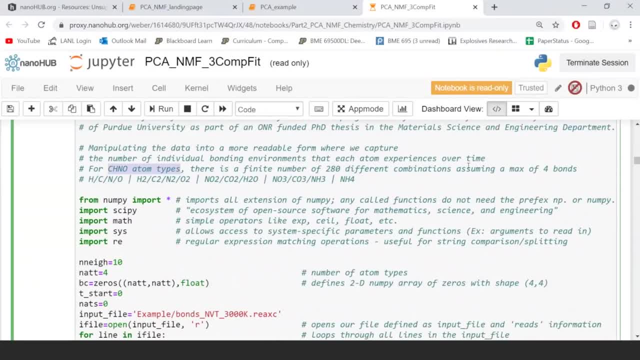 variables, But of course, as I stated, you can do PCA on n dimensions. So we're going to go over this toy example, where we're only going to address two input variables, But of course, as I stated, you can do PCA on n dimensions. 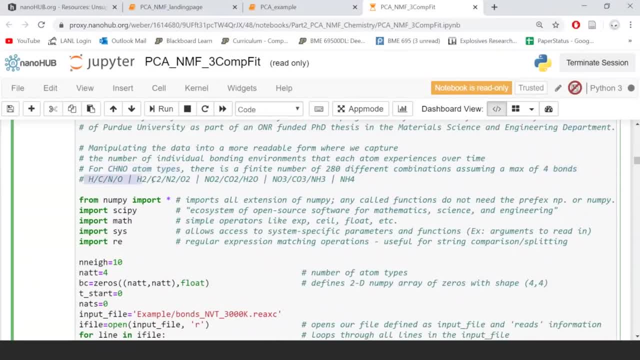 So we're going to go over this toy example where we're only going to address two input variables. But of course, as I stated, you can do PCA on n dimensions. So we're going to go over this toy example where we're only going to address two input. 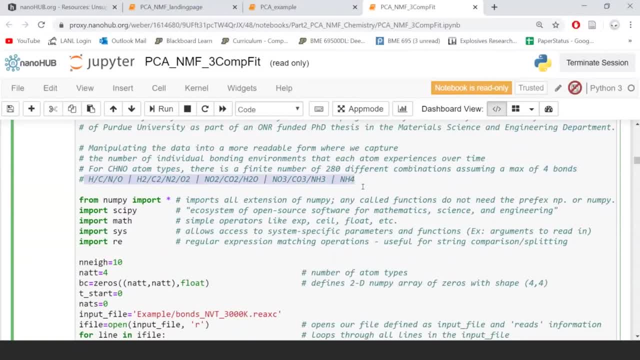 variables, But of course, as I stated, you can do PCA on n dimensions. So we're going to go over this toy example, where we're only going to address two input variables, But of course, as I stated, you can do PCA on n dimensions. 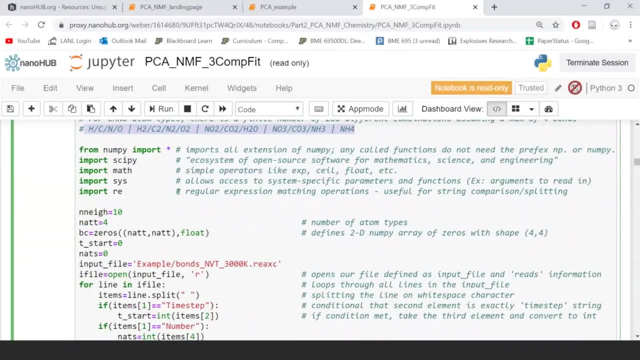 So we're going to go over this toy example where we're only going to address two input variables. But of course, as I stated, you can do PCA on n dimensions. So we're going to go over this toy example where we're only going to address two input. 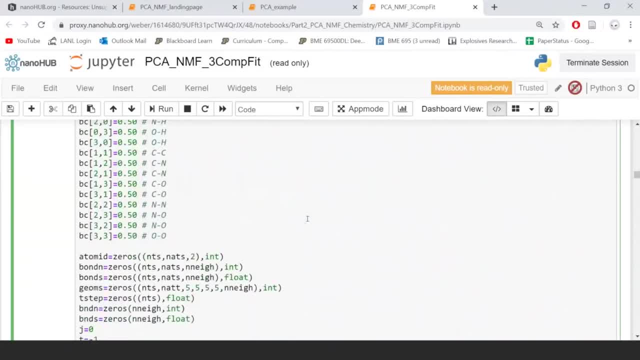 variables, But of course, as I stated, you can do PCA on n dimensions. So we're going to go over this toy example, where we're only going to address two input variables, But of course, as I stated, you can do PCA on n dimensions. 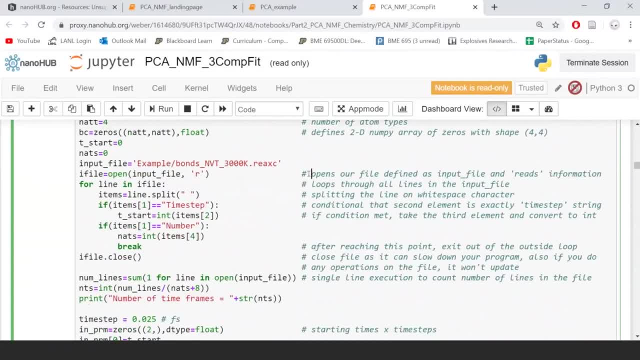 So we're going to go over this toy example where we're only going to address two input variables. But of course, as I stated, you can do PCA on n dimensions. So we're going to go over this toy example where we're only going to address two input. 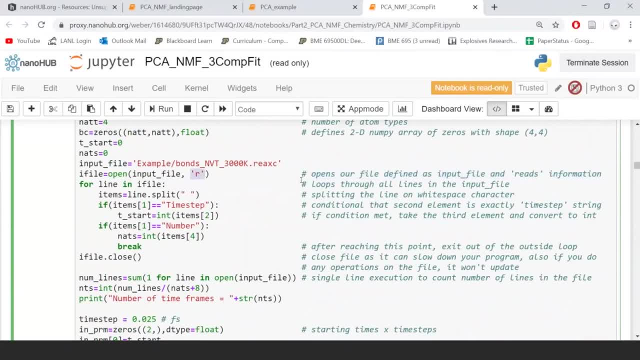 variables, But of course, as I stated, you can do PCA on n dimensions. So we're going to go over this toy example, where we're only going to address two input variables, But of course, as I stated, you can do PCA on n dimensions. 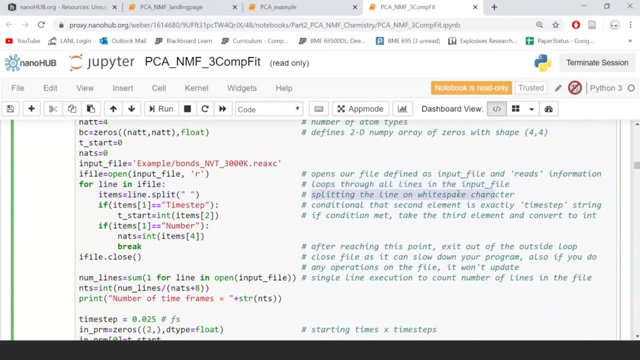 So we're going to go over this toy example where we're only going to address two input variables. But of course, as I stated, you can do PCA on n dimensions. So we're going to go over this toy example where we're only going to address two input. 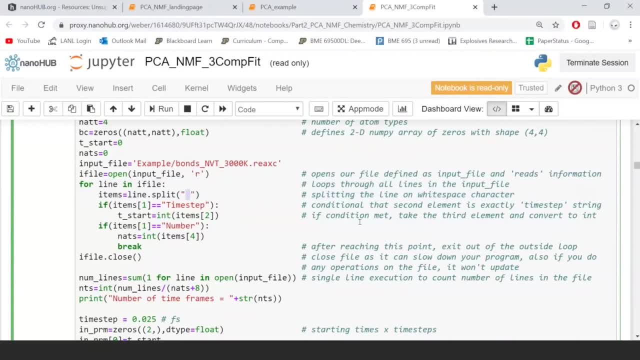 variables, But of course, as I stated, you can do PCA on n dimensions. So we're going to go over this toy example, where we're only going to address two input variables, But of course, as I stated, you can do PCA on n dimensions. 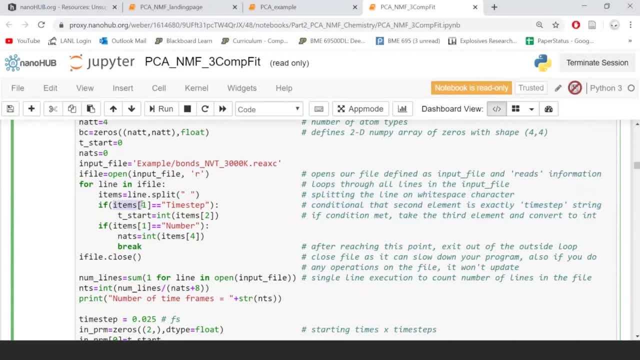 So we're going to go over this toy example where we're only going to address two input variables. But of course, as I stated, you can do PCA on n dimensions. So we're going to go over this toy example where we're only going to address two input. 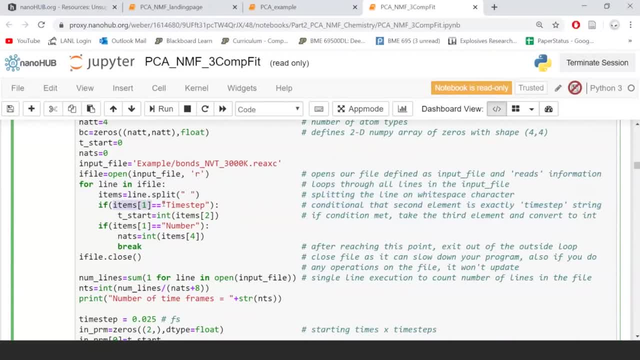 variables, But of course, as I stated, you can do PCA on n dimensions. So we're going to go over this toy example, where we're only going to address two input variables, But of course, as I stated, you can do PCA on n dimensions. 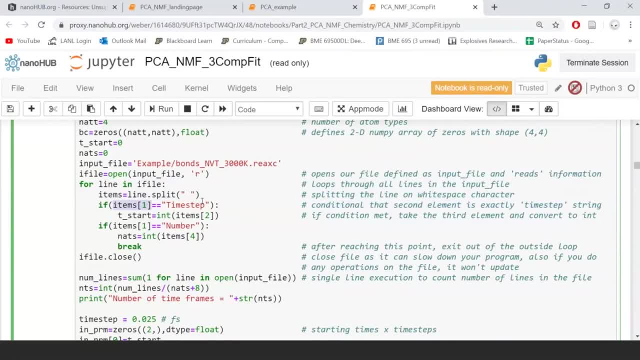 So we're going to go over this toy example where we're only going to address two input variables. But of course, as I stated, you can do PCA on n dimensions. So we're going to go over this toy example where we're only going to address two input. 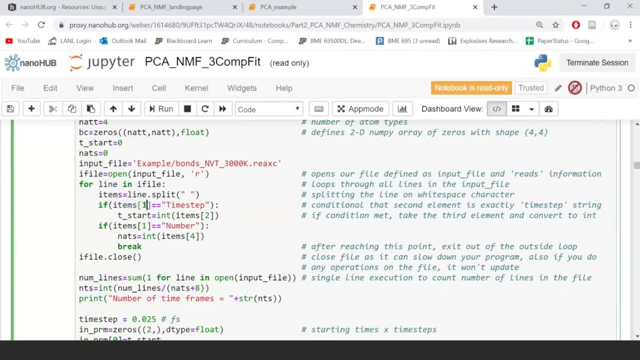 variables, But of course, as I stated, you can do PCA on n dimensions. So we're going to go over this toy example, where we're only going to address two input variables, But of course, as I stated, you can do PCA on n dimensions. 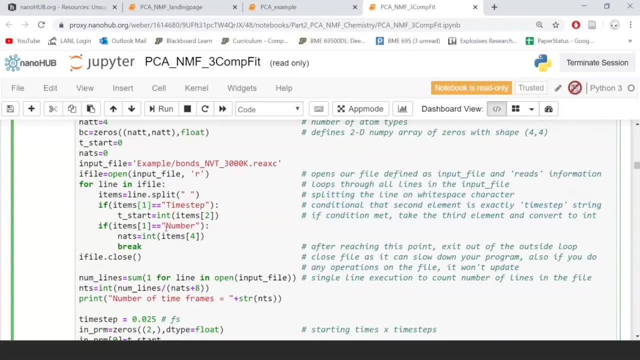 So we're going to go over this toy example where we're only going to address two input variables. But of course, as I stated, you can do PCA on n dimensions. So we're going to go over this toy example where we're only going to address two input. 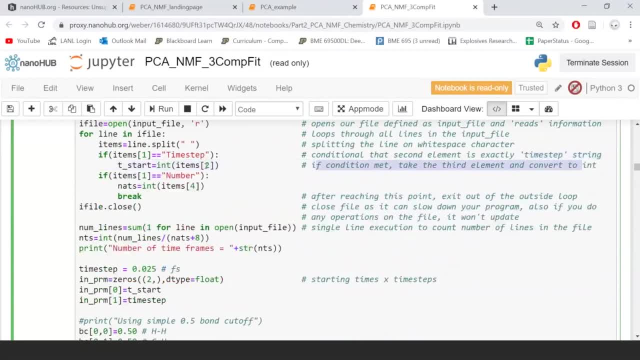 variables, But of course, as I stated, you can do PCA on n dimensions. So we're going to go over this toy example, where we're only going to address two input variables, But of course, as I stated, you can do PCA on n dimensions. 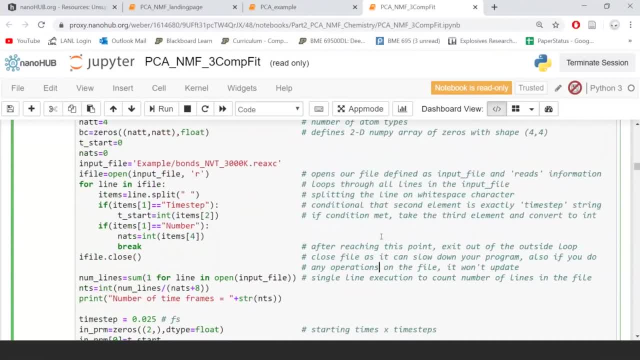 So we're going to go over this toy example where we're only going to address two input variables. But of course, as I stated, you can do PCA on n dimensions. So we're going to go over this toy example where we're only going to address two input. 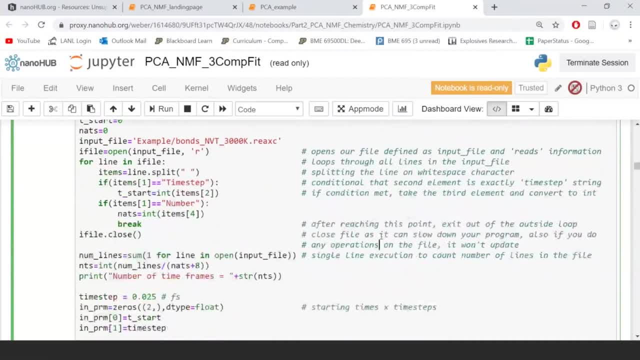 variables, But of course, as I stated, you can do PCA on n dimensions. So we're going to go over this toy example, where we're only going to address two input variables, But of course, as I stated, you can do PCA on n dimensions. 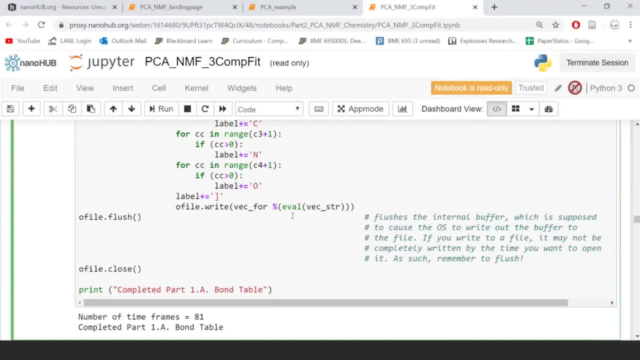 So we're going to go over this toy example where we're only going to address two input variables. But of course, as I stated, you can do PCA on n dimensions. So we're going to go over this toy example where we're only going to address two input. 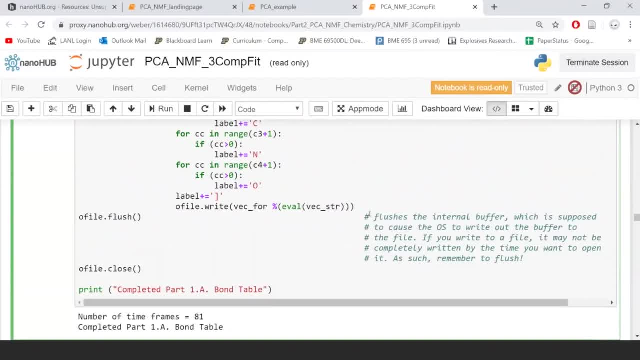 variables, But of course, as I stated, you can do PCA on n dimensions. So we're going to go over this toy example, where we're only going to address two input variables, But of course, as I stated, you can do PCA on n dimensions. 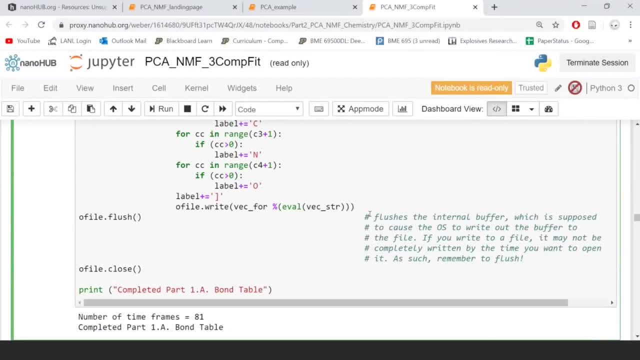 So we're going to go over this toy example where we're only going to address two input variables. But of course, as I stated, you can do PCA on n dimensions. So we're going to go over this toy example where we're only going to address two input. 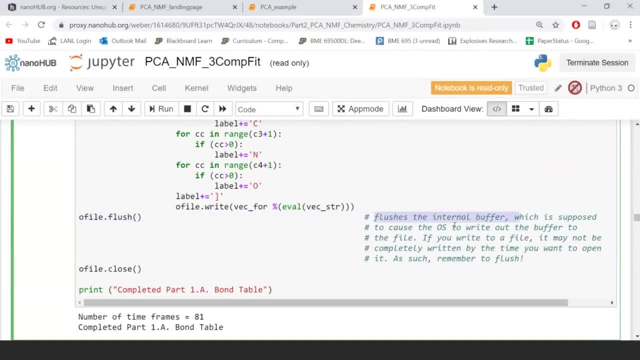 variables, But of course, as I stated, you can do PCA on n dimensions. So we're going to go over this toy example, where we're only going to address two input variables, But of course, as I stated, you can do PCA on n dimensions. 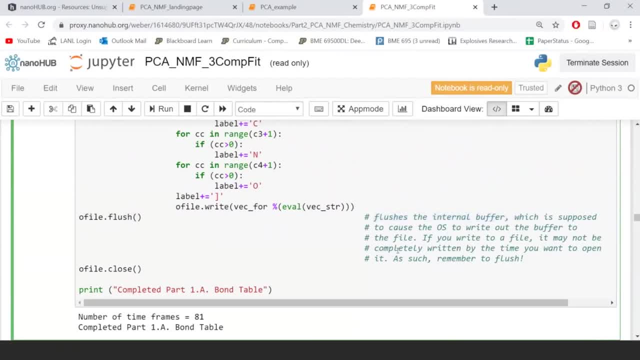 So we're going to go over this toy example where we're only going to address two input variables. But of course, as I stated, you can do PCA on n dimensions. So we're going to go over this toy example where we're only going to address two input. 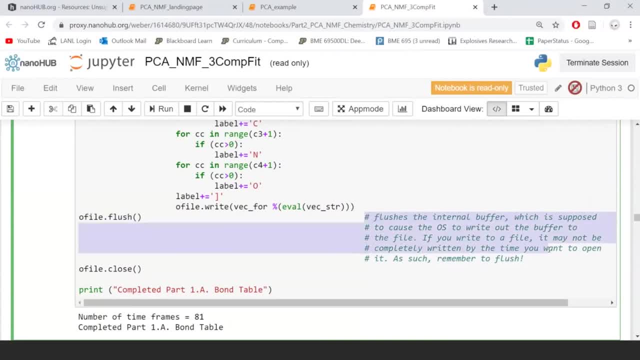 variables, But of course, as I stated, you can do PCA on n dimensions. So we're going to go over this toy example, where we're only going to address two input variables, But of course, as I stated, you can do PCA on n dimensions. 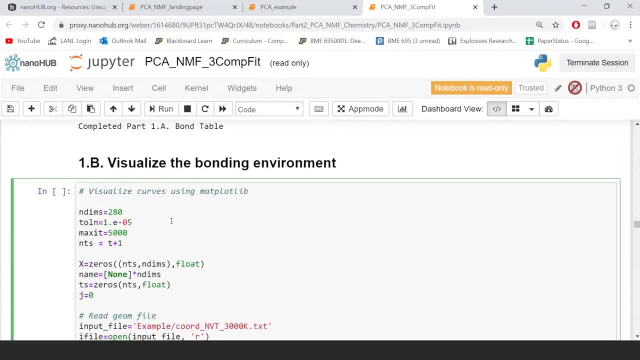 So we're going to go over this toy example where we're only going to address two input variables. But of course, as I stated, you can do PCA on n dimensions. So we're going to go over this toy example where we're only going to address two input. 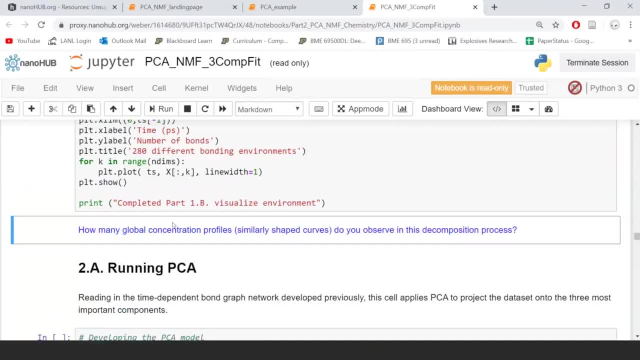 variables, But of course, as I stated, you can do PCA on n dimensions. So we're going to go over this toy example, where we're only going to address two input variables, But of course, as I stated, you can do PCA on n dimensions. 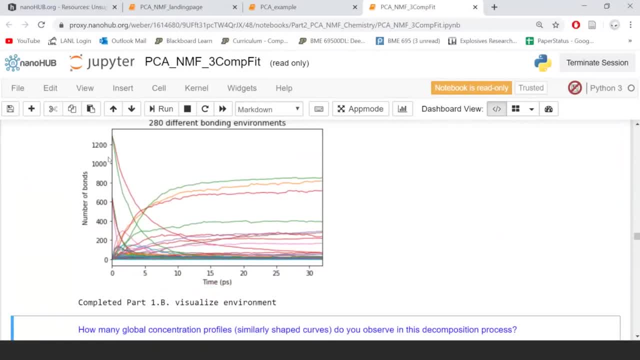 So we're going to go over this toy example where we're only going to address two input variables. But of course, as I stated, you can do PCA on n dimensions. So we're going to go over this toy example where we're only going to address two input. 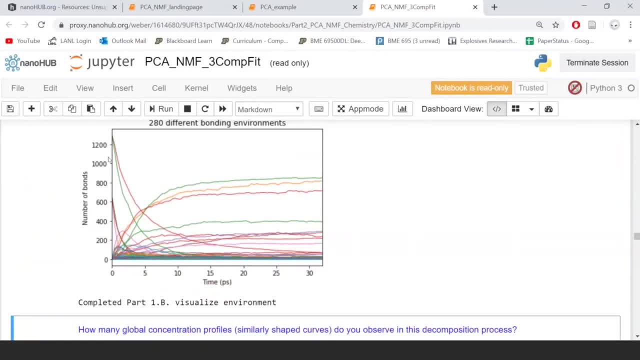 variables, But of course, as I stated, you can do PCA on n dimensions. So we're going to go over this toy example, where we're only going to address two input variables, But of course, as I stated, you can do PCA on n dimensions. 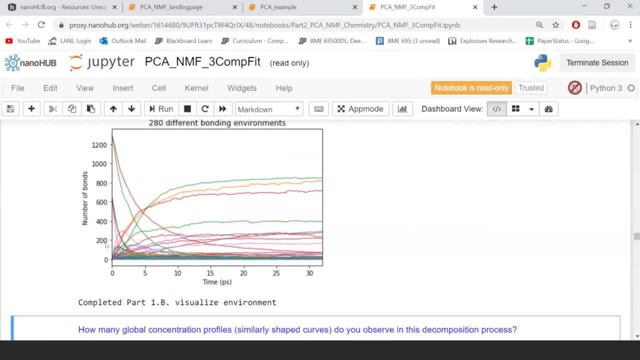 So we're going to go over this toy example where we're only going to address two input variables. But of course, as I stated, you can do PCA on n dimensions. So we're going to go over this toy example where we're only going to address two input. 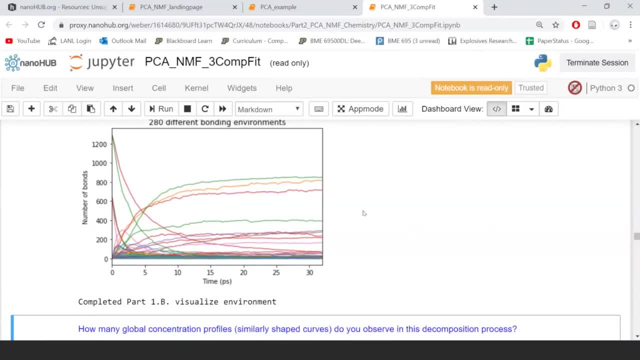 variables, But of course, as I stated, you can do PCA on n dimensions. So we're going to go over this toy example, where we're only going to address two input variables, But of course, as I stated, you can do PCA on n dimensions. 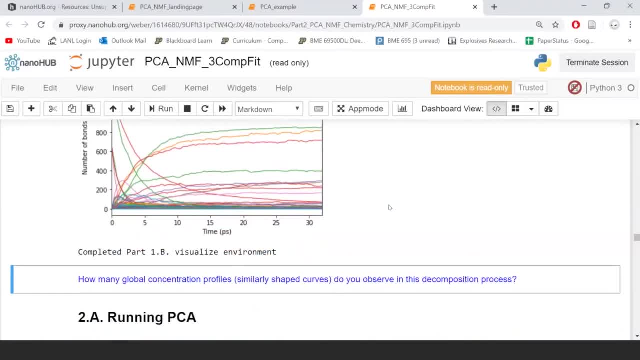 So we're going to go over this toy example where we're only going to address two input variables. But of course, as I stated, you can do PCA on n dimensions. So we're going to go over this toy example where we're only going to address two input. 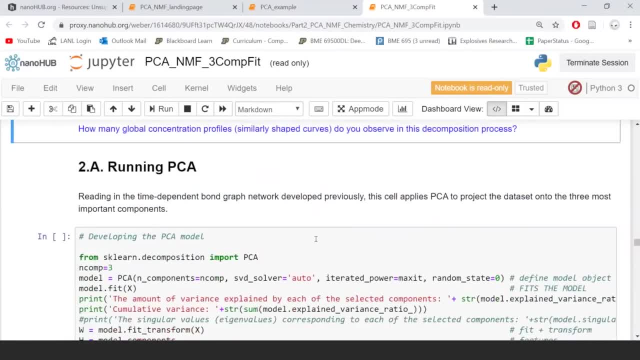 variables, But of course, as I stated, you can do PCA on n dimensions. So we're going to go over this toy example, where we're only going to address two input variables, But of course, as I stated, you can do PCA on n dimensions. 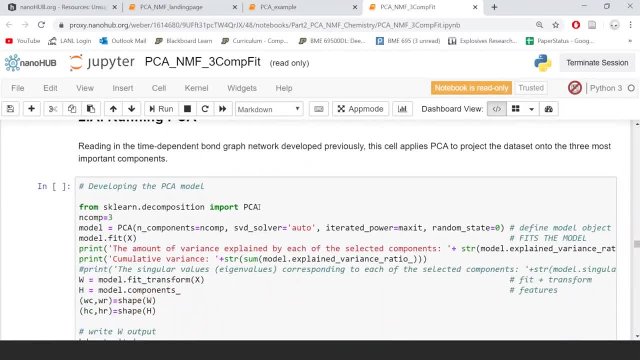 So we're going to go over this toy example where we're only going to address two input variables. But of course, as I stated, you can do PCA on n dimensions. So we're going to go over this toy example where we're only going to address two input. 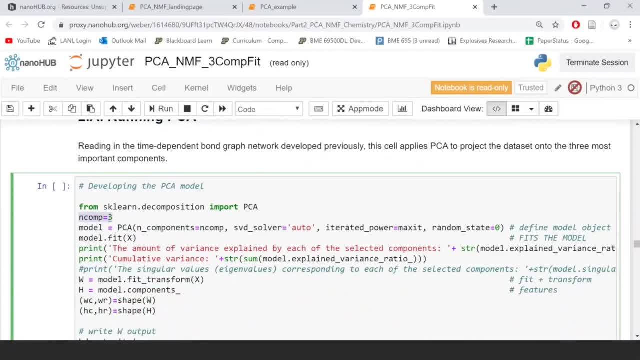 variables, But of course, as I stated, you can do PCA on n dimensions. So we're going to go over this toy example, where we're only going to address two input variables, But of course, as I stated, you can do PCA on n dimensions. 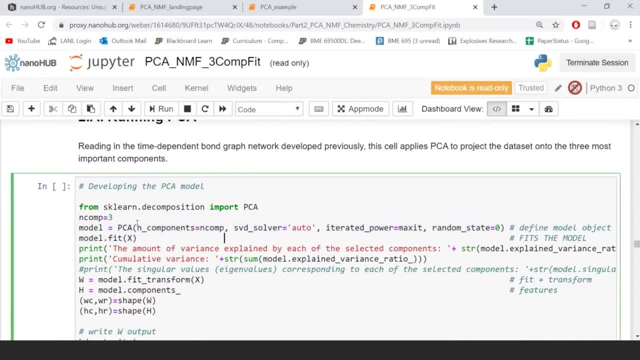 So we're going to go over this toy example where we're only going to address two input variables. But of course, as I stated, you can do PCA on n dimensions. So we're going to go over this toy example where we're only going to address two input. 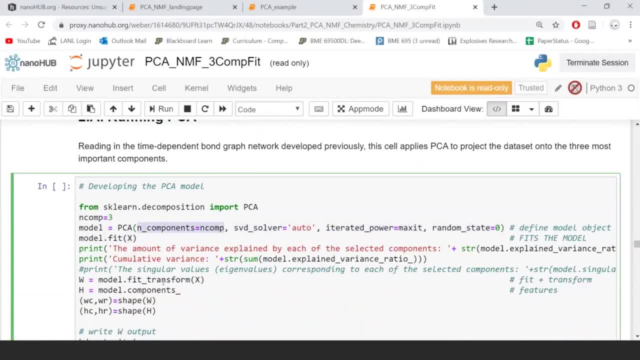 variables, But of course, as I stated, you can do PCA on n dimensions. So we're going to go over this toy example, where we're only going to address two input variables, But of course, as I stated, you can do PCA on n dimensions. 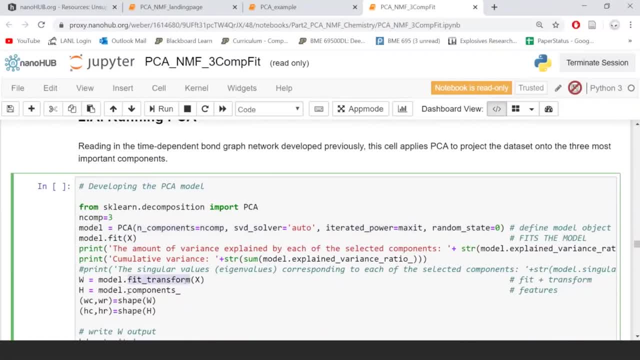 So we're going to go over this toy example where we're only going to address two input variables. But of course, as I stated, you can do PCA on n dimensions. So we're going to go over this toy example where we're only going to address two input. 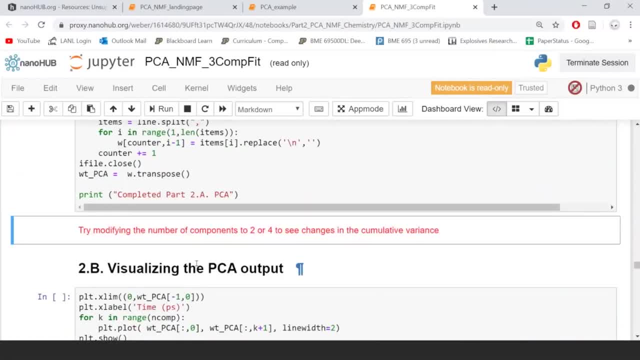 variables, But of course, as I stated, you can do PCA on n dimensions. So we're going to go over this toy example, where we're only going to address two input variables, But of course, as I stated, you can do PCA on n dimensions. 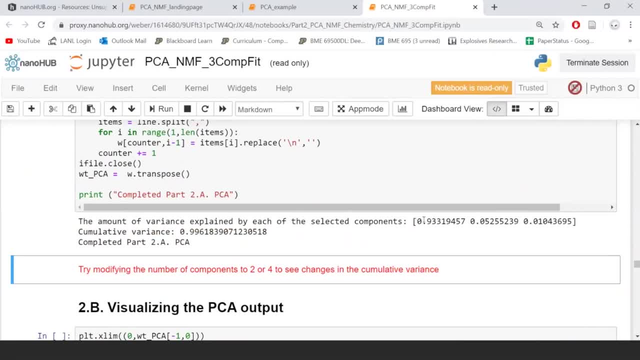 So we're going to go over this toy example where we're only going to address two input variables. But of course, as I stated, you can do PCA on n dimensions. So we're going to go over this toy example where we're only going to address two input. 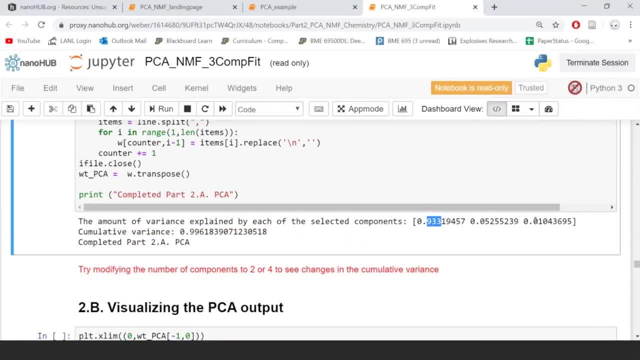 variables, But of course, as I stated, you can do PCA on n dimensions. So we're going to go over this toy example, where we're only going to address two input variables, But of course, as I stated, you can do PCA on n dimensions. 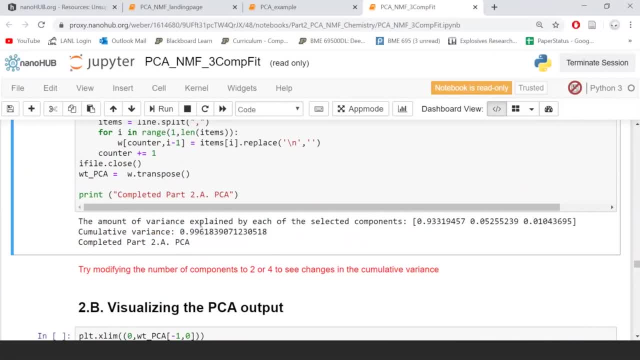 So we're going to go over this toy example where we're only going to address two input variables. But of course, as I stated, you can do PCA on n dimensions. So we're going to go over this toy example where we're only going to address two input. 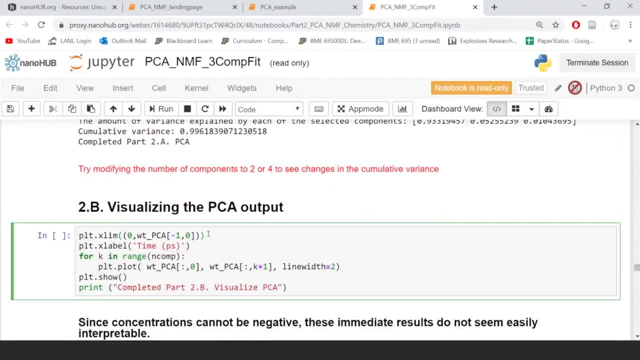 variables, But of course, as I stated, you can do PCA on n dimensions. So we're going to go over this toy example, where we're only going to address two input variables, But of course, as I stated, you can do PCA on n dimensions. 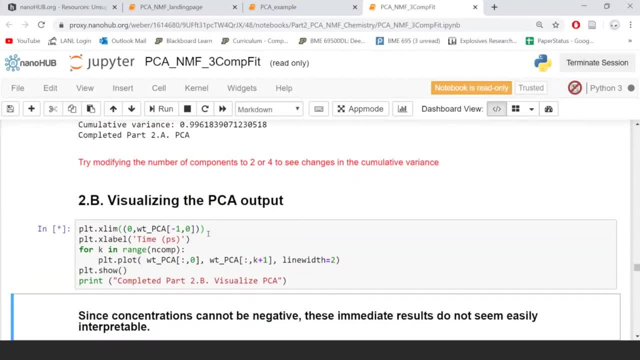 So we're going to go over this toy example where we're only going to address two input variables. But of course, as I stated, you can do PCA on n dimensions. So we're going to go over this toy example where we're only going to address two input. 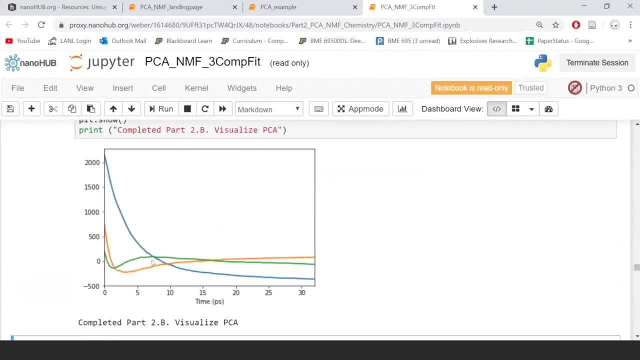 variables, But of course, as I stated, you can do PCA on n dimensions. So we're going to go over this toy example, where we're only going to address two input variables, But of course, as I stated, you can do PCA on n dimensions. 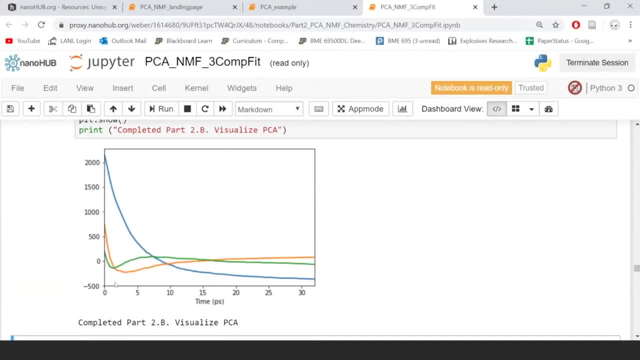 So we're going to go over this toy example where we're only going to address two input variables. But of course, as I stated, you can do PCA on n dimensions. So we're going to go over this toy example where we're only going to address two input. 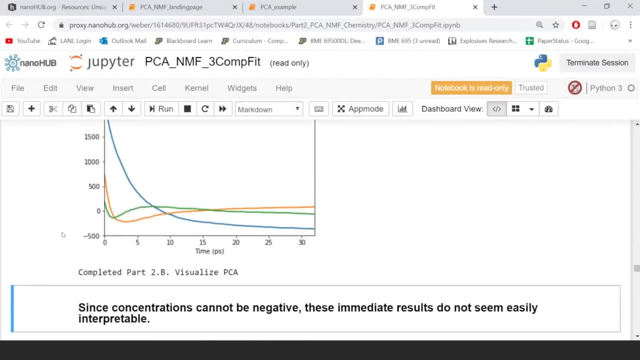 variables, But of course, as I stated, you can do PCA on n dimensions. So we're going to go over this toy example, where we're only going to address two input variables, But of course, as I stated, you can do PCA on n dimensions. 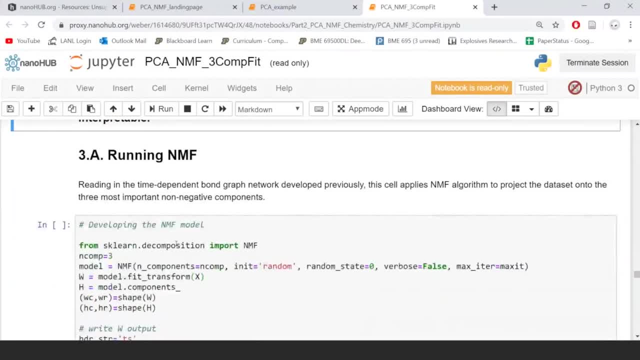 So we're going to go over this toy example where we're only going to address two input variables. But of course, as I stated, you can do PCA on n dimensions. So we're going to go over this toy example where we're only going to address two input. 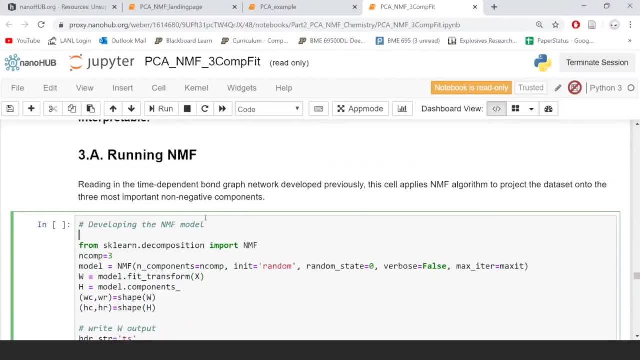 variables, But of course, as I stated, you can do PCA on n dimensions. So we're going to go over this toy example, where we're only going to address two input variables, But of course, as I stated, you can do PCA on n dimensions. 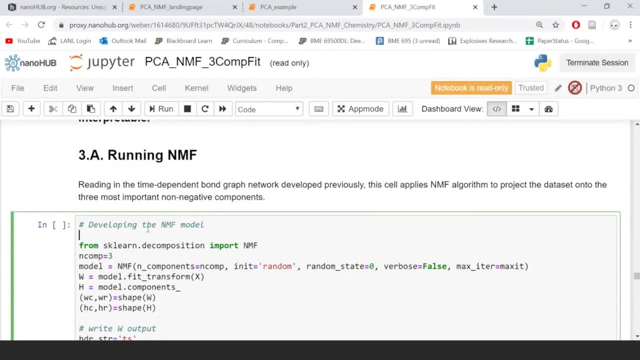 So we're going to go over this toy example where we're only going to address two input variables. But of course, as I stated, you can do PCA on n dimensions. So we're going to go over this toy example where we're only going to address two input. 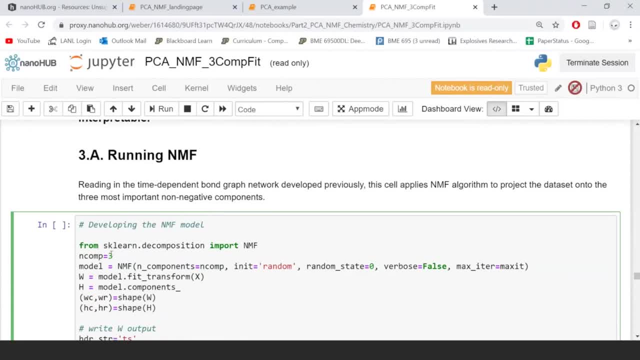 variables, But of course, as I stated, you can do PCA on n dimensions. So we're going to go over this toy example, where we're only going to address two input variables, But of course, as I stated, you can do PCA on n dimensions. 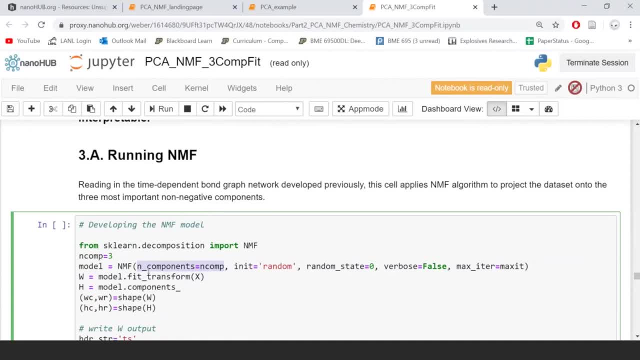 So we're going to go over this toy example where we're only going to address two input variables. But of course, as I stated, you can do PCA on n dimensions. So we're going to go over this toy example where we're only going to address two input. 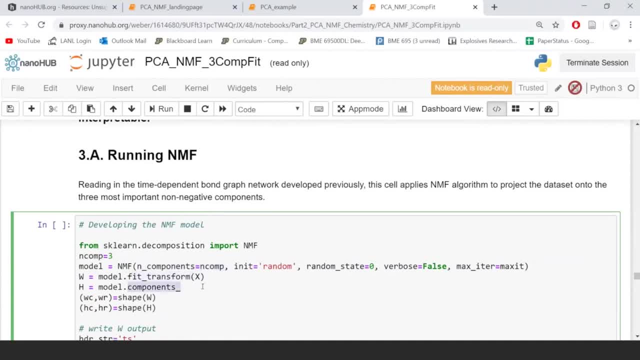 variables, But of course, as I stated, you can do PCA on n dimensions. So we're going to go over this toy example, where we're only going to address two input variables, But of course, as I stated, you can do PCA on n dimensions. 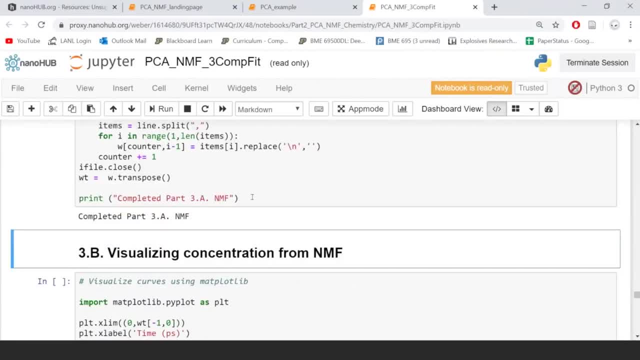 So we're going to go over this toy example where we're only going to address two input variables. But of course, as I stated, you can do PCA on n dimensions. So we're going to go over this toy example where we're only going to address two input. 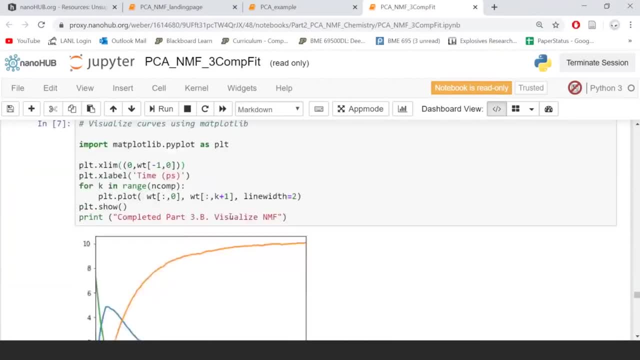 variables, But of course, as I stated, you can do PCA on n dimensions. So we're going to go over this toy example, where we're only going to address two input variables, But of course, as I stated, you can do PCA on n dimensions. 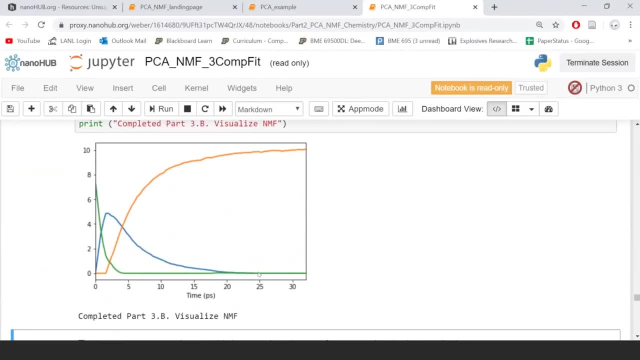 So we're going to go over this toy example where we're only going to address two input variables. But of course, as I stated, you can do PCA on n dimensions. So we're going to go over this toy example where we're only going to address two input. 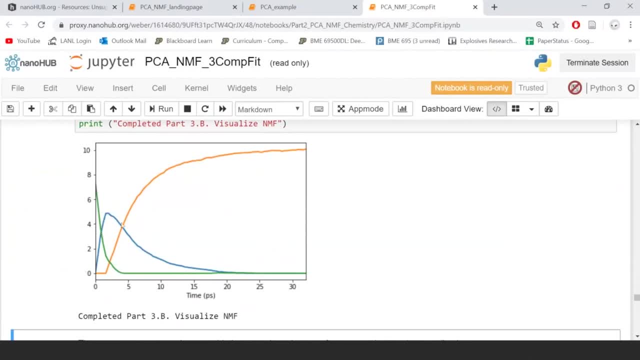 variables, But of course, as I stated, you can do PCA on n dimensions. So we're going to go over this toy example, where we're only going to address two input variables, But of course, as I stated, you can do PCA on n dimensions. 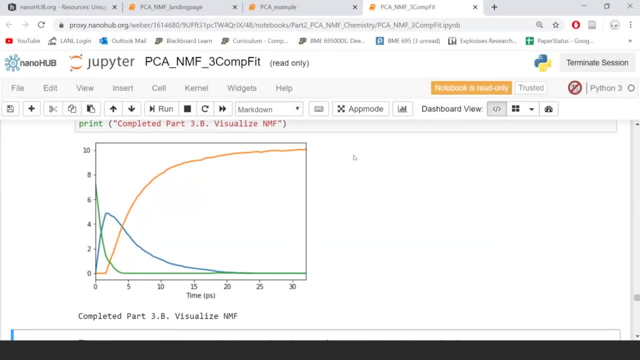 So we're going to go over this toy example where we're only going to address two input variables. But of course, as I stated, you can do PCA on n dimensions. So we're going to go over this toy example where we're only going to address two input. 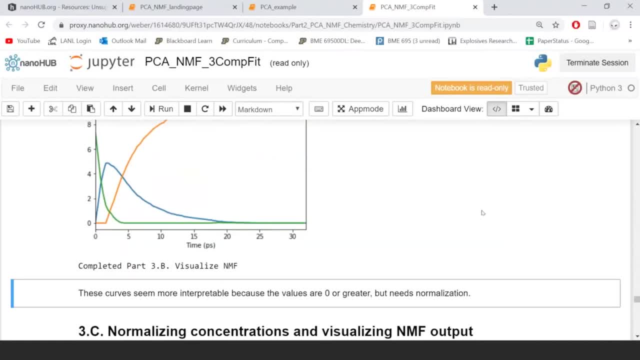 variables, But of course, as I stated, you can do PCA on n dimensions. So we're going to go over this toy example, where we're only going to address two input variables, But of course, as I stated, you can do PCA on n dimensions. 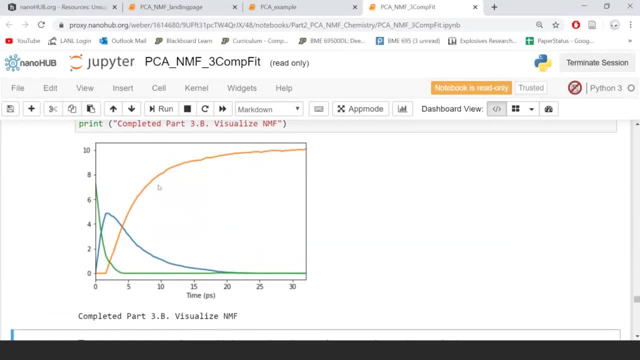 So we're going to go over this toy example where we're only going to address two input variables. But of course, as I stated, you can do PCA on n dimensions. So we're going to go over this toy example where we're only going to address two input. 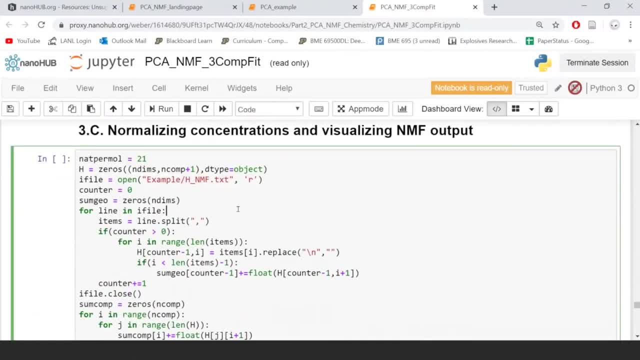 variables, But of course, as I stated, you can do PCA on n dimensions. So we're going to go over this toy example, where we're only going to address two input variables, But of course, as I stated, you can do PCA on n dimensions. 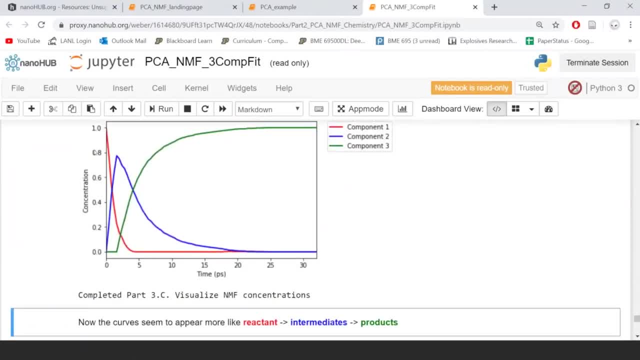 So we're going to go over this toy example where we're only going to address two input variables. But of course, as I stated, you can do PCA on n dimensions. So we're going to go over this toy example where we're only going to address two input. 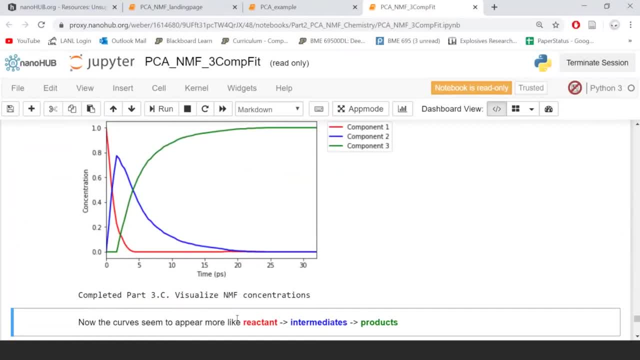 variables, But of course, as I stated, you can do PCA on n dimensions. So we're going to go over this toy example, where we're only going to address two input variables, But of course, as I stated, you can do PCA on n dimensions. 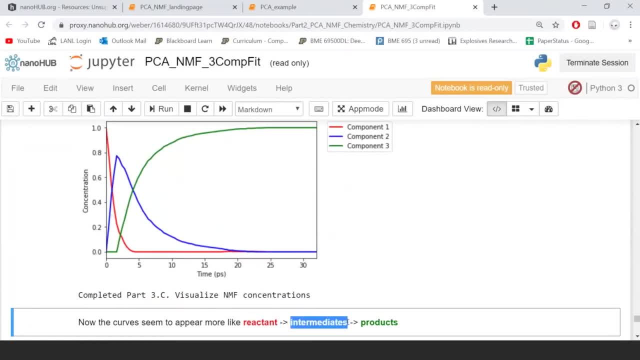 So we're going to go over this toy example where we're only going to address two input variables. But of course, as I stated, you can do PCA on n dimensions. So we're going to go over this toy example where we're only going to address two input. 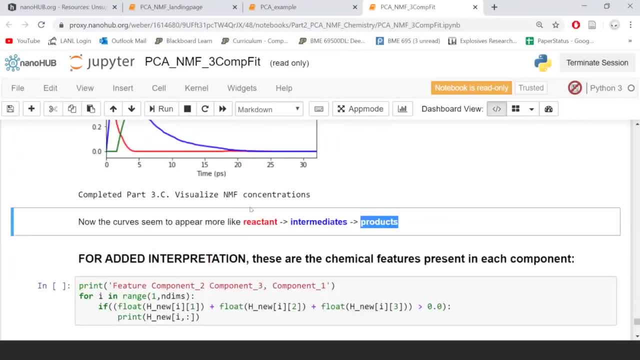 variables, But of course, as I stated, you can do PCA on n dimensions. So we're going to go over this toy example, where we're only going to address two input variables, But of course, as I stated, you can do PCA on n dimensions. 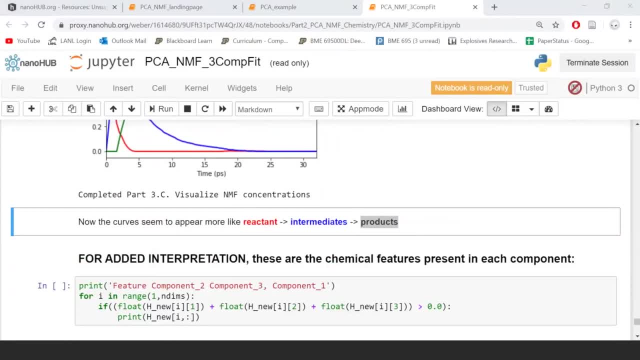 So we're going to go over this toy example where we're only going to address two input variables. But of course, as I stated, you can do PCA on n dimensions. So we're going to go over this toy example where we're only going to address two input. 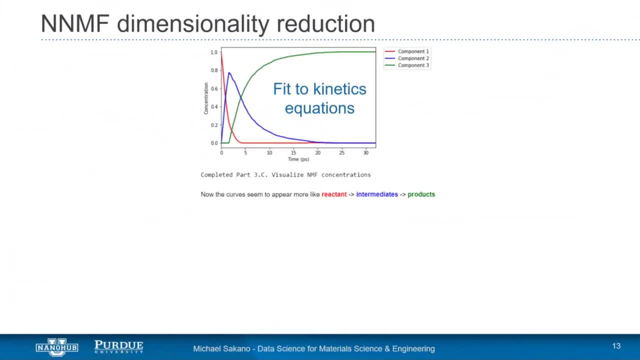 variables, But of course, as I stated, you can do PCA on n dimensions. So we're going to go over this toy example, where we're only going to address two input variables, But of course, as I stated, you can do PCA on n dimensions. 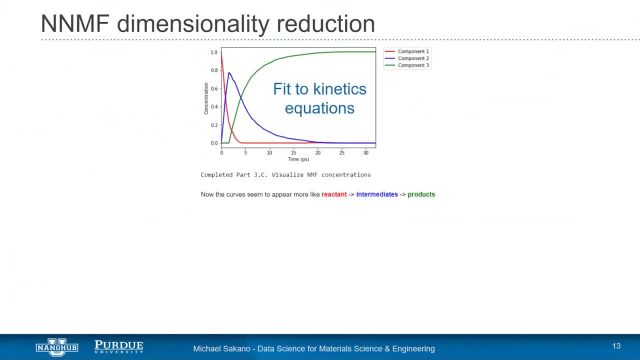 So we're going to go over this toy example where we're only going to address two input variables. But of course, as I stated, you can do PCA on n dimensions. So we're going to go over this toy example where we're only going to address two input. 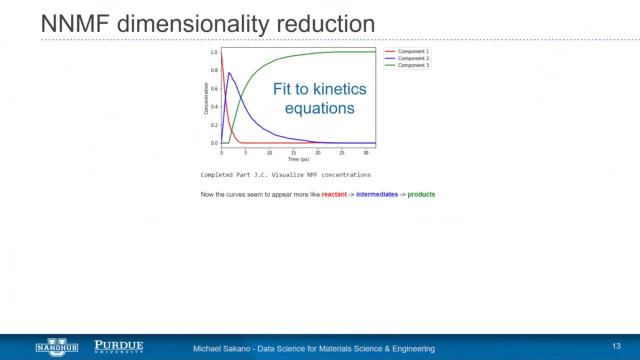 variables, But of course, as I stated, you can do PCA on n dimensions. So we're going to go over this toy example, where we're only going to address two input variables, But of course, as I stated, you can do PCA on n dimensions. 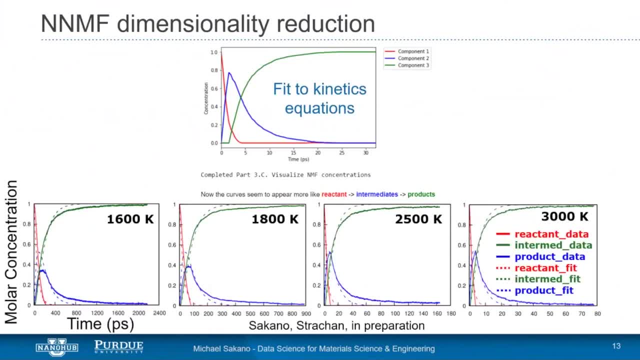 So we're going to go over this toy example where we're only going to address two input variables. But of course, as I stated, you can do PCA on n dimensions. So we're going to go over this toy example where we're only going to address two input. 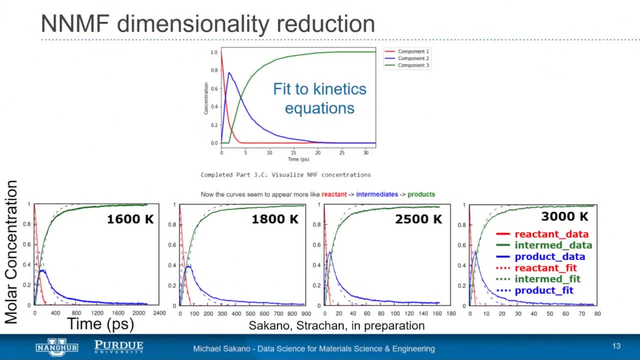 variables, But of course, as I stated, you can do PCA on n dimensions. So we're going to go over this toy example, where we're only going to address two input variables, But of course, as I stated, you can do PCA on n dimensions. 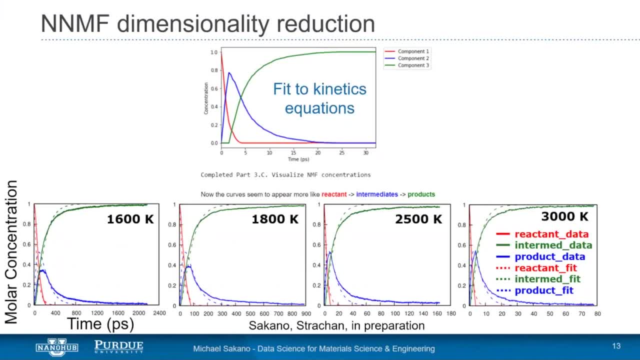 So we're going to go over this toy example where we're only going to address two input variables. But of course, as I stated, you can do PCA on n dimensions. So we're going to go over this toy example where we're only going to address two input. 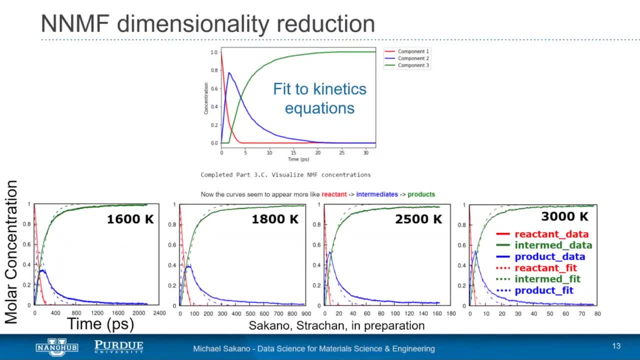 variables, But of course, as I stated, you can do PCA on n dimensions. So we're going to go over this toy example, where we're only going to address two input variables, But of course, as I stated, you can do PCA on n dimensions. 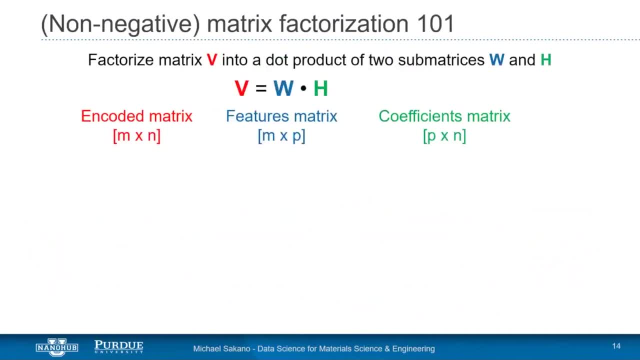 So we're going to go over this toy example where we're only going to address two input variables. But of course, as I stated, you can do PCA on n dimensions. So we're going to go over this toy example where we're only going to address two input. 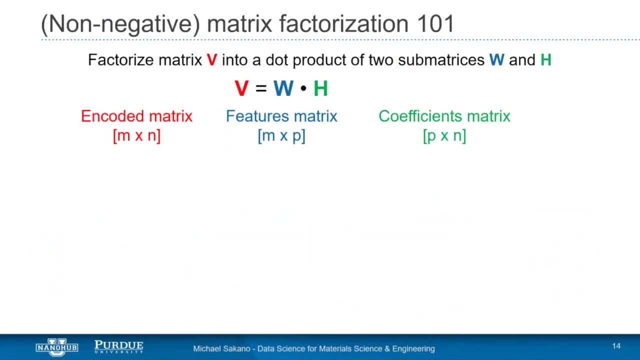 variables, But of course, as I stated, you can do PCA on n dimensions. So we're going to go over this toy example, where we're only going to address two input variables, But of course, as I stated, you can do PCA on n dimensions. 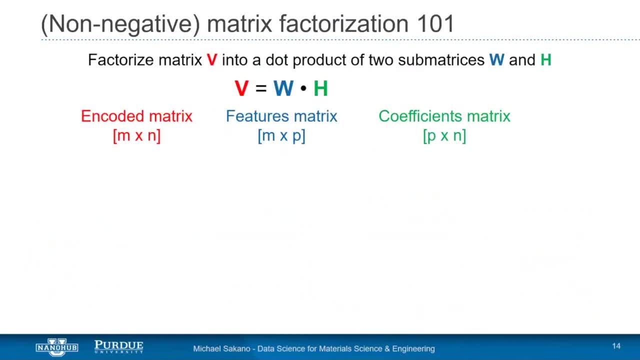 So we're going to go over this toy example where we're only going to address two input variables. But of course, as I stated, you can do PCA on n dimensions. So we're going to go over this toy example where we're only going to address two input. 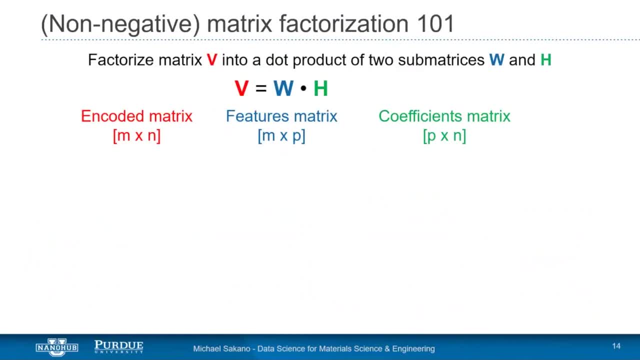 variables, But of course, as I stated, you can do PCA on n dimensions. So we're going to go over this toy example, where we're only going to address two input variables, But of course, as I stated, you can do PCA on n dimensions. 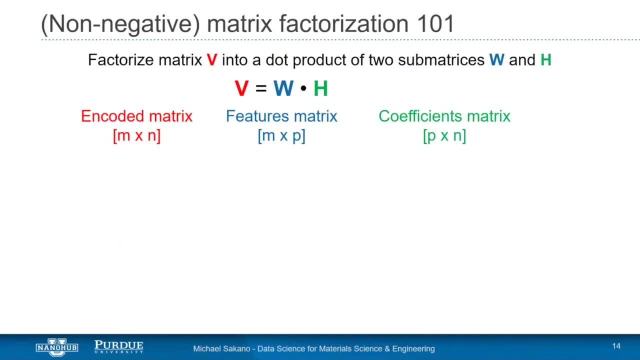 So we're going to go over this toy example where we're only going to address two input variables. But of course, as I stated, you can do PCA on n dimensions. So we're going to go over this toy example where we're only going to address two input. 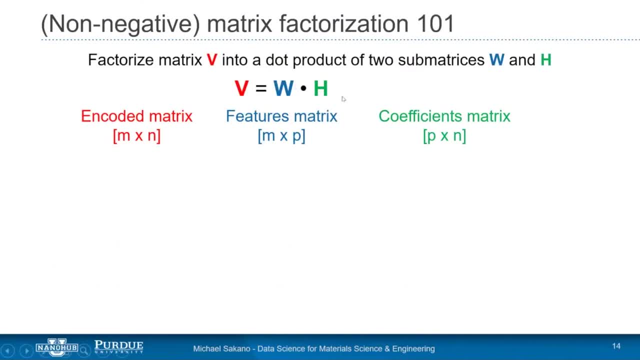 variables, But of course, as I stated, you can do PCA on n dimensions. So we're going to go over this toy example, where we're only going to address two input variables, But of course, as I stated, you can do PCA on n dimensions. 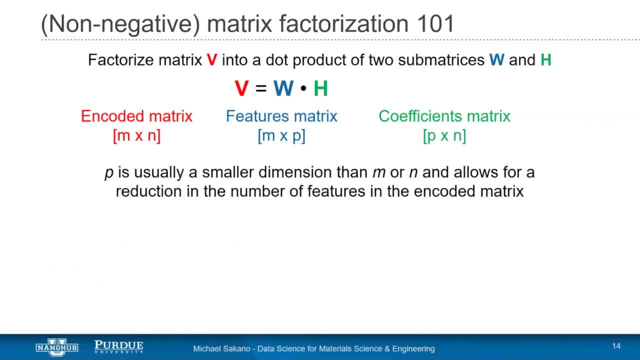 So we're going to go over this toy example where we're only going to address two input variables. But of course, as I stated, you can do PCA on n dimensions. So we're going to go over this toy example where we're only going to address two input. 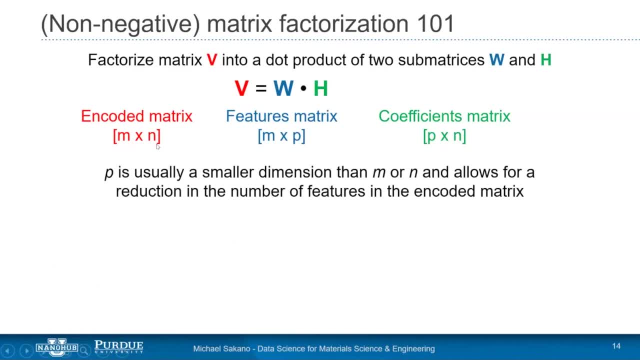 variables, But of course, as I stated, you can do PCA on n dimensions. So we're going to go over this toy example, where we're only going to address two input variables, But of course, as I stated, you can do PCA on n dimensions. 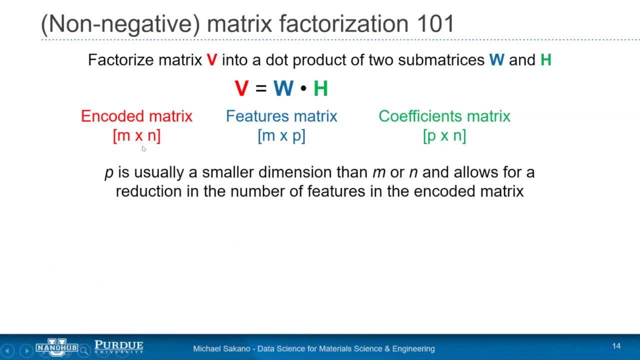 So we're going to go over this toy example where we're only going to address two input variables. But of course, as I stated, you can do PCA on n dimensions. So we're going to go over this toy example where we're only going to address two input. 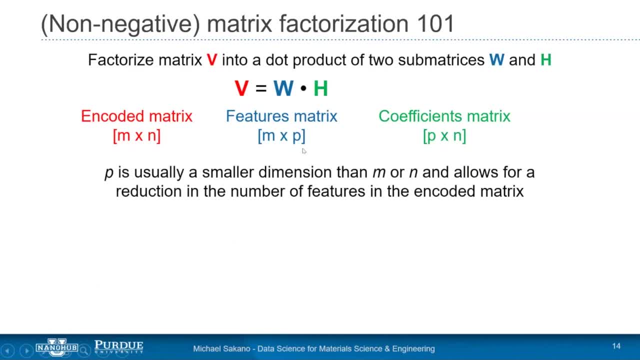 variables, But of course, as I stated, you can do PCA on n dimensions. So we're going to go over this toy example, where we're only going to address two input variables, But of course, as I stated, you can do PCA on n dimensions. 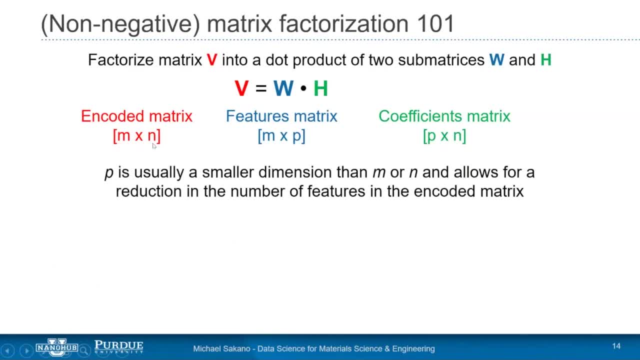 So we're going to go over this toy example where we're only going to address two input variables. But of course, as I stated, you can do PCA on n dimensions. So we're going to go over this toy example where we're only going to address two input. 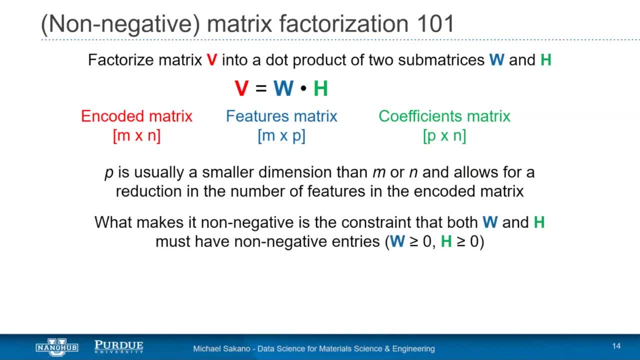 variables, But of course, as I stated, you can do PCA on n dimensions. So we're going to go over this toy example, where we're only going to address two input variables, But of course, as I stated, you can do PCA on n dimensions. 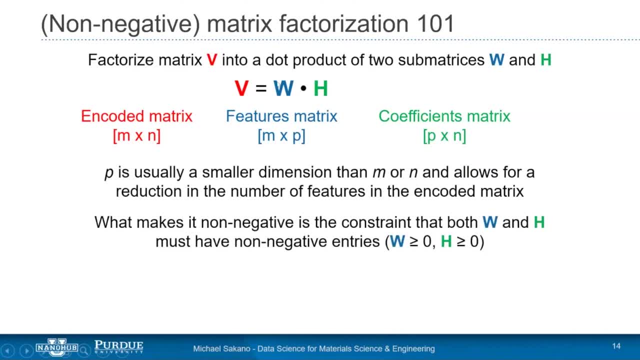 So we're going to go over this toy example where we're only going to address two input variables. But of course, as I stated, you can do PCA on n dimensions. So we're going to go over this toy example where we're only going to address two input. 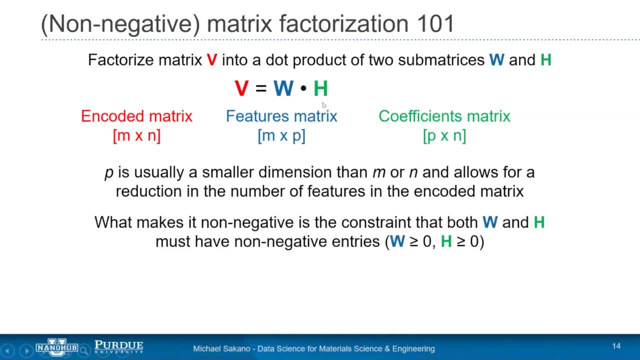 variables, But of course, as I stated, you can do PCA on n dimensions. So we're going to go over this toy example, where we're only going to address two input variables, But of course, as I stated, you can do PCA on n dimensions. 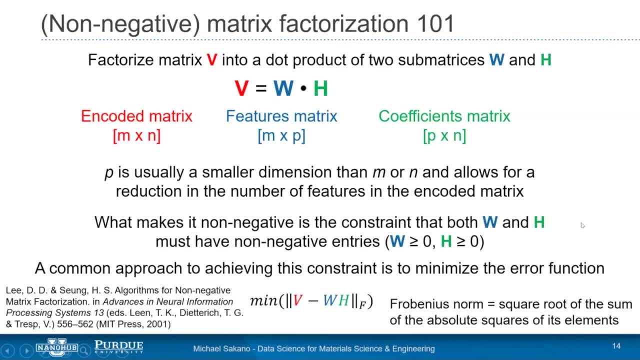 So we're going to go over this toy example where we're only going to address two input variables. But of course, as I stated, you can do PCA on n dimensions. So we're going to go over this toy example where we're only going to address two input. 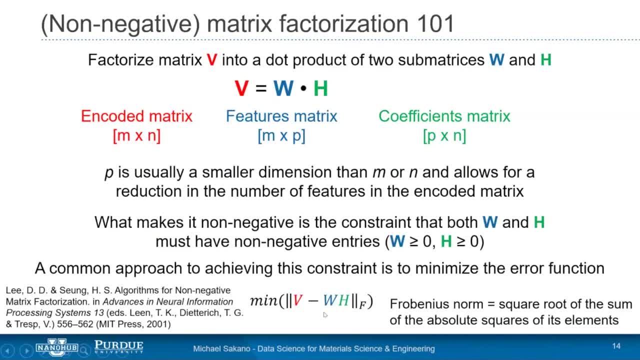 variables, But of course, as I stated, you can do PCA on n dimensions. So we're going to go over this toy example, where we're only going to address two input variables, But of course, as I stated, you can do PCA on n dimensions. 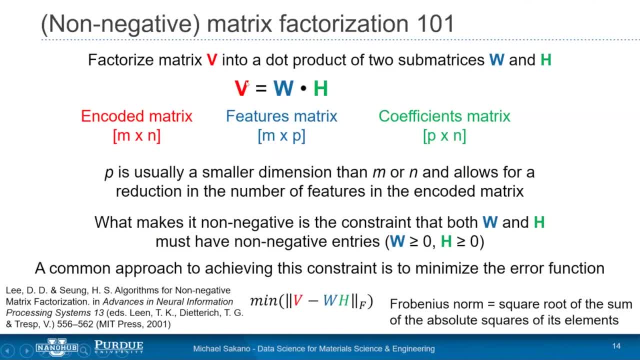 So we're going to go over this toy example where we're only going to address two input variables. But of course, as I stated, you can do PCA on n dimensions. So we're going to go over this toy example where we're only going to address two input. 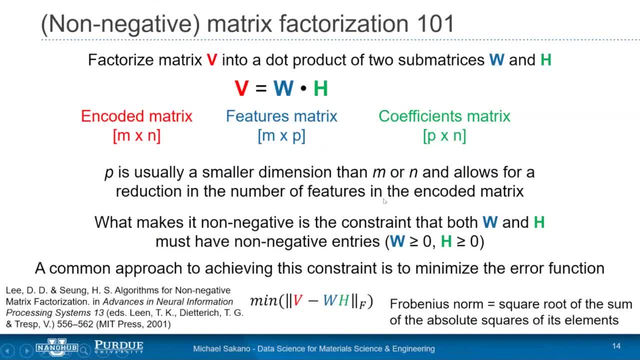 variables, But of course, as I stated, you can do PCA on n dimensions. So we're going to go over this toy example, where we're only going to address two input variables, But of course, as I stated, you can do PCA on n dimensions. 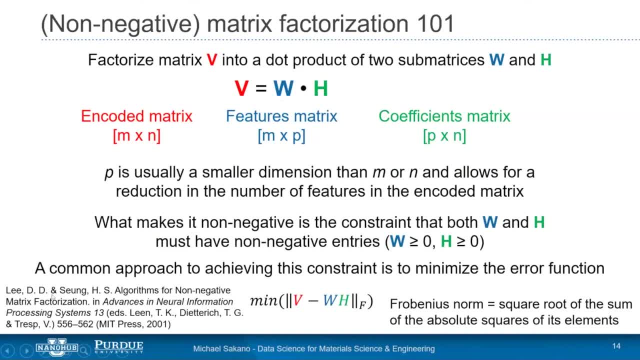 So we're going to go over this toy example where we're only going to address two input variables. But of course, as I stated, you can do PCA on n dimensions. So we're going to go over this toy example where we're only going to address two input. 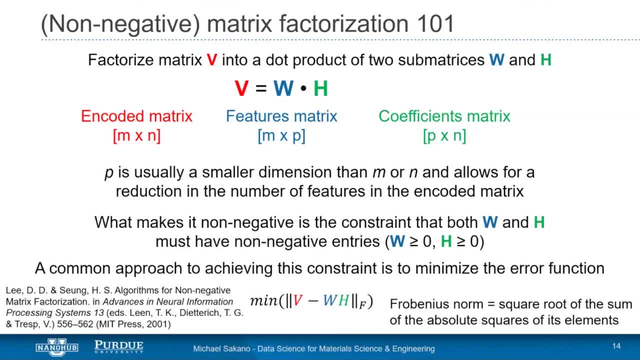 variables, But of course, as I stated, you can do PCA on n dimensions. So we're going to go over this toy example, where we're only going to address two input variables, But of course, as I stated, you can do PCA on n dimensions. 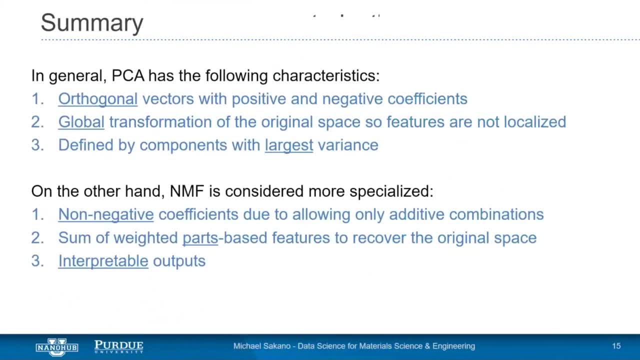 So we're going to go over this toy example where we're only going to address two input variables, But of course, as I stated, you can do PCA on n dimensions, both PCA and NMF. So we've shown that PCA can provide you with both positive and negative. 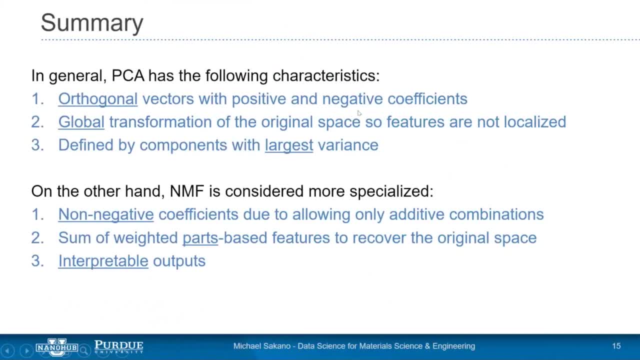 weights- Remember the image where we had faces or features that could be expressed in positive and negative weights- but it ensures that the vectors or the eigenvectors that we obtain are orthogonal to one another. And this is a global transformation, because what you might have noticed in the PCA- 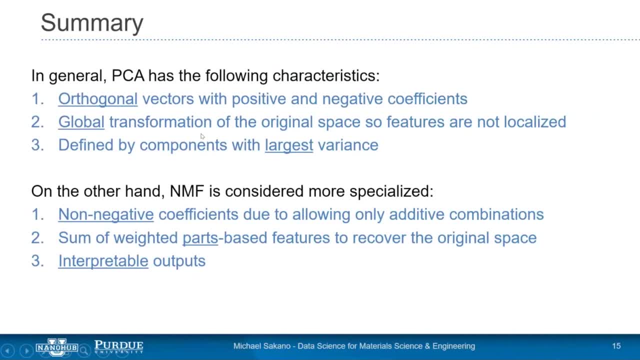 is that some of the eigenvectors we obtain had both faces and noses. It wasn't very localized, it was more of a global transformation of the original space. And the way that PCA does its algorithm is: it defines the number of principal, it defines the principal components as such, that 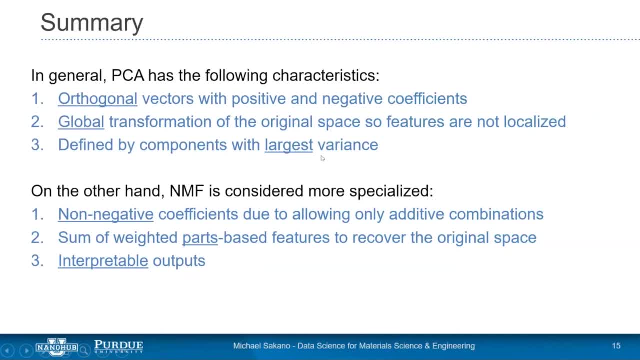 those having the largest variance And when you do a dimension at reduction, you remove the components with that have the least amount of explained variance. On the other hand, NMF is more specialized. as I just stated, We know that the coefficients in the components matrix must have non-negative 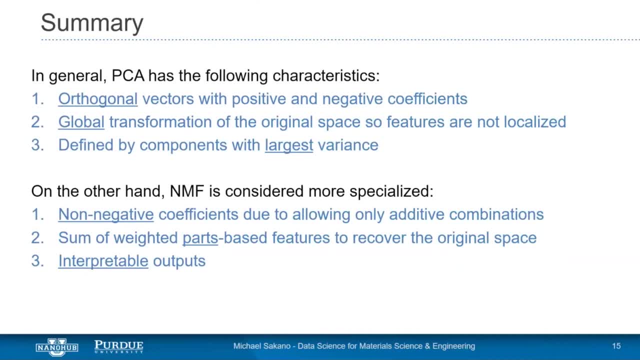 entries, and this is due to its only additive properties, And we also saw in the face example that some of the features were parts-based. We actually were able to extract out only eyebrows or only noses, And so this actually allows our results to be more interpretable in those specific examples. So with that, I'd like to thank. 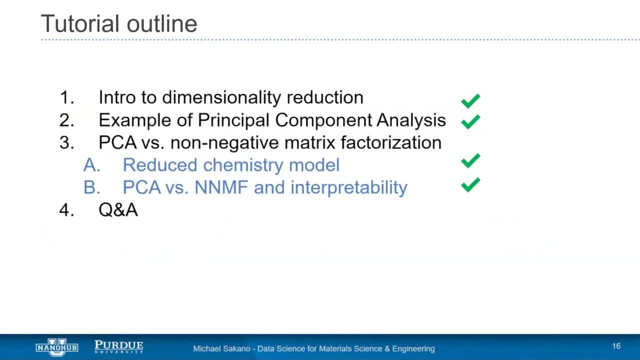 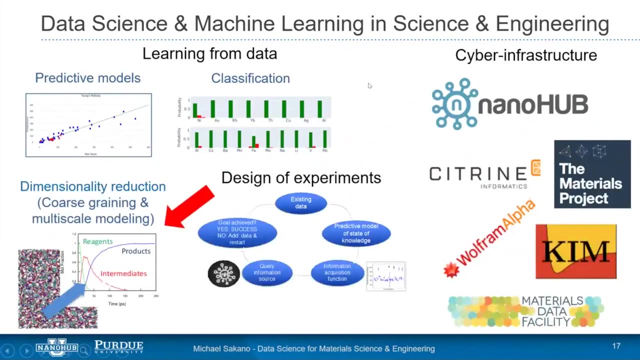 you for your time. Hopefully you understood as we went through the rundown of principal component analysis and non-negative matrix factorization And with that I'd like to reiterate the grand scheme of data science, machine learning and science and engineering. Again, we have cyber infrastructures. 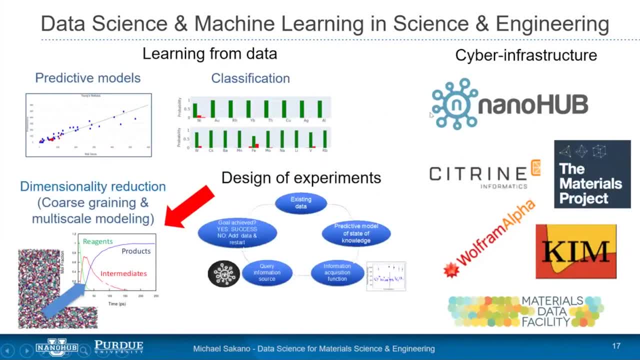 that allow us to learn from a variety of data. We've shown that we can create predictive models and do classification. This session we focused on dimensionality reduction, going from n-dimensional space and reducing our data down to very simple three-dimensional features, And all this is to help guide in the design of experiments. 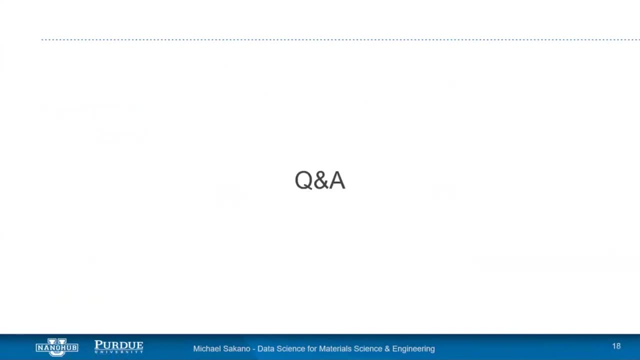 So with that, I'd like to open up the floor to any questions that you may have at this time. Thank you, I'll start with a question. So in your first example, Michael, you were describing PCA with two different components. Yes, So how much of the variance can be explained by the first component? 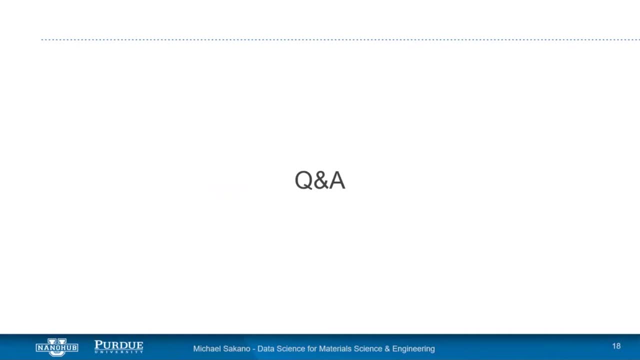 So in PCA we're trying to explain complicated phenomena using simple components. How much can we do with the first component? only for your toy example? Yep, I'll go back to that right now. So, as I explained in the first example, the explained variance will not change if you do this. dimensionality reduction. 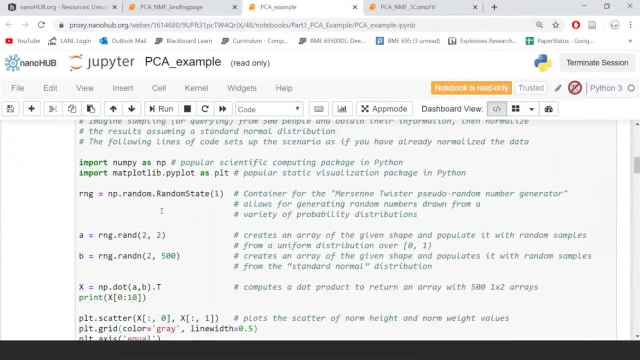 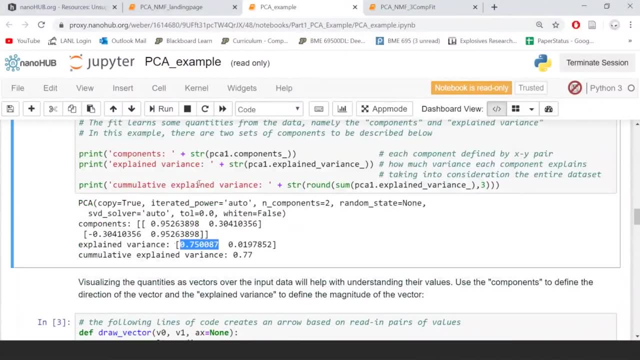 So in this example- let me find it- we're able to explain the first component, alreadyermanial 75% of the variance of the original data space was being explained by the first variance- 75%- And you can see that when we do this, dimensionality reduction- 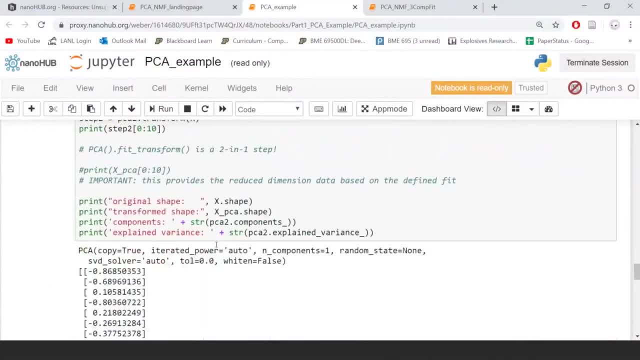 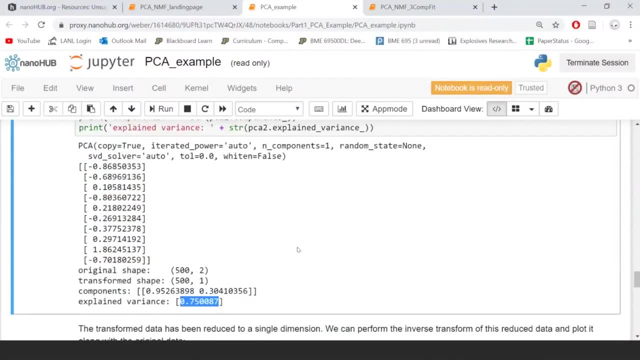 I believe this variable should not change at all, because they were still explaining it by the exact same first principal component. So, to answer your question, we were able to explain 75% of the variance through the first component, and the second one really didn't add much. 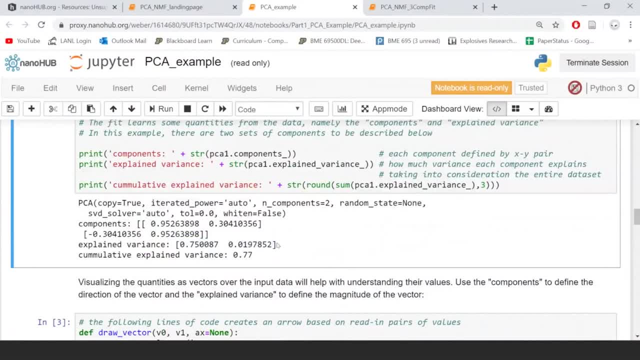 It didn't explain much more variance. So this was an example that we wanted to show. yeah, you can do a dimensionality reduction, going from two components to one component, and you'll still more or less retain the majority of explaining the variance in your data. 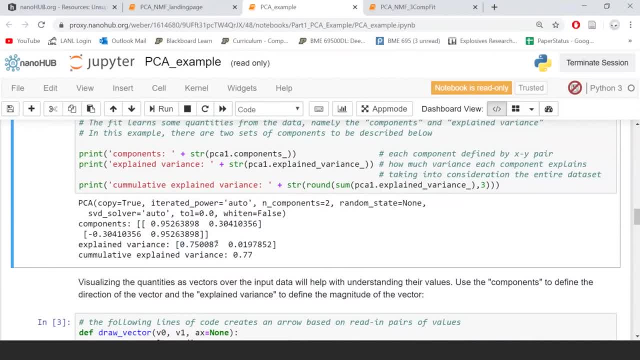 So 75%, Thank you. So I was wondering. can you hear me, Michael? Yes, I was wondering whether these types of techniques of dimensionality reduction could be used in tandem with machine learning. So this could be the first step to reduce your problem. 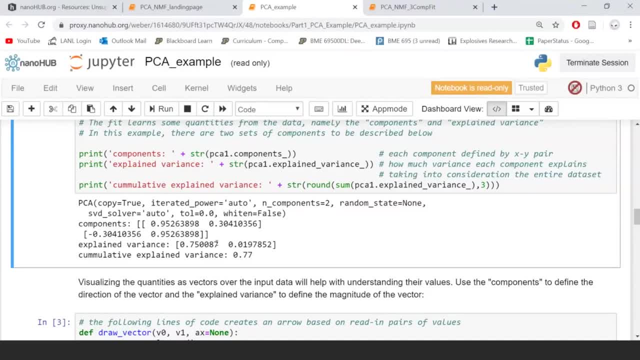 And then you could, for example, use some of the machine learning techniques that Saketh described in the previous presentation. Do you have any comments on that, or, Saketh? I mean, I believe it's all you have to make sure, I think is ensure that you do the correct post-processing. 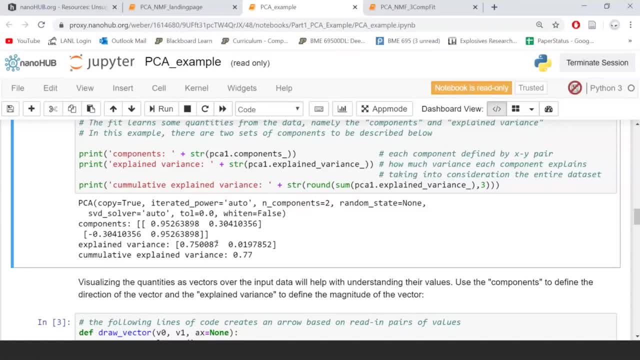 Make sure that you follow along in what you're mapping in on what space. If you're doing dimensionality reduction, make sure you map it back into the original space. Just don't do the fit and say, hey, this is our data. 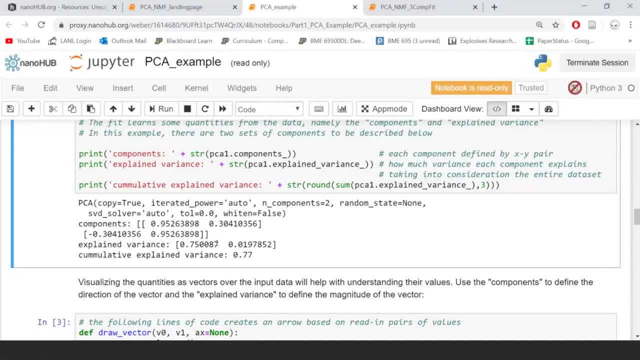 You need to do the fit, inverse transform after you do the fit. But I think there's definitely value in taking the data, taking this, what we've done in our reduced dimensional space and actually moving forward with it. I think I definitely agree that you can do machine learning. 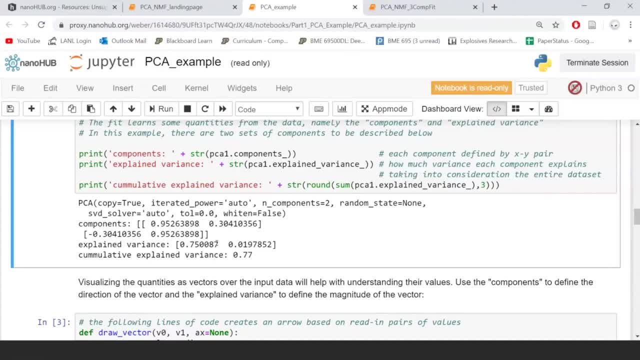 training a neural network with this information. All we were trying to do is remove unnecessary variants, or more or less, we were trying to remove any values that might contain noise in our data set, I believe. So I'm pretty sure you can definitely link this. 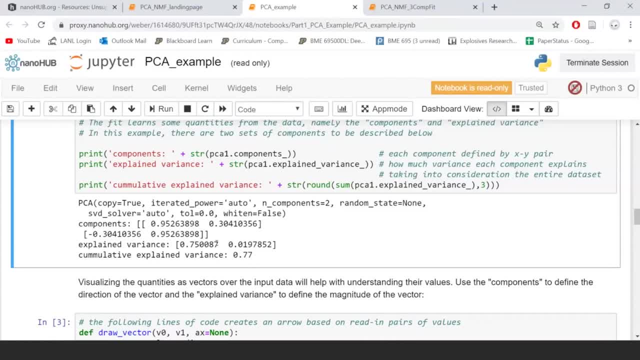 and move it forward in machine learning algorithms. Saketh, Maybe he can provide some input. Yeah, I was just going to say that in the past few years there have been many examples of autoencoders or encoder-decoder- pairs of networks that try to do the same thing. 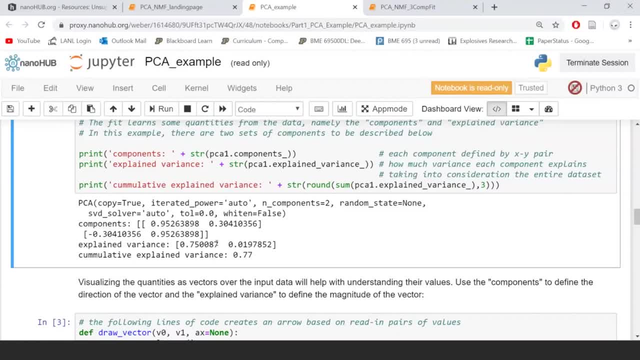 You would have one sort of network that would learn the minimum number of features that you need to then predict the quantity of interest. If you can do the dimensionality reduction using non-negative matrix factorization or PCA, it would just feed in and replace the encoder part. 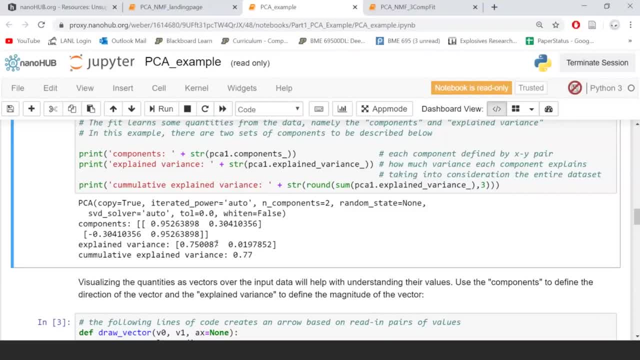 of the encoder-decoder network And then the subsequent part would stay the same. So if you are interested in describing a given material, you can have elemental descriptors. You can have descriptors that comes from DFT calculations And maybe not all of them are necessary. 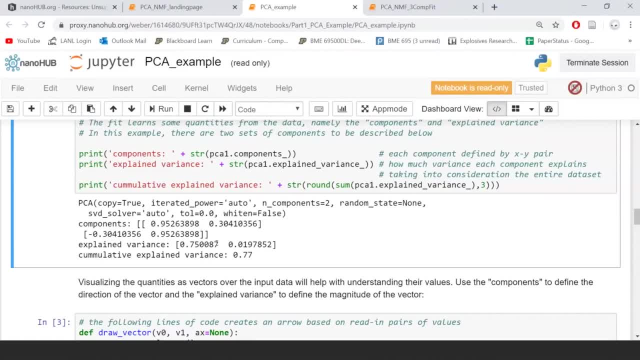 And a technique like this can reduce it down, distill it down to a set of features that you actually need to make predictions of, say conductivity or strength or something like that. Yeah, there are many cases, in almost every engineering or science application, when you have a high dimensional space. 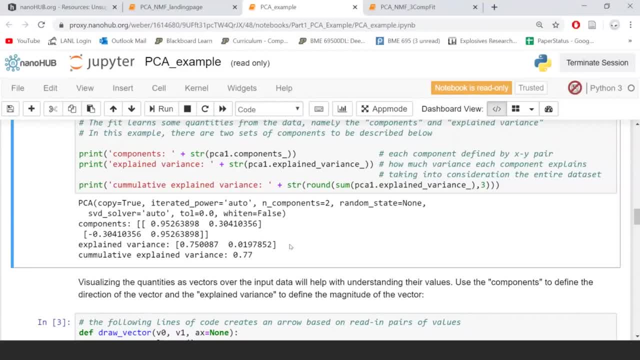 the actual states of your system are a much lower dimensionality manifold in that very big space. For example, important sampling techniques to do integrals. that's their need. It's because if you do brute force exploration of your space, most of the time you're going to explore areas. 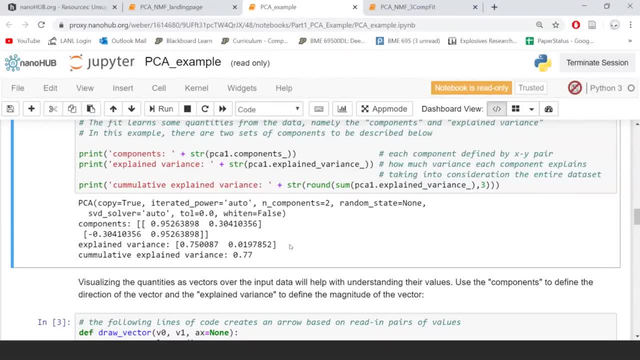 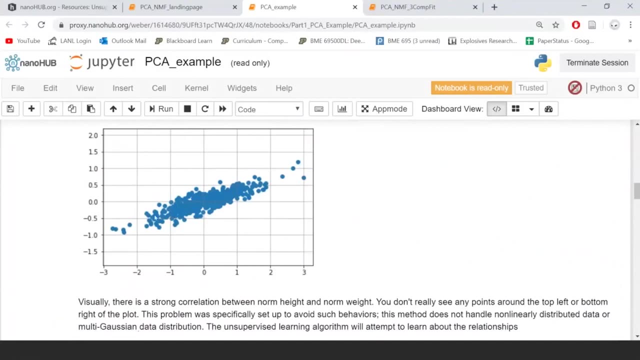 that are completely irrelevant. You can kind of see that in this 2D example that Michael showed, where if I throw points randomly there in that square, a lot of those points would lie in the blank spaces, where that's completely irrelevant for my problem. 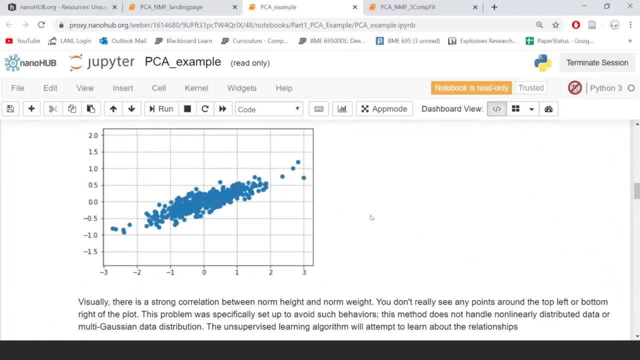 In 2D. that's not a big deal, But you can very quickly see that if this happens in higher dimensions, you're completely wasting your time doing brute force exploration of space. That's the reason for things like metropolis, Markov chain, metropolis type algorithms is to do important sampling. 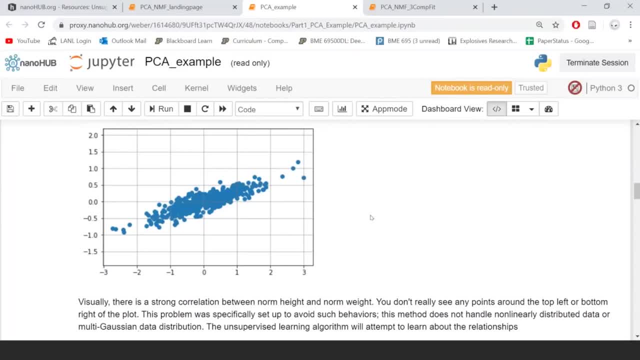 They're all based on the fact that in engineering and science, we always deal with a very lower dimensional manifold that we care about. Identifying that manifold is key to be able to start even thinking about solving the problem. Here's a question from the chat. 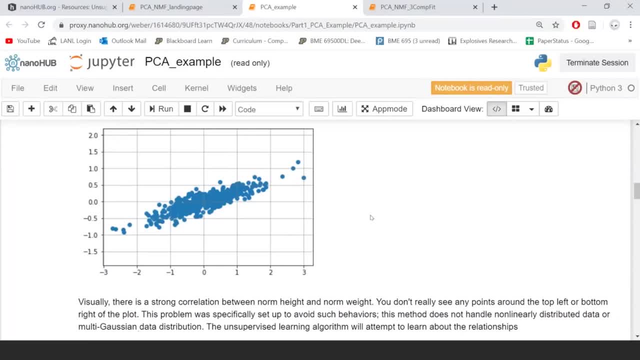 Does the non-negative matrix vectorization capture non-linearities or non-linear correlations? I do not believe so I'm sure it's very similar. The algorithmic approach is very similar to PCA, but it just has that constraint of non-negativity. 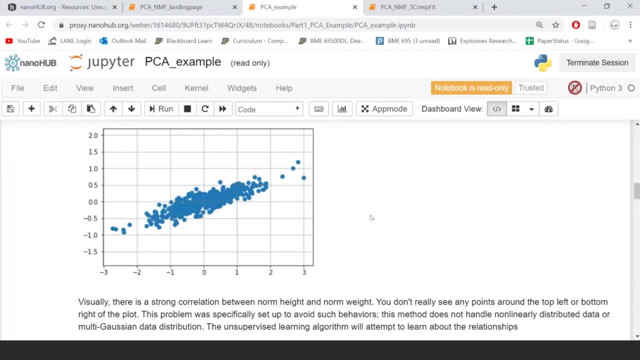 So, as like PCA, it doesn't handle non-linear behaviors, just like if you, as Professor Strachan was saying, if you have data that exists here and data that exists here, or if you can imagine that this data space was more circular, it's not. 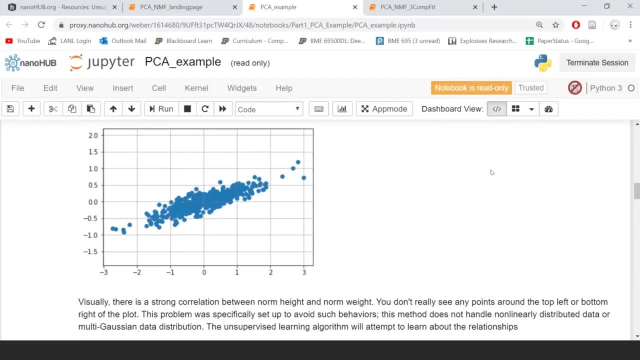 going to handle it very well. I know there are, I'm aware of approaches that can actually handle such behaviors, These being kernel- PCA is another one, so kernel underscore PCA. I urge you, if you're interested in these, this sort. 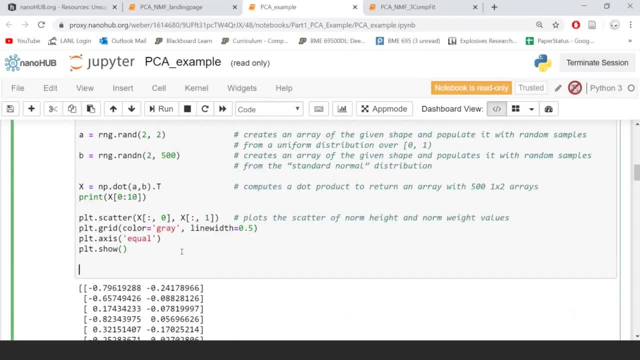 this is just a flavor of PCA and MF, but if you're more interested in taking this further, I urge you to go to the scikit-learndecomposition- something like that- And it'll go through a variety of examples of how to do the decomposition techniques. 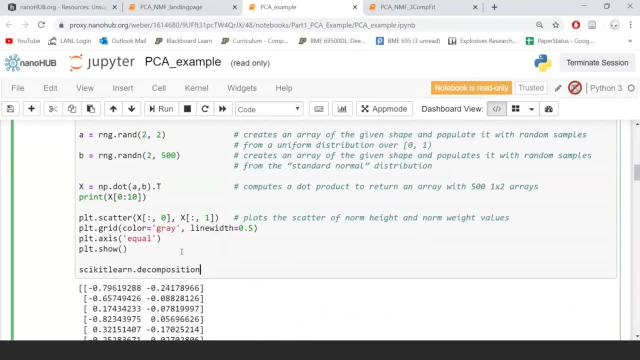 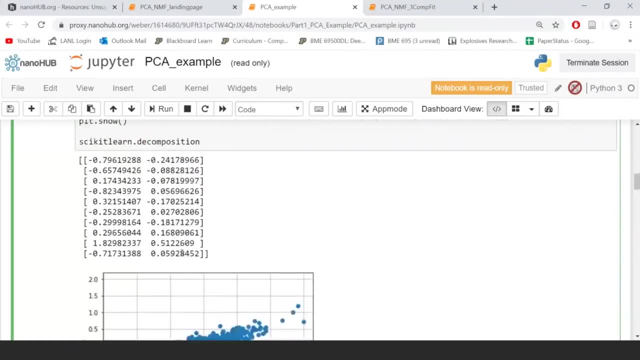 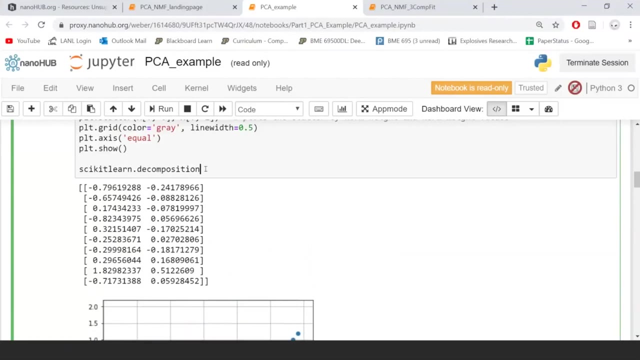 to handle more non-linear manifolds, non-linear behavior. Kernel PCA is one of them that I'm aware of at this moment, but there are a lot more listed there and it's a lot more detailed list. They have a lot of examples you can go through and try. 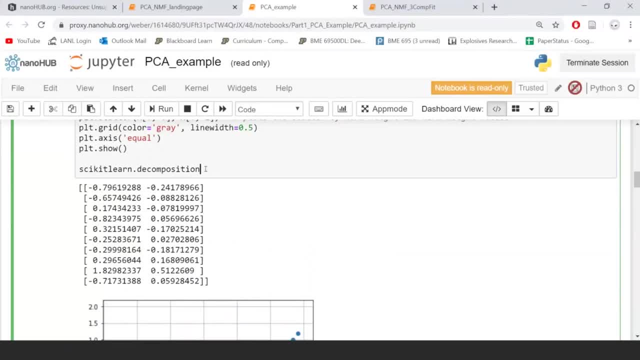 to read up on your own time, But for the interest of time I only wanted to focus on PCA and MF in this tutorial. Thank you. Another question from the chat. It says manifold learning algorithms can capture non-linear data. Are you familiar with manifold learning algorithms? 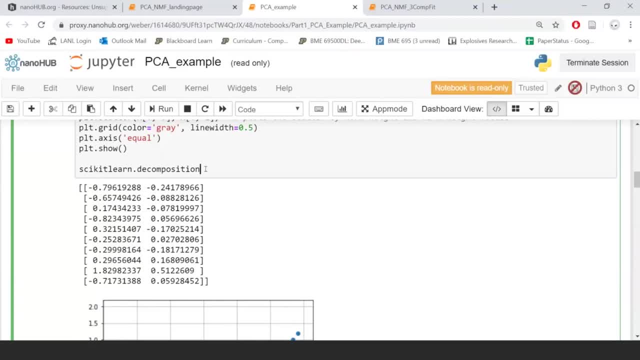 I mean, I think there was one of them that I explored, but I can't remember. off the top of my head I am aware that it does exist, But I think for the interest of the research we've stuck with linear data. 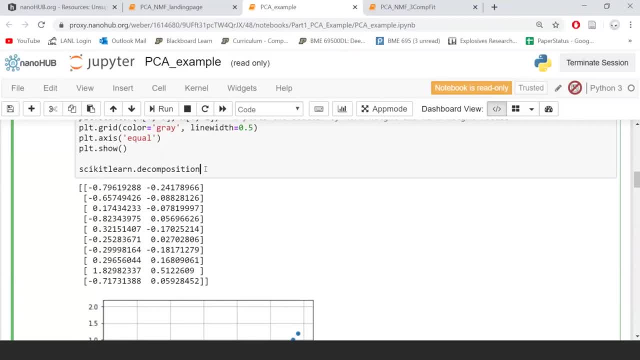 These are great. These are linear transformations. It's an eigenvalue, eigenvector problems we're essentially solving. But yes, I am aware of it, It just wasn't applied in this tutorial. I think the answer is yes And it'd be good to. maybe we can volunteer an expert. 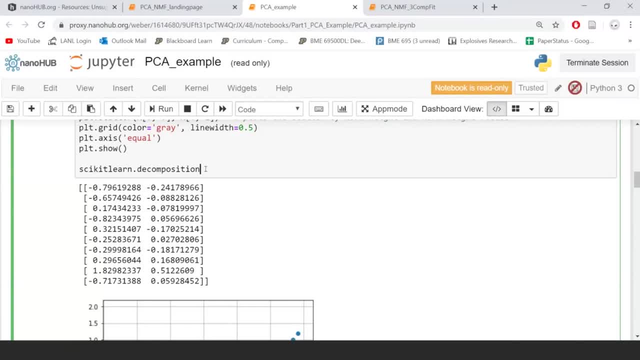 and give us a seminar, one of these hands-on tutorials on manifold learning algorithms. Thank you, Thank you, And I think that's the only way to get to the point of this course. if we can get more learning algorithms that can go beyond PCA. 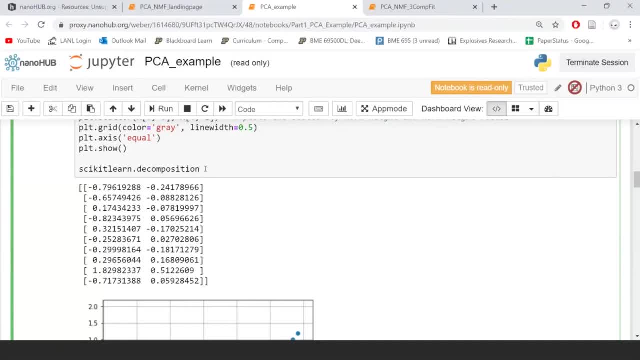 that would be an interesting topic. Yeah, Are there any other questions? I just want to interject with you. If you don't have any questions or they come up at a later time, you're more than welcome to email me And I will try to address it and get back to you. 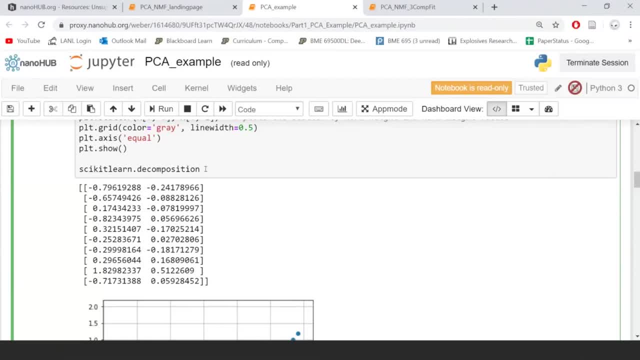 as soon as possible. if you're not, Or if you're interested in helping us with some of these sessions, if you have, as Professor Shotkin said, if you have expert knowledge in any of these areas, we'd more than welcome your ideas and maybe discuss with you how we can further provide interest into the community. 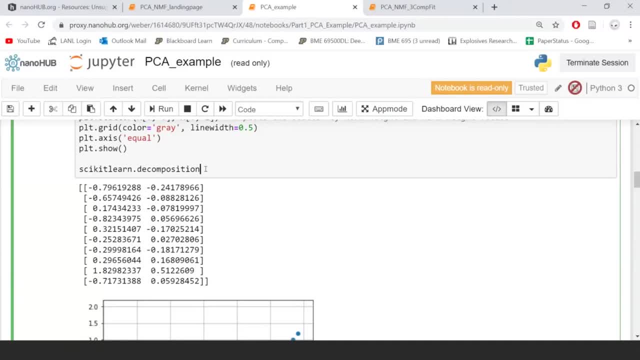 Yeah, if you want to volunteer to run one of these, or if you have topics that you would like us to cover, let us know. Okay, so if there are not any other questions, please unmute your mics and join me in thanking Michael for this session. Thanks everyone for coming.